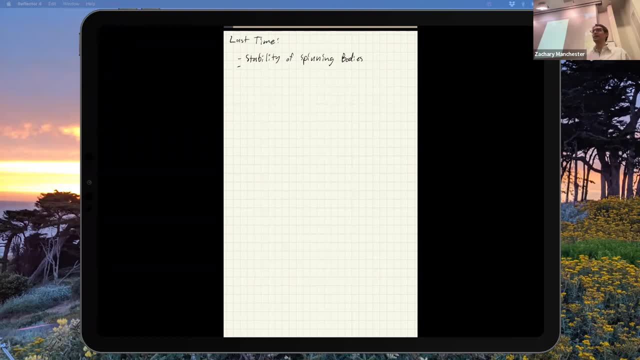 decades of the some Russian cosmonaut guy's name that I'm going to butcher if I try to pronounce it like Zybakov or something like effect, which is it's the tennis racket flip effect, right, And yes, some cosmonaut did it on Mir and made a video and then, like they named it after. 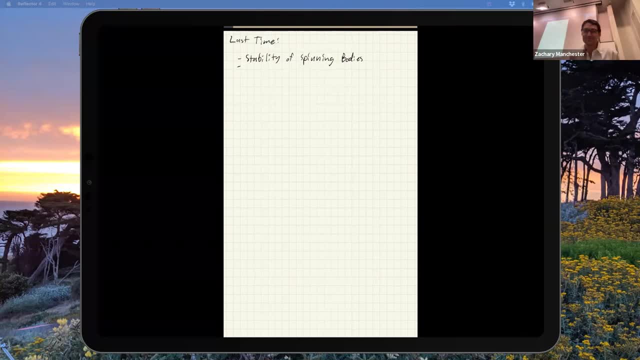 him, even though it was known for like 300 years before that or whatever Fun fact. And then we did like the numerical stuff, right, And this, yeah, so this we talked about kind of like 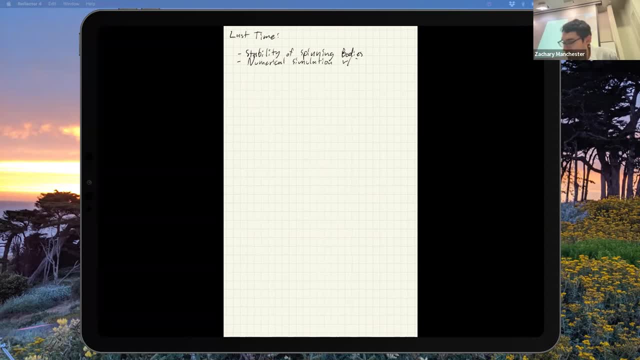 the things you should do. So, like if you're using a stock integration scheme, like if you're trying to use an ODE solver toolbox, like differentialequationsjl, like on the homework, the move is to probably just use the Baumgardt stabilization trick, If you can write your own. 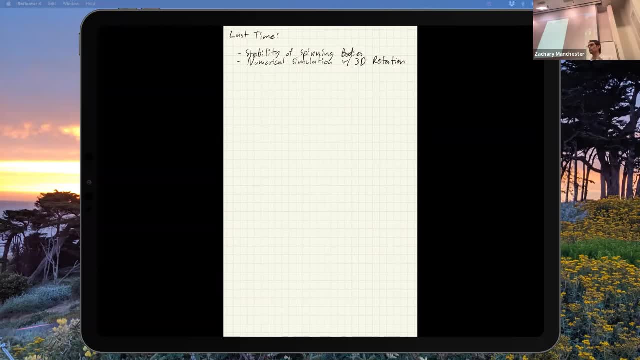 integrator, then the RKMK stuff is kind of the move and it's kind of the better way to go. The hacky-hacky classic move is to just renormalize your quaternions In your RK4 step. But yeah, all of those are kind of- you know, passable, It turns out the 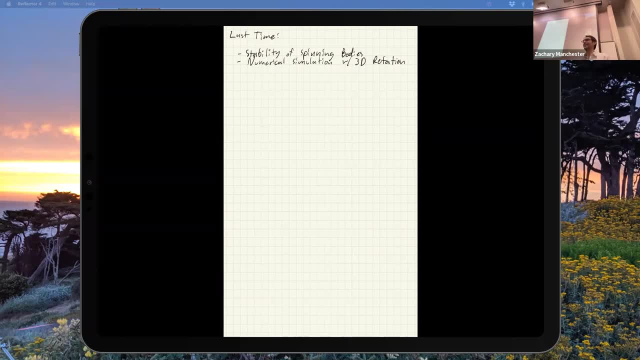 normalizing the quaternion thing in your RK step is not actually that terrible And it roughly. it almost looks the same as for the same reason as, like this Baumgardt stabilization thing only acts orthogonal to the true dynamics. It's sort of the same idea, Like it doesn't actually mess. 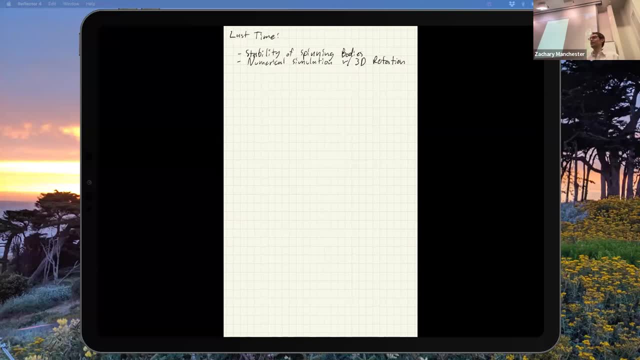 up the dynamics and it's kind of okay And you can like prove some things that basically you can show that it doesn't ruin the order of the Runge. So if you do RK4, and you just renormalize the quaternion, it turns out you still get a fourth. 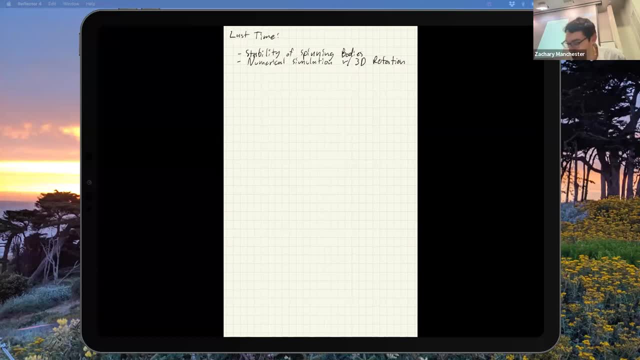 order accurate, like RK step and it's sort of okay. So I don't know. Fun fact, It seems sketchy. It's kind of sketchy, but it's okay And that's pretty much what everyone does. 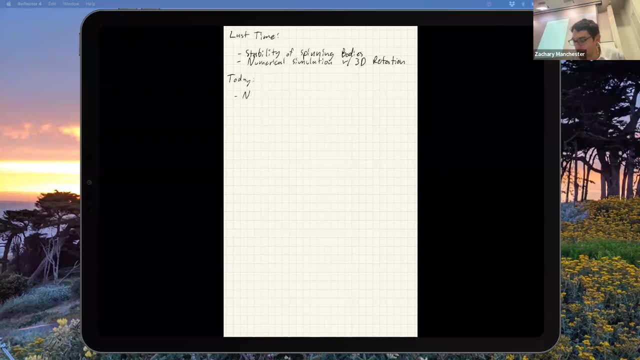 Okay, So today we're going to talk about Newton-Euler dynamics, aka SE3.. And so all the robotics people probably know about this. So this is the special Euclidean group, which is SO3 plus R3, right Like it's rotation, and 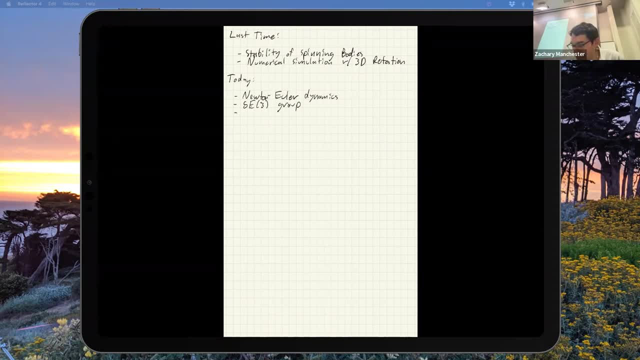 translation in R3.. And then we're going to talk about sort of practical stuff, So like quad rotors and airplanes which are, say, like kind of the maybe the canonical, like SE3 systems and robotics that we see all the time, And there's a lot of fun stuff in there. So okay, So who's? 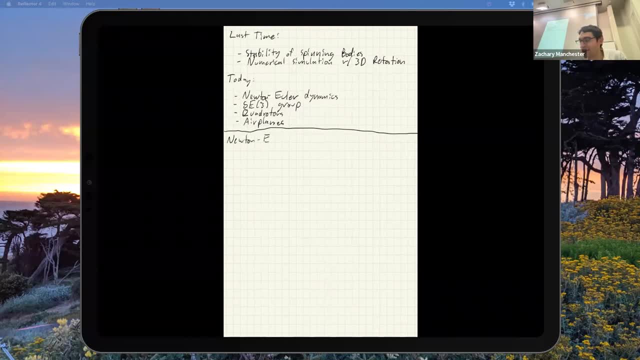 I feel like probably everyone has done this before. Show of hands: No, Oh, wow, Okay, Cool, Maybe this will be useful. So this is again. yeah, like this is basically the full sort of like translation. 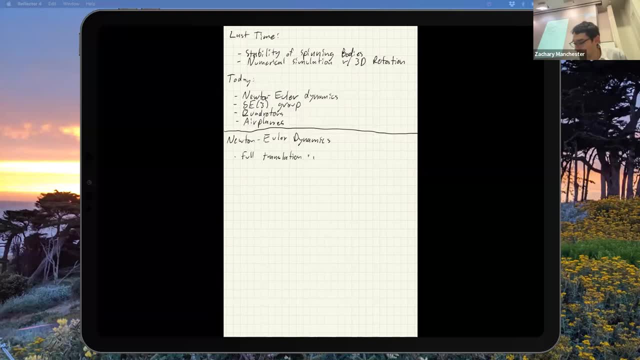 and rotation dynamics for a rigid body, And basically you just mash up F equals MA for the translation stuff and the Euler equation for the rotation stuff that we saw last week, And just kind of stack these things. There's some subtlety, though, which we will talk about, So you end up with something like this: 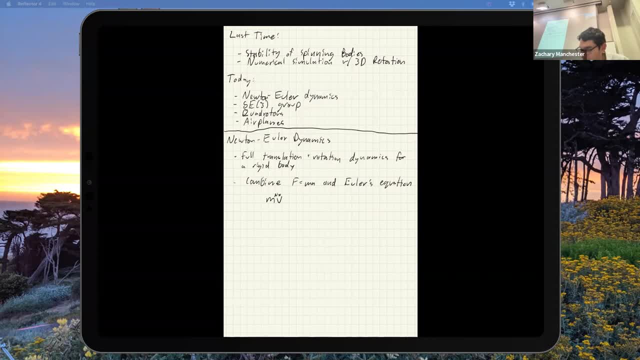 You get your like: MV dot in the end frame equals f in the n frame. and then you've got, you know, the euler equation which we're going to write in the body frame. so there's. this is where the subtlety comes in. there's actually multiple 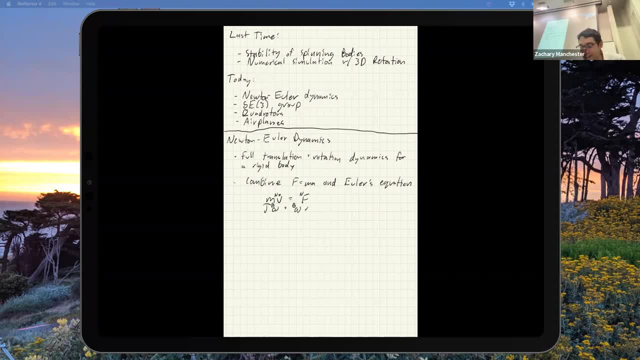 ways to write this stuff down. so i will show you the two sort of common options. so yeah, the most important thing to like note here is that f equals ma, always in an inertial frame. right, that's only valid in an inertial frame. euler's equation is only ever valid in a body fixed frame. so that's. 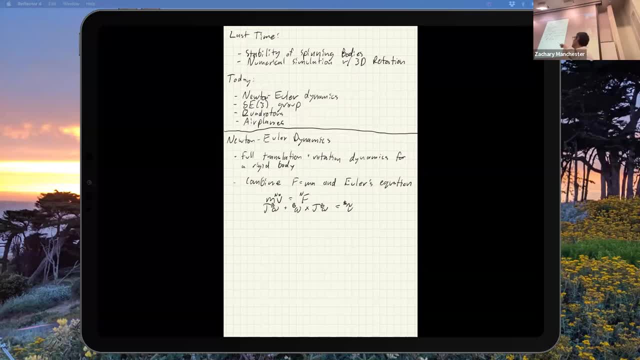 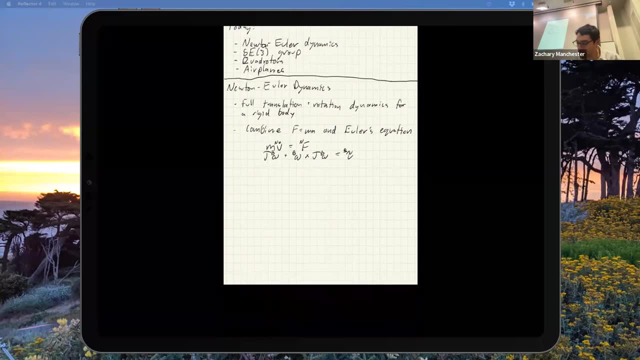 why i'm writing little decorations on here, right, so the forces are in the n frame, the torques are in the body frame, and this is kind of subtle and there's sort of some, some, some choices to make, right. so here's, you will see both of these and i guess i think i made this, hopefully, point in. 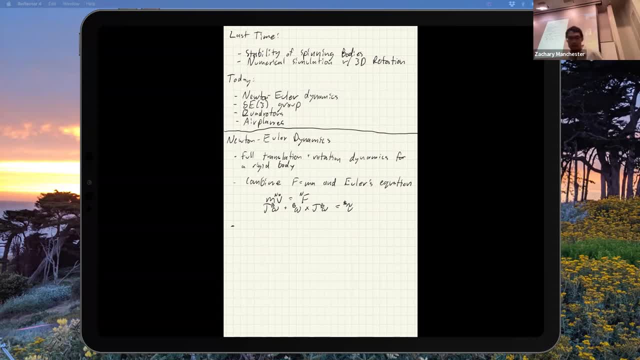 omega dot. yes, j omega dot dot. there's a dot on this guy. thank you, um. so if i- i hopefully made this point in- like the rotation stuff, like there's a million different sort of conventions for writing down rotations, you can write down, you know, the attitude as body to inertial or inertial to body and you. 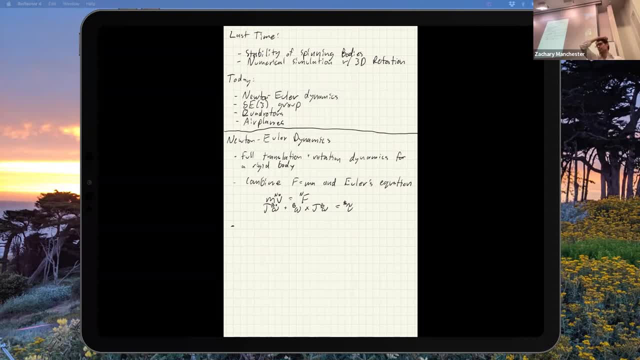 could stack the quaternion up in different ways and all this stuff right. generally the convention in aerospace and robotics is body to inertial, but that gets violated all the time. you'll see books where they do it the other way. generally the convention in physics is inertial to body. 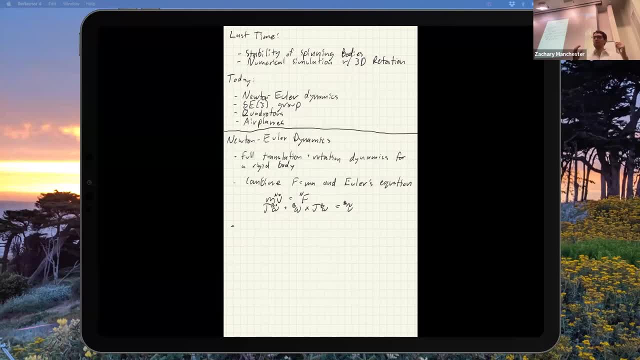 it's the other way, um, and i think this is sort of like this idea of you know, if you're a robot, you're sort of like living in the robot frame and you have all your sensors on the robot, so everything's body frame right by by default, whereas in physics you're like in the lab frame looking down at. 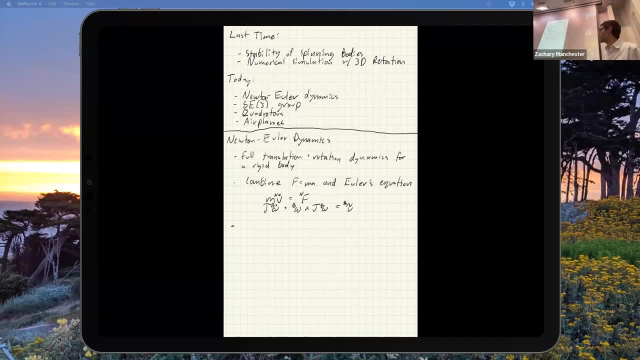 the experiment. so all your sensors are in the lab frame, right? so they kind of do it the other way. it doesn't really matter, but you will see stupid, terrible things all over the place, like. one of the things that is absolutely mind-blowing is that most of the books that do this. 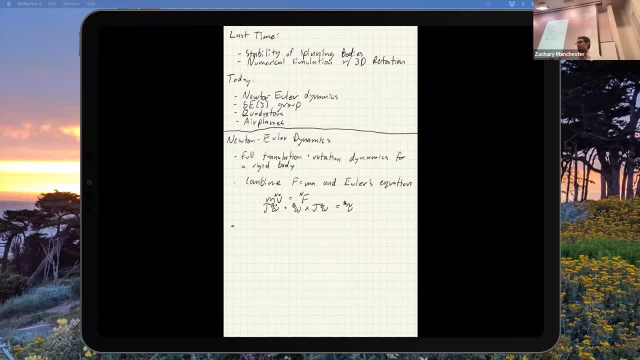 you'll find that they write the quaternion one way and the rota rotation matrix the other way. So we'll have, like all the rotation matrices will be body to inertial and then randomly they'll write the quaternions inertial to body And then all the like. 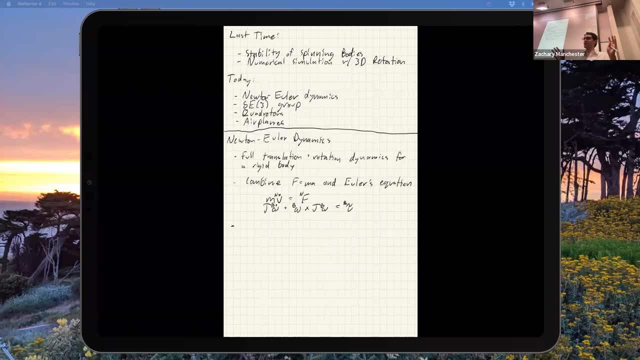 transformations between rotation matrix and quaternion will be all screwed up and like everything is terrible. So basically never, ever, ever trust like equations for this stuff that you get out of a book or a paper. like never trust them because there's literally at least half a. 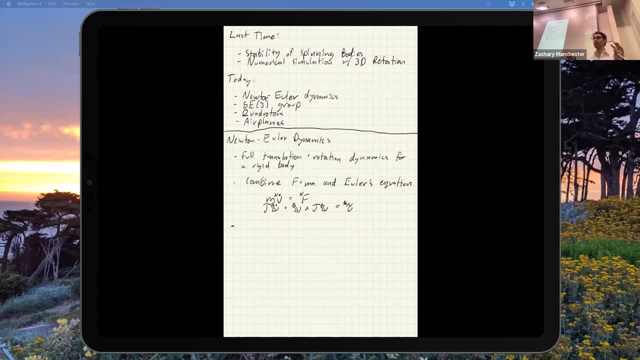 dozen conventions that are possible and people mix and match them for no good reason And it's absolutely just infuriating. So the message is: if you ever read a paper or a book that has anything involving rotations, quaternions, et cetera- SE3 dynamics- you pretty much need to. 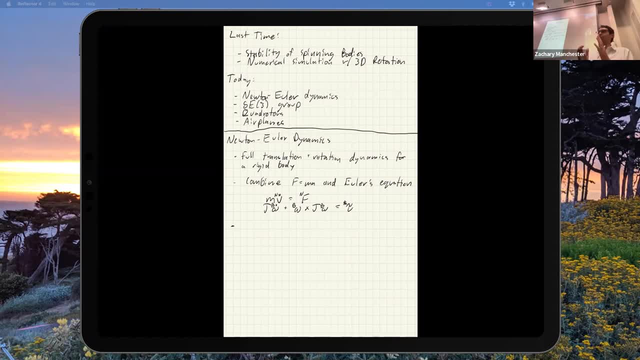 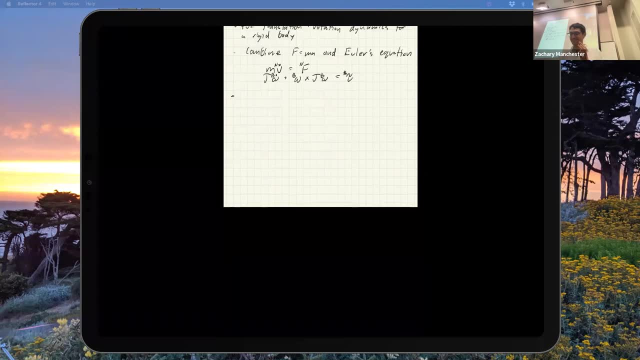 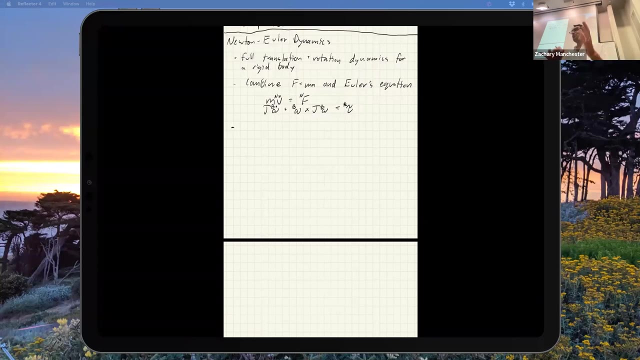 sit there and like re-derive the rotation kinematics yourself and like figure out what frames they're in, because they people do just absolutely unbelievably dumb things with this stuff like all the time. It is kind of awful, So welcome to like. you know, this is like when you 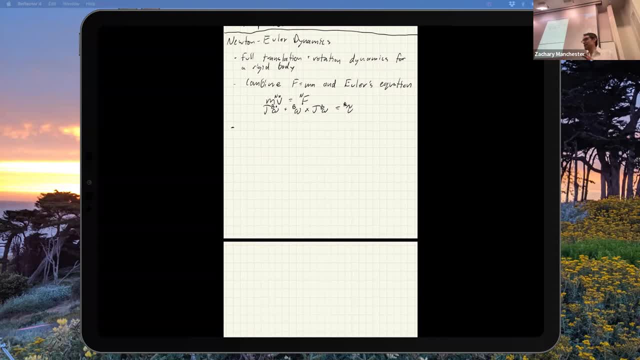 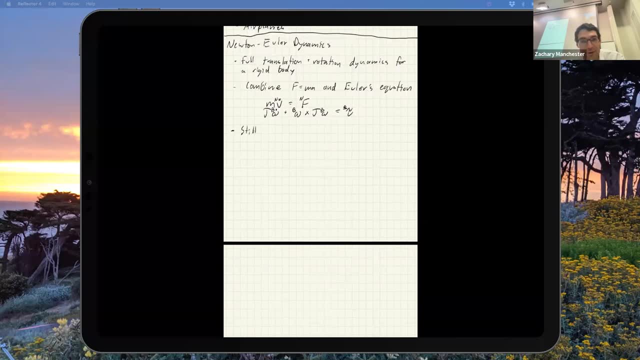 graduate from like undergrad math And like no one knows what they're doing anymore and there aren't any standards or like conventions that people reliably follow, So you basically have to do it yourself every time. Okay, So end of rant. There are some options here, to put it mildly. So the two most common sort of things you'll 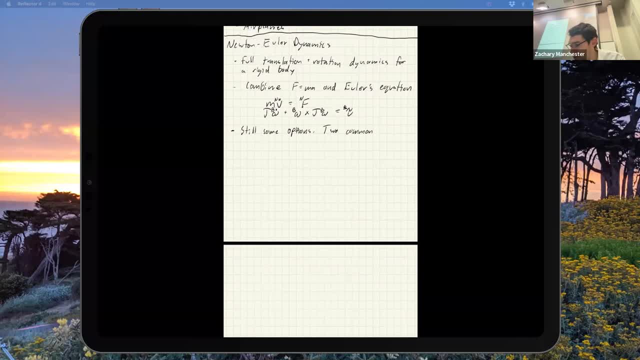 see. again, you have to kind of be really careful because they won't tell you explicitly. You'll see the state vector sort of stacked up. Either you'll see the state vector stacked up or you'll see the state vector stacked up Either. 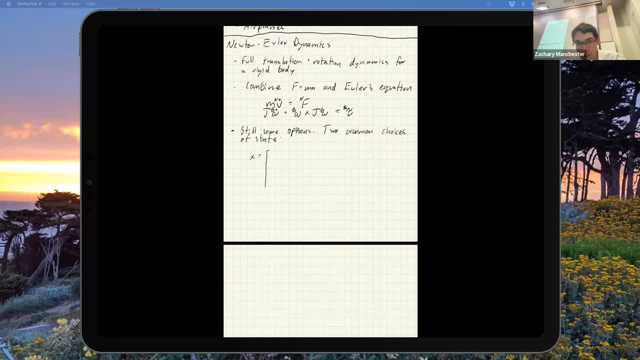 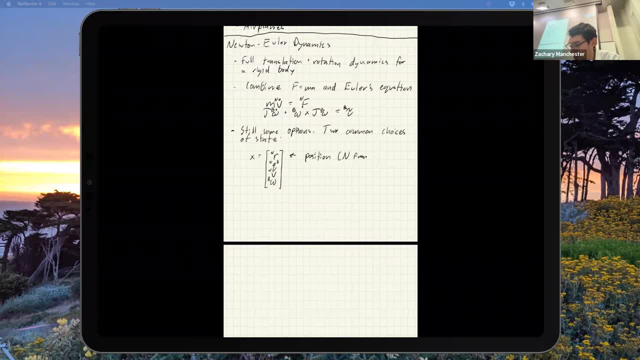 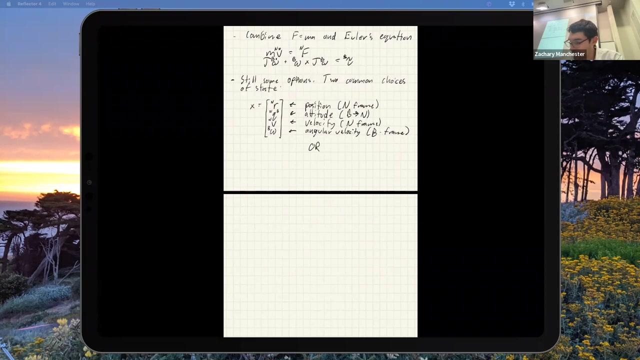 Position and frame. attitude B to N: velocity, linear velocity, obviously right, and frame And then angular velocity in the B frame. OK, so that's one option. The other common option is: let's see, let's do this. so mostly the same, except you write: 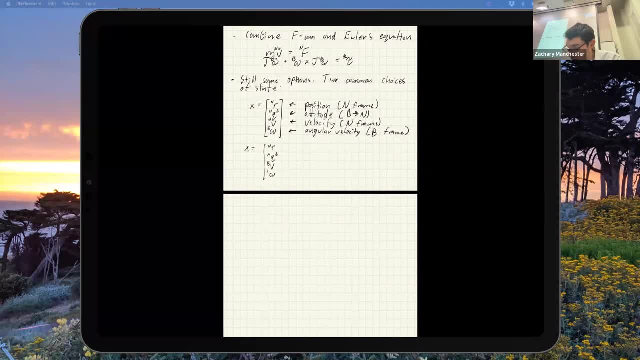 the velocity in the B frame as well. So you write all the velocities in the B frame, which seems a little weird, And what this is going to do now is you're now writing effectively. writing F equals MA in a rotating frame. 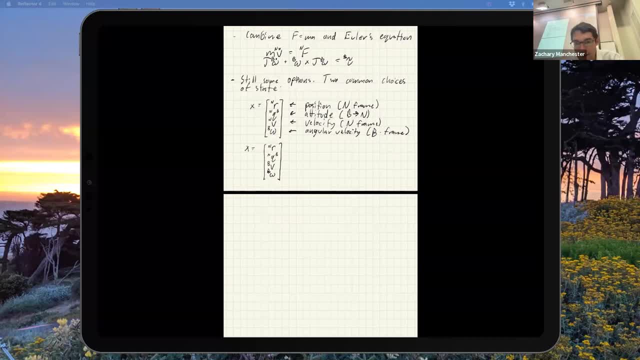 So you're going to pick up an extra term in there and we'll kind of so this is all the same, except now this guy is in the B frame, So why would you ever do this? It seems more complicated and annoying to write the velocity in the rotating frame. 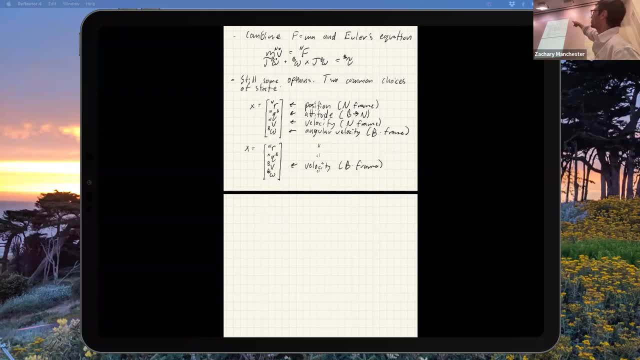 You get a new term. you get a new weird Coriolis term in F equals MA and you get a new term. So why would you ever do weird kinematics to integrate VB into RN? right to account for the rotating frame. 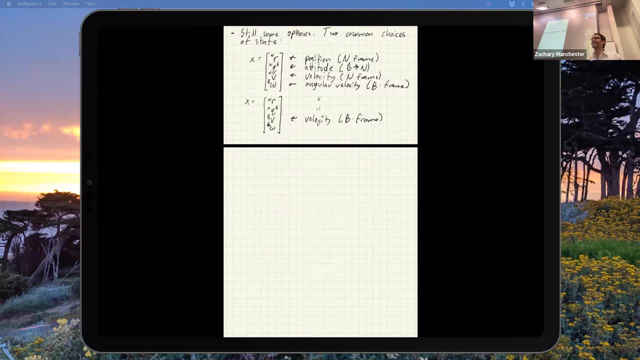 So why Does anyone have any clue why you would want to do this, Aren't they what? Yeah, so that's basically where this is coming from. So it turns out the first one does not obey like a consistent group transfer. 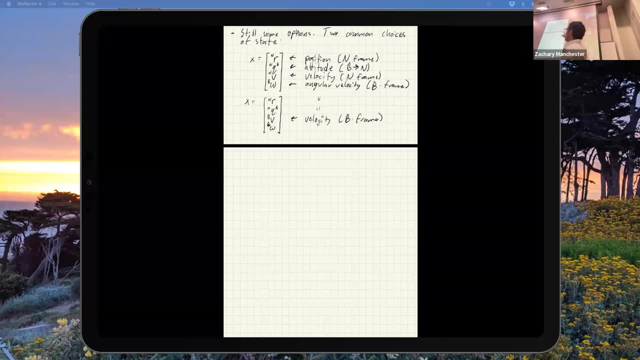 The second one does So. the second one is actually SE3.. The first one's not And that's sort of practically useless, I have to say, But there's a bunch of fancy math that you can do with the second one that people are. 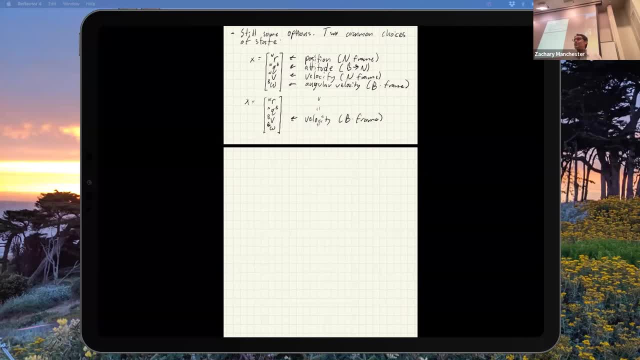 enamored with Some of it's kind of cool but honestly, practically speaking, I would say it makes almost no difference. There are fun control laws you can write down with the SE3 stuff and you can do all this nice thing. 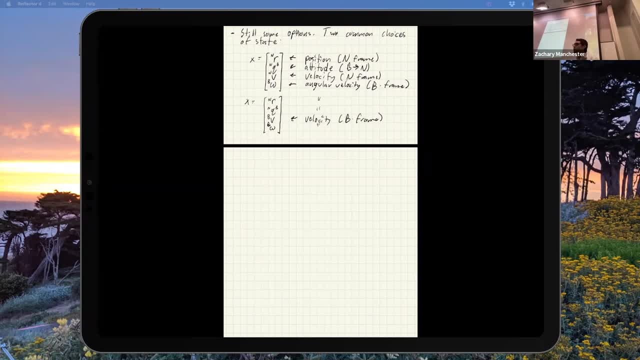 You know, SE3 transformation matrices with that. The one thing that seems maybe vaguely useful about it is: it turns out there's in the last like 5, 10 years there's been these French guys who've come out with a whole theory of. 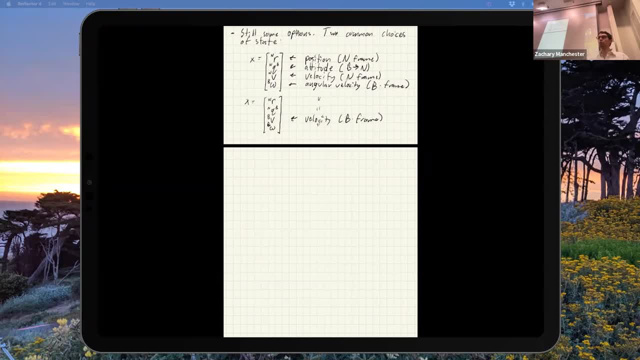 Kalman filtering on Lie groups. That's really nice actually And you can prove for nonlinear systems, ie extended Kalman filters, where you're doing a bunch of linearizing, it turns out if you write the Kalman filter down in the 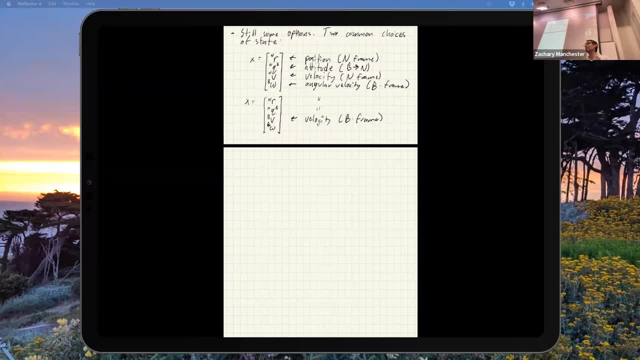 Lie algebra like this for a Lieger system. you can prove Convergence like Aspen, product convergence, exponential convergence of the nonlinear estimator of the Kalman filter by using a bunch of these group theory tricks. So that's the one thing. that's kind of cool. 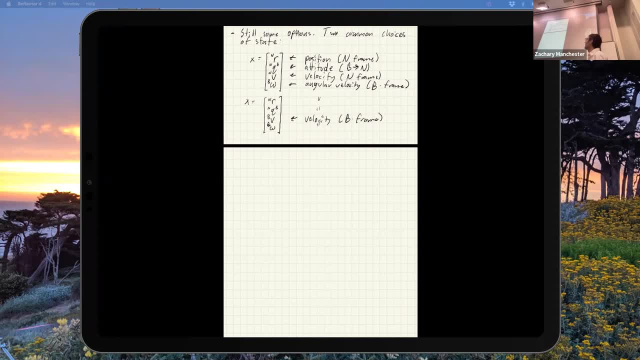 Practically speaking, I think the performance of those things is like not much different from like just doing the first one. But the theory is very nice and you can prove nice like global convergence results for these things, So kind of cool. 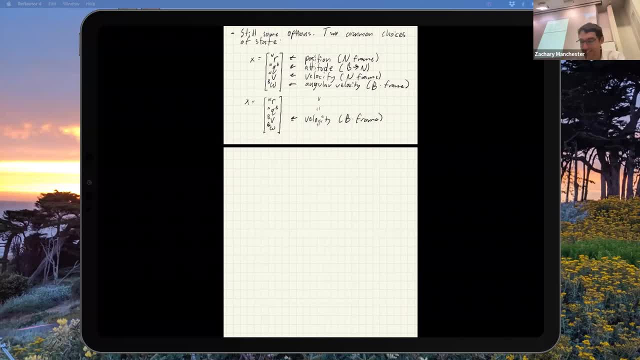 Unclear if they're practically any better, though, But like, the math is nice, So that Okay. So let's say So. for simulation it really doesn't matter at all, I would say, But for control and estimation theory it doesn't. 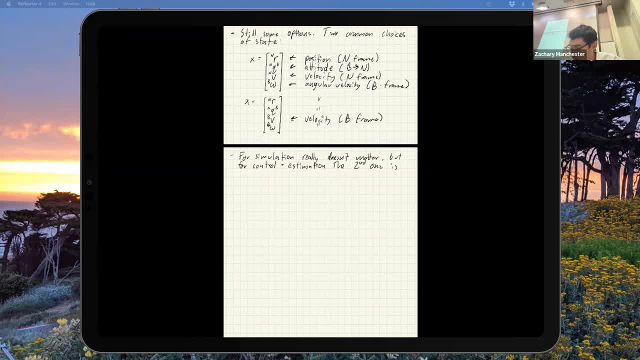 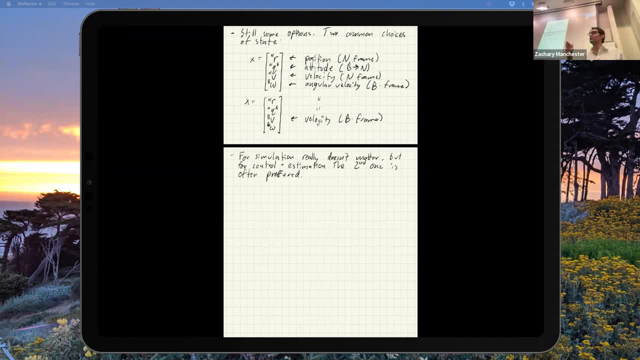 It actually is cool. So what ends up happening? It turns out, if you write the like ekf equations down in the Lie algebra, it turns out that they, the, the matrices associated with the ekf, are invariant, ie they are not time varying. 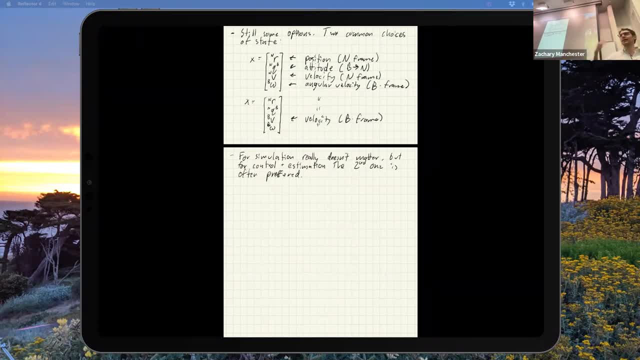 anymore Like So a standard ekf right, You have to relinearize. It turns out if you magically do it in the Lie algebra like this and use the exponential tricks, it's invariant now, Like the a's and b's don't change because they're constant in that. 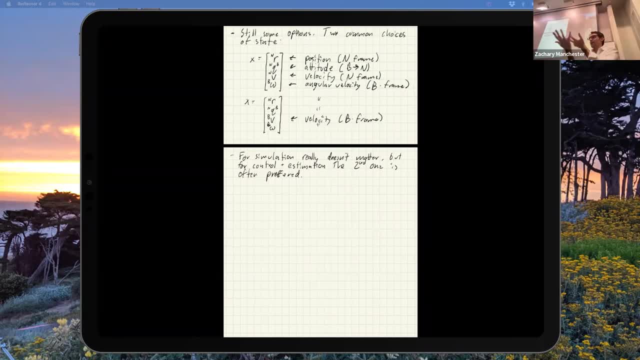 What you're basically doing, right, If you think about it, the dynamics are sort of moving around on this sphere, right? Remember the quaternion kinematics. The invariant trick is you do it on the Lie algebra, which is always the tangent plane. 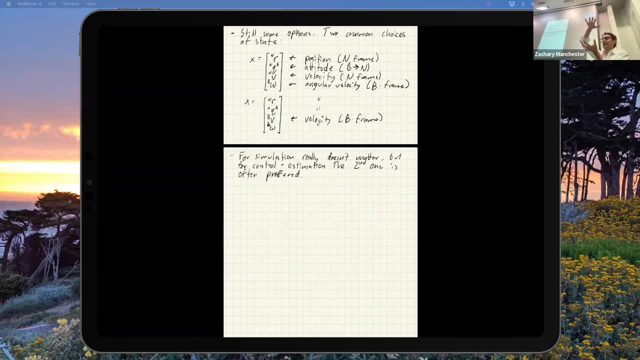 at the North Pole. So the North Pole tangent plane is constant, Doesn't change. And you use the kinematics trick to like: move the, move the tangent plane around Outside of the filter. So now the filter equations are always at the North Pole tangent plane, and so they. 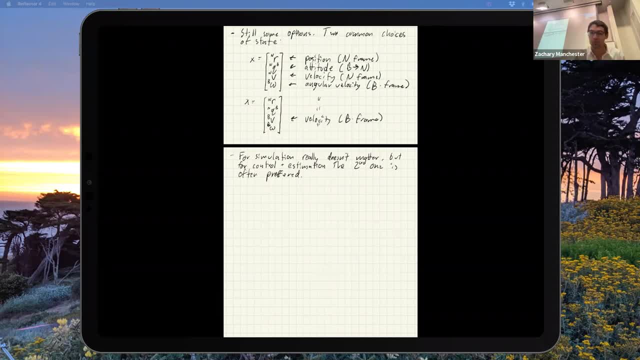 stay constant. They're invariant, which is pretty slick actually. right, That's kind of cool, Okay, So any question about that. So a justification for using like body frame vectors that I've seen is like aerodynamics are in the body frame and like your IMU or your accelerometer measurements or body frame. 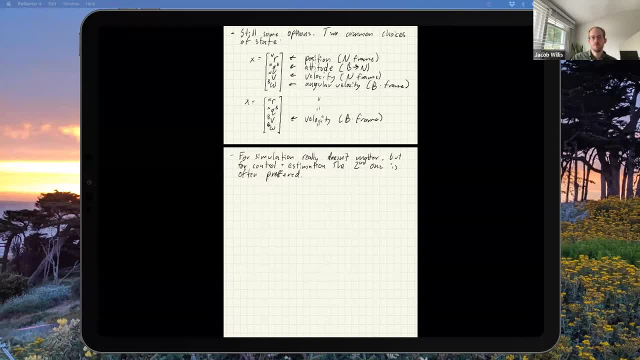 And and. Yeah, so I would say, that's that. So those things are all unequivocally true. Practically speaking, you're going to end up rotating stuff back and forth either way. Go out and we'll do this in a minute. 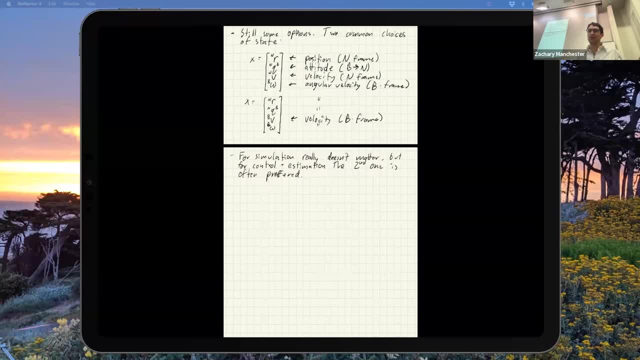 Like you're going to So like, but gravity is always in the inertial frame right. So you always have a mix and match situation where some things are inertial and some things are body and you're rotating stuff. I don't think it makes a big difference when you're simulating, but there are nice things. 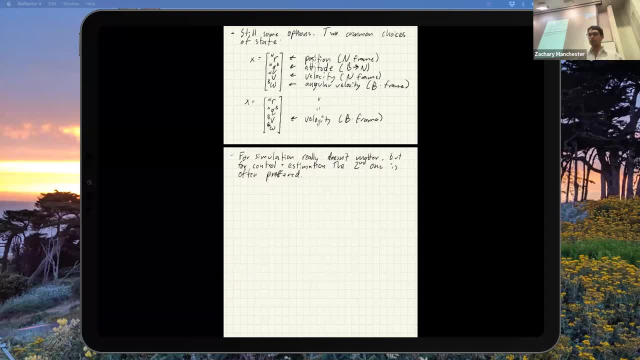 you can prove. Yeah, Yeah, Theoretically about the S3 stuff like the invariant column filters- probably the biggest example, Turns out. controllers also generally work better with the second one. empirically, like it is, it is nicer for certain things like writing down my key id. and the second one. 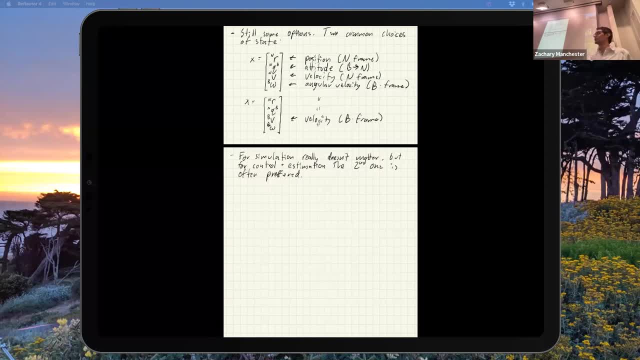 works better turns out in the first one, Because in some sense it's the same argument like that: that North Pole tangent plane, sort of like, doesn't move around as much, So it's like nicer to write things there because the things don't change as much. 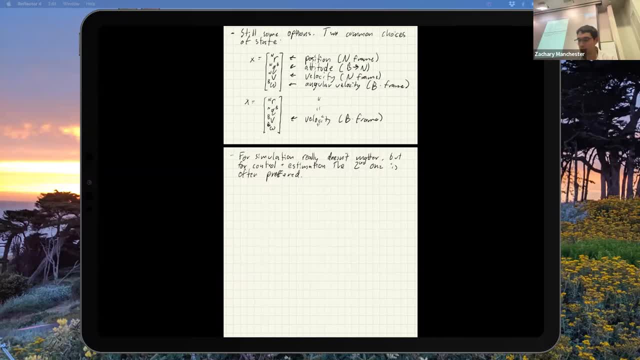 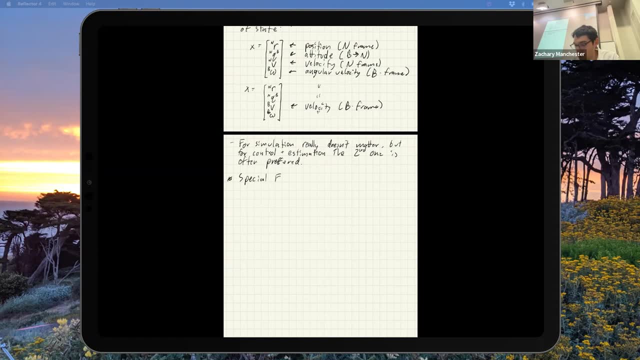 um, so like when your control works better there, okay, cool. so here's, here's sort of the the key thing. so we're going to talk now about what's called the special euclidean group, everybody. so this is se3 and it's, uh, the group of all rigid body transformations and, as we said like kind of last time, um, all the. 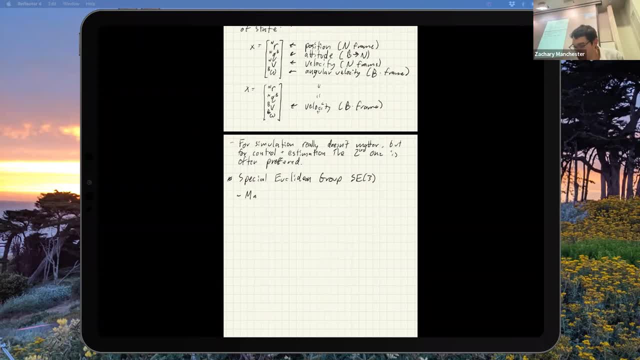 useful groups are matrix groups. you can always write it down as a matrix, so here's what that looks like. so these are commonly written as big t for a transformation, i guess, and so you'd imagine like this is kind of this body to inertial thing if you write the little decorations and the sort 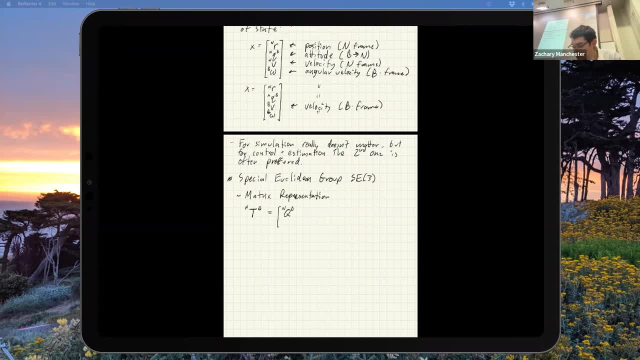 of this big chunk up here is the rotation matrix and then, um, then you have this over here the translation vector, and then kind of just pad the matrix out, like so, so we've got center of mass translation and then this guy's the unusual rotation, um, and so, if i can write, let's draw the cartoony picture, i guess. um, 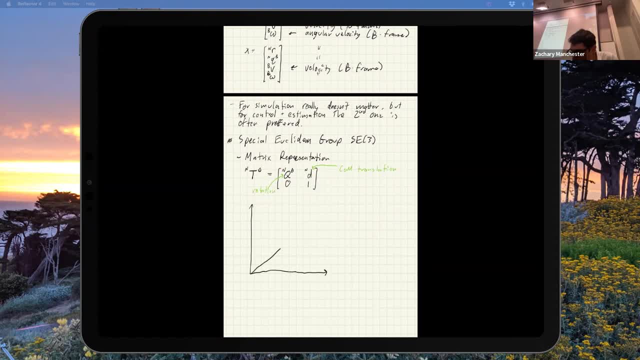 so if i have some like world frame here, so like n1 and two and three um, and i've got my rigid body over here and this guy has a center of mass um, so i've got like my body frame, you know, attached to this guy, say, 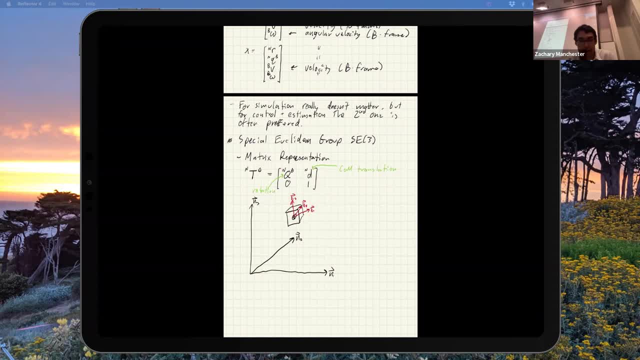 and i've got this. um yeah, let's see what else was i trying to say here? all right, so i've got some- let's take some- vector fixed in the body frame, right? so this might be a sensor measurement, right, that you're making, like might be your gyro measurement. 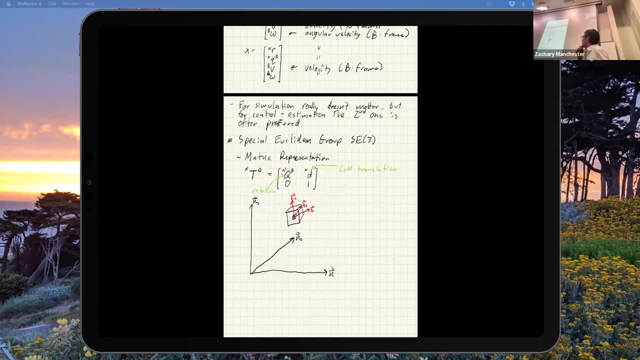 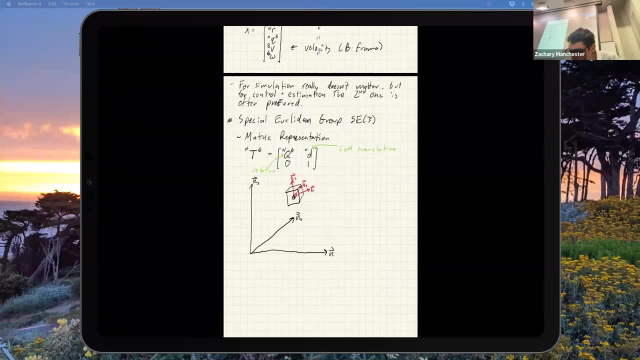 whatever, uh, or it could be like: maybe a more, a better one would be like some camera, you know, um, some vector to a feature from a camera right in a camera frame or that kind of thing. so you've got this guy over here, so we'll call this r. 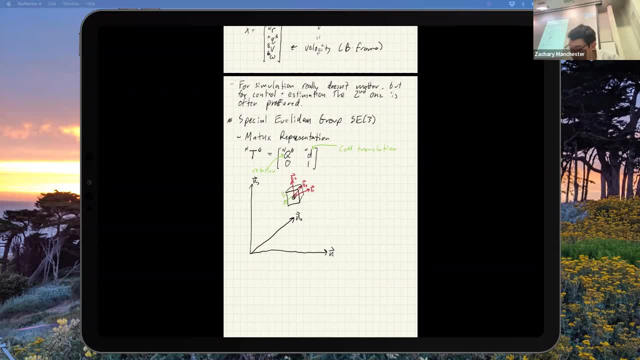 b, and then what we want to get from this thing is rn, which is the same vector. that's pointing to the same feature, right, but it's rooted in the world frame and written on the other coordinate frame, so that this is what this transformation matrix does. so we got this guy. 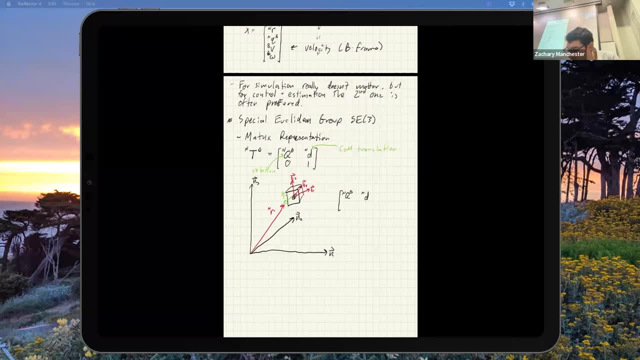 uh, here's the translation thing, and we're going to multiply it by in the following way: so we take that rb, we pad it with a one- that's just how you do it to make the algebra work out- and you'll get out qr plus d and a one on the. 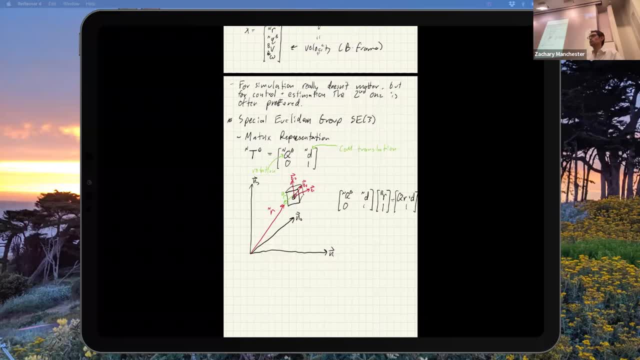 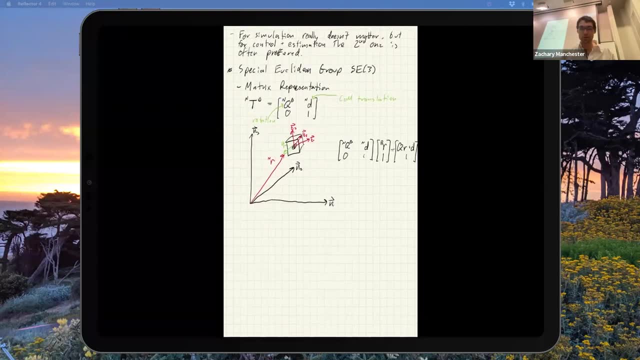 bottom right so it rotates and then translates makes sense. and who's seen this before? what's you guys? this is like kdc stuff, right, like. this is a little bit, maybe kind of. yeah, okay, so that's sort of the the mechanics of doing it now. what we're gonna so now we're gonna do, is look at. 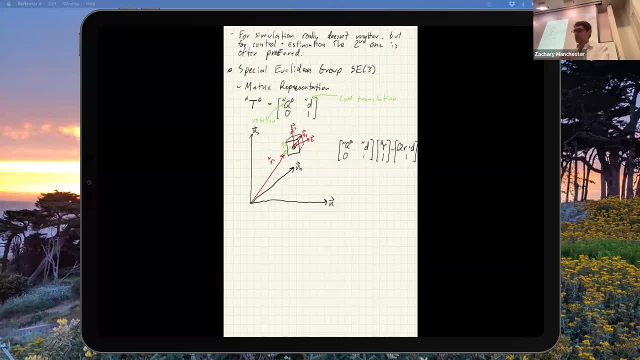 the sort of like kinematics and velocity for this guy right, and this should sort of make clear that that whole state vector thing we just talked about before. okay, so we're gonna kind of do the the following thing. so we're gonna take a little sort of 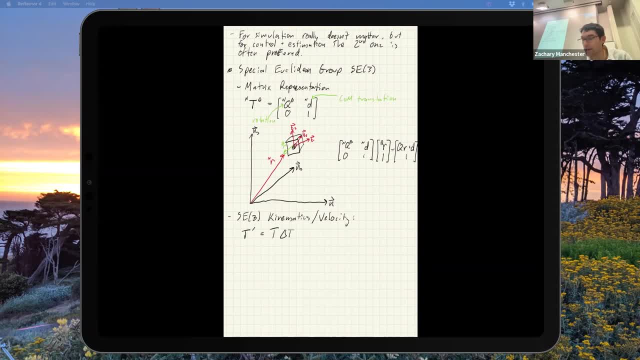 perturbation of one of these guys. so we got t times, some delta t, right, so a small but finite transformation and we're going to write down the kind of taylor expansiony stuff. so we got this guy, we got this guy. this is sort of the nominal t. 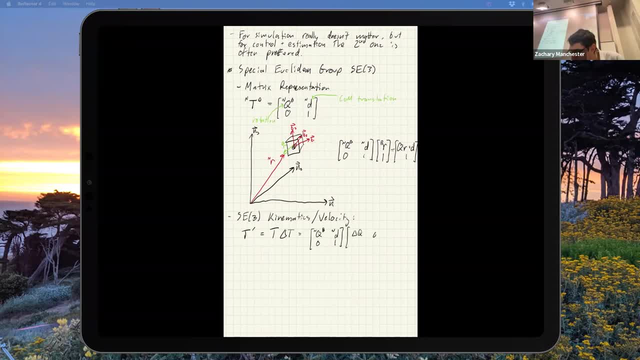 and now we're going to write down a small like a delta q and a delta d over here and we're going to multiply that out and sort of see what happens. so we're going to get obviously q times delta q and we're going to get um over here. 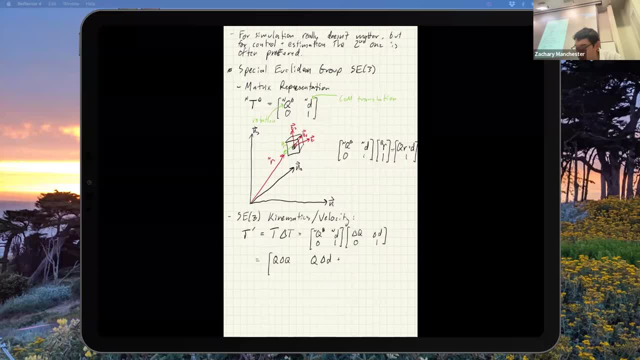 q times: delta d plus d plus the original d. okay, so this stuff over here is sort of obviously the same as what we had with s03. so the fancy way of saying this is that s03 is a subgroup of se3. right, it's all there, as usual, it's. 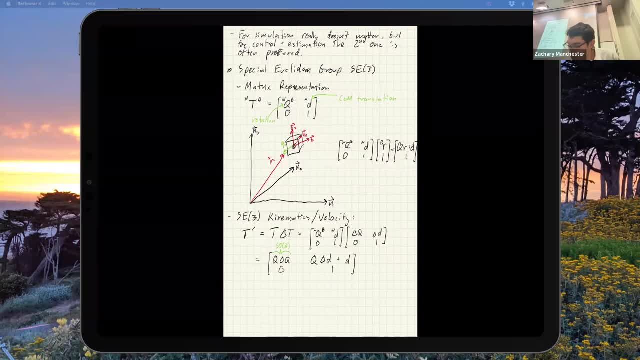 like this sub, sub chunk. okay, so now, from this flow, we want to look carefully at this. so what is this saying about delta d, specifically the subgroup of se3? right, so now what we're gonna do is we're gonna d specifically. maybe i should write little decorations on here. what frame is delta d in? 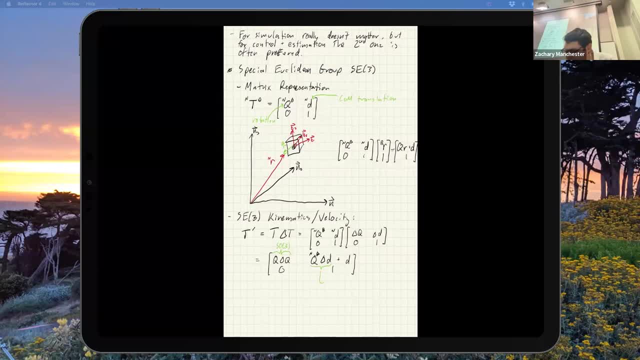 that's sort of the important takeaway from this. so this is, remember, this is n frame stuff, okay, so so this whole thing, this guy's in the end frame, so clearly to make things line up like this whole thing has to be the end frame. right, looking at this equation, like what frame is delta? 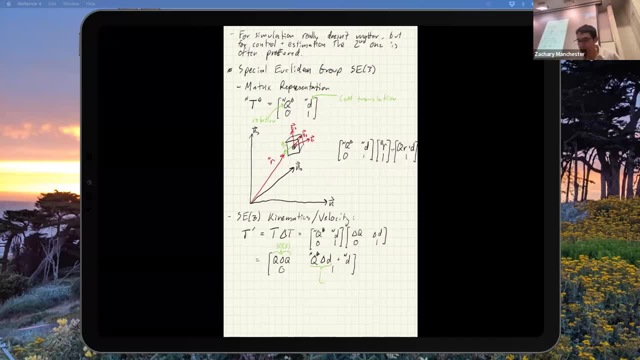 d in in the body frame, right, okay, so that's kind of the key insight. uh, is that when you're doing and you're chaining them together, so sort of what this tells you is like if i, if i apply some little tiny delta d, you know, to this guy, it ends up being the body frame when i chain it together. so therefore, 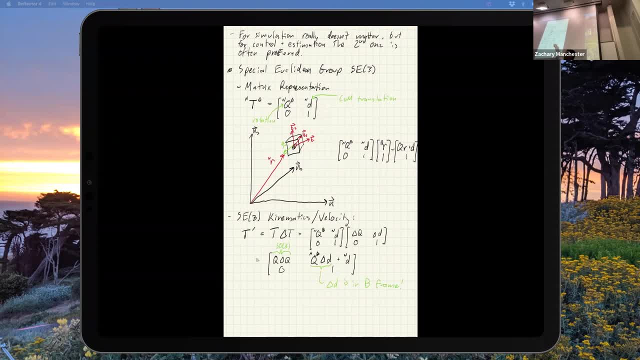 if i write down the velocity, ika, lee algebra here, just like with the rotation, so like this guy clearly is in body frame, right, that was like that's like our omega half thing on a deal, this guy, the translation he got, and in the limit if 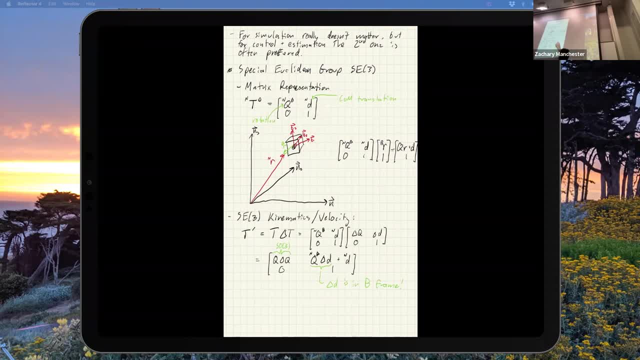 i take a limit here and make this a velocity. if i divide by a vt, basically it says that my velocities are going to be in the body frame, which makes sense because the omegas are in the body frame and it's sort of consistent, right. but that's sort of where that comes from. 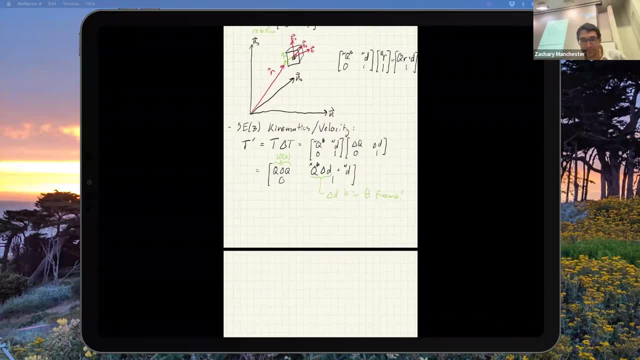 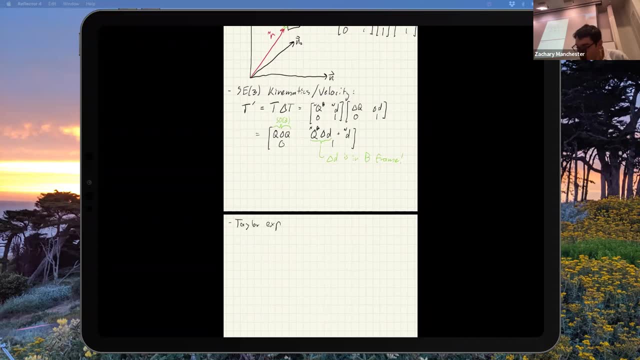 um, so i'll do that now all the way out, i guess. uh, so we get delta. q is the proxy or it equals right, like: this is the exponential that we saw before. so it's our omega hat times some time step and we can approximate this to first order. 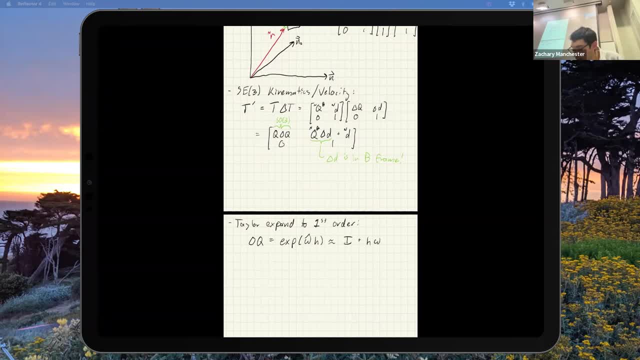 with the taylor expansion of the exponential. as, like h omega hat, it's first order in h, right, so we did that before. and then for delta d, we're just going to get it's approximately, you know. so this is in the body frame, right, so it's. 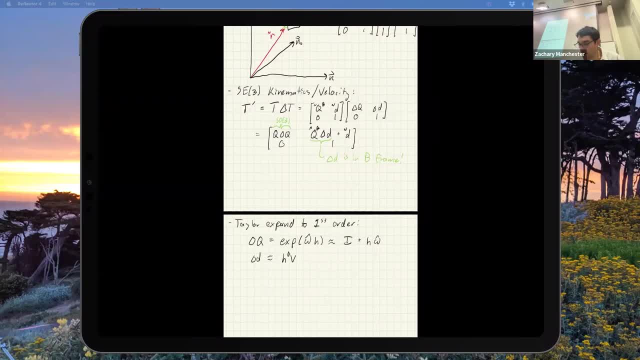 approximately just h times some velocity in the body frame right. this is basically assuming, like euler integration or you know, tiny tiny com step. so if i kind of write this out now, i'm going to get t prime is approximately so my original thing, qd times i plus. 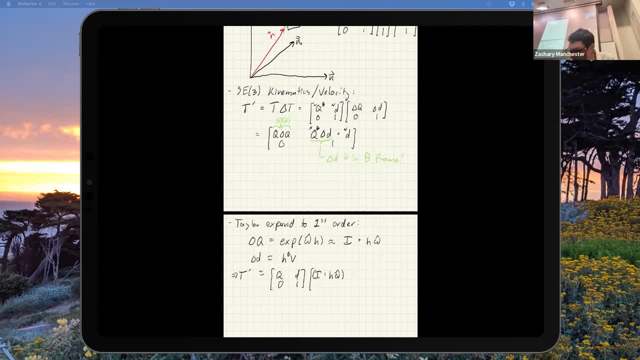 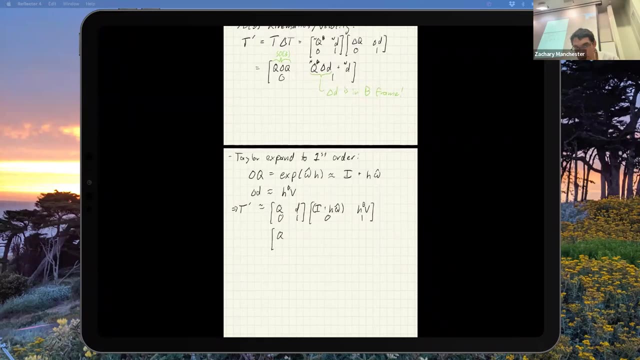 h omega hat for the small rotation, and then h times v in the b frame for the small translation. first order in h. and now i can kind of just pull this thing apart, and so if i so, if i multiply those together, i'm going to get q plus h, q omega hat. 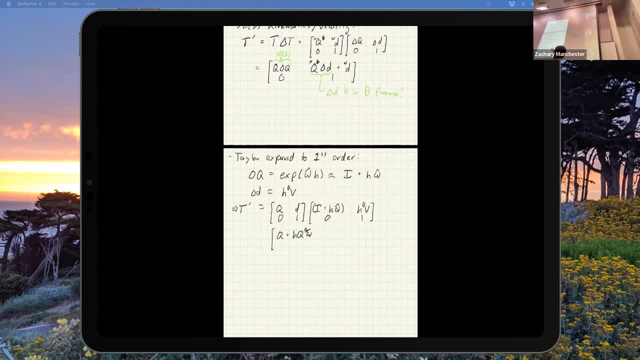 right, which looks just like this, looks familiar, right. so this is our rotation kinematics we had before and then over here I'm going to get hqv in the body frame plus d in the end frame: 0, 1,. blah, blah, blah. 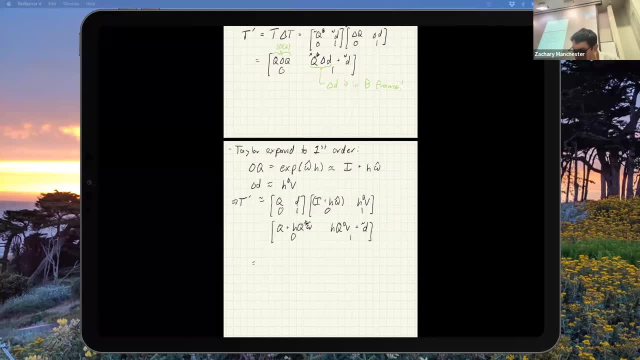 Cool. So that's multiplied together. Now I'm going to pull it apart and I'm going to get qd01, which is our original t, plus the first order in h stuff which looks like qv01 times omega. hat v in the body frame 0, 1.. I guess I'll write the frames on. 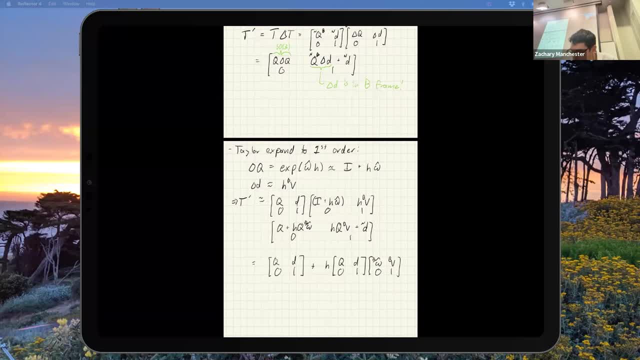 Okay, so what this looks like now is t, and then this is t, and then this guy is your like omega hat equivalent, right? So I got Okay, We'll write this as, I guess, w. Maybe we should write this as w hat, I don't know Yeah. 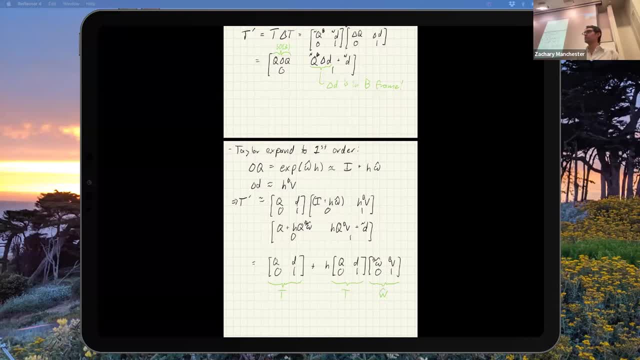 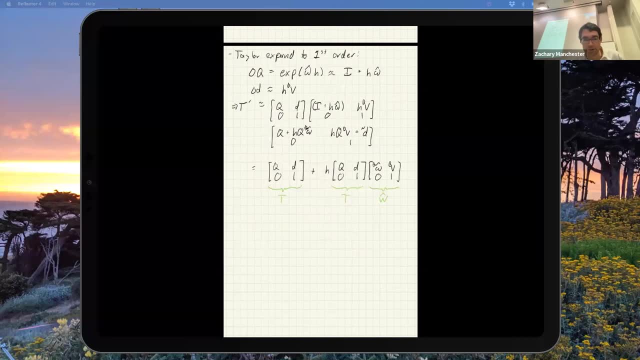 let's do w hat to be consistent with, like the omega hat notation. So what you're doing now right, is like: so this is So obviously. the kinematic equation is like this thing, that's first order in h, right, That's like sort of your. So if I take the 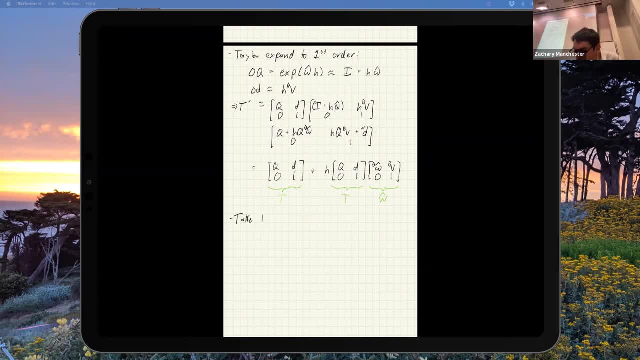 limit now as h goes to 0, and I, What I'm really doing here is basically like: this is like a delta, t, right. So I'm going to. I'm basically going to divide around, divide by h, right? So to make 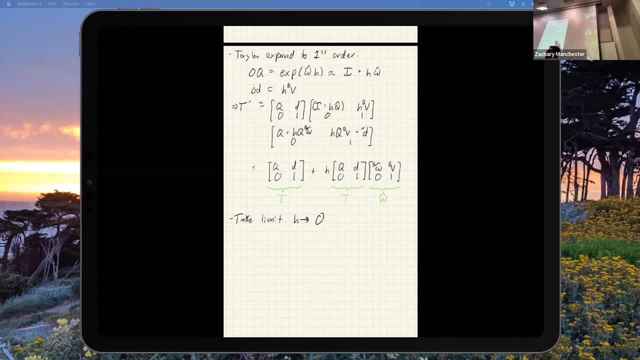 this perfectly clear, right? this is: t prime equals t plus stuff times h. I'm going to go: t prime minus t divided by h right, which is the limit for t. dot Everyone get that? So let me write that down explosively. 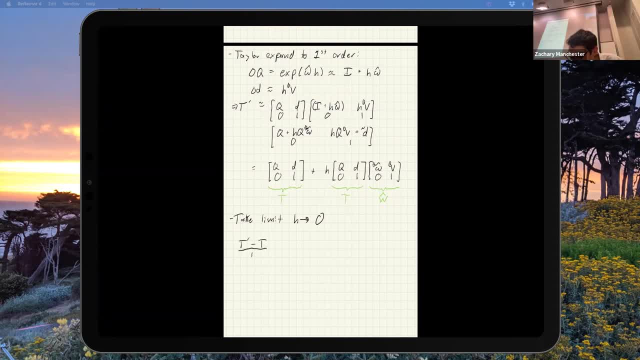 So t prime minus t over h is going to be t dot right, And that is the stuff that's left. So that's just t w hat And that's my kinematics now. right, So we'll call this guy Like. 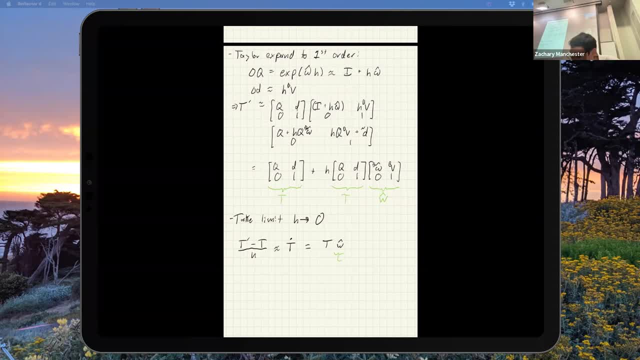 we have the hat map for s o 3. We're going to call this now the hat map for s e 3. And remember, big letters group, little letters, algebra right. So the li, And remember li, algebras are vector spaces. So this guy, I can stack up omega and v as a single six vector. 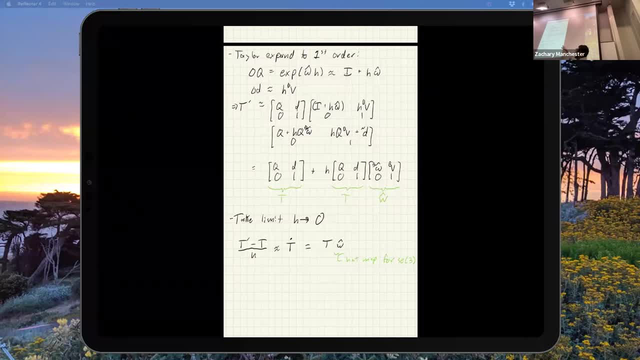 And that's what my like s e 3 guy is right. And then when I hat it, it means I stuff it into this matrix. How big is that matrix? Four by four, right? So this is three by three. This is a three. 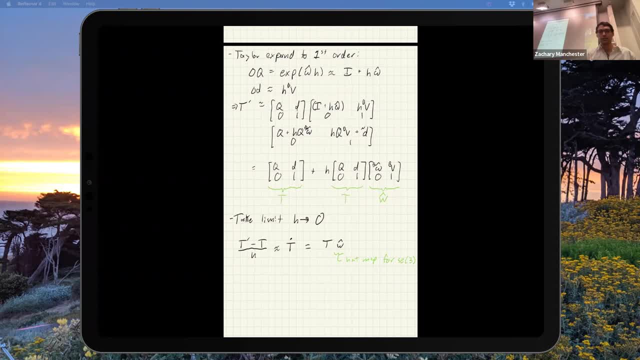 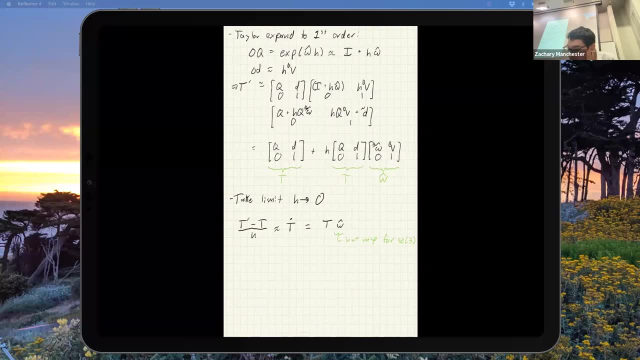 by one, And then I've had it like this to make the algebra work out: Okay, so let's write that, So w, w equals, And again, you can do this either way, Sort of arbitrary conventions which you always have to be careful about, which is why you kind of have to do this stuff yourself. 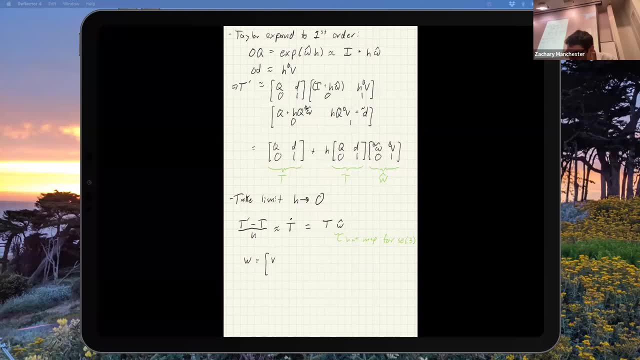 and can't trust books and papers anymore. v, b, we'll stack it like this: Um in R6 is the li algebra s e, 3. Um and then yeah, um, as a sort of sort of as with. 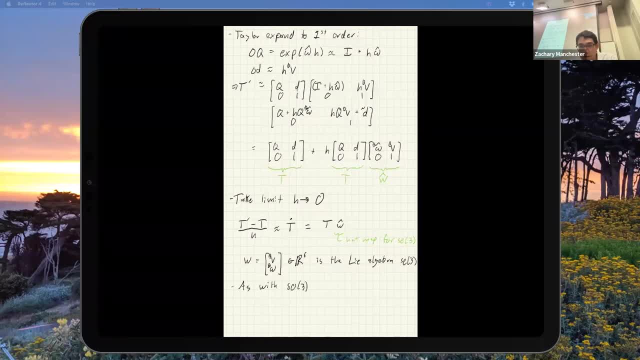 s o 3 or constant w um. we have as the So for constant w. this is a linear ODE right And so same deal as before. we can just exponentiate this guy. right to get uh. 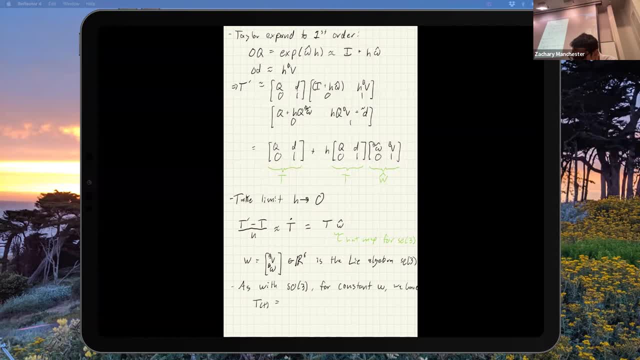 t of t equals t naught times the exponential of like um t w hat, right Exponential. Now I'm gonna go with that Again. linear systems, right. Think about it as e dot equals e omega hat, that kind of thing. 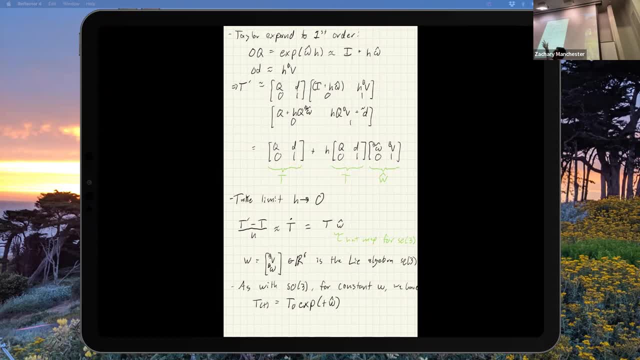 Oh, the other kind of note, right, Remember, for linear systems we usually have like a, e, phi right, And here it's b, a backwards. Why is that? I don't know. So what if I flip the order, Like what happens? 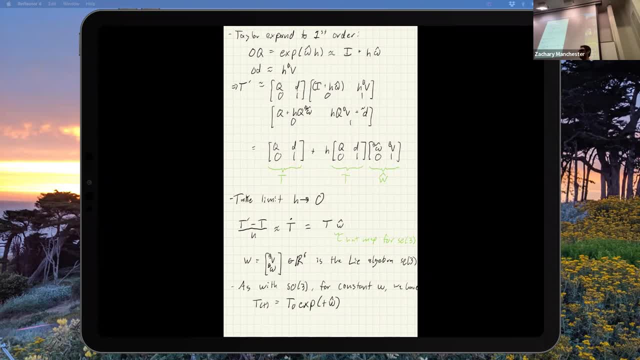 I get the wrong answer. It's just that they don't commute right. But like, does anyone have any thoughts on what's going on there? Like what happens if I flip the order? Like what's um what would be happening? 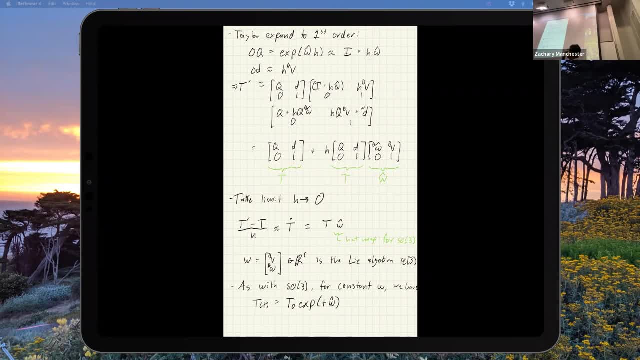 Yeah, Opposite direction, Yeah, So. so here's a way to think about this. This guy is in the body frame And this is body to inertial. What happens if I flip the order and I put the uh w hat on the other side? 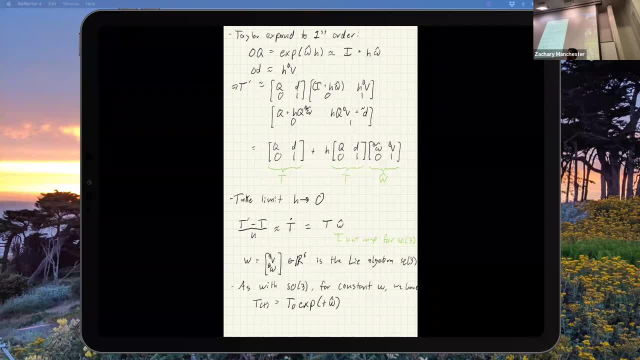 It means you're writing these velocities in the inertial frame, So you can do that. so, but what that mean corresponds to if you do this the other way, it corresponds to having all the velocities in the inertial frame. So if you were to write down omega in the inertial frame instead of the body frame, 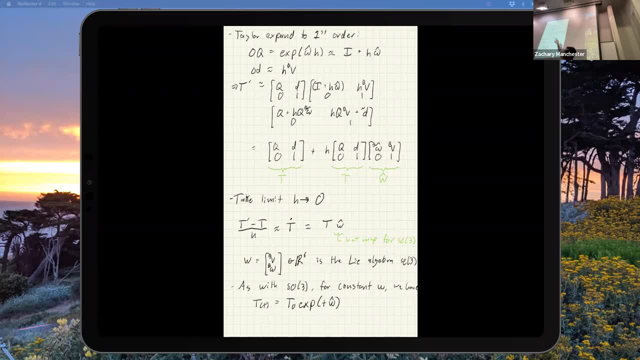 and in this case you know you would, you would end up with kinematics the other way, and that's that's why- and you will see that in bush- and that's what's going on in the linear systems case it's effectively like inertial frame velocities. um, it's sort of a difference that makes 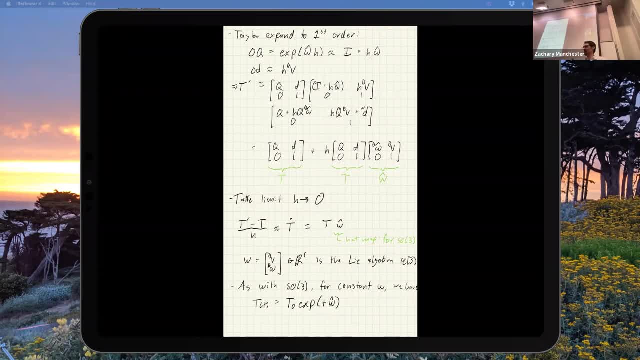 sense. this is why, again, you got to be super careful with this stuff. you'll see like multiple conventions, you'll see mix and match. so the one thing that is clear: it's still a group. if you write them both in the inertial frame, um, it just has everything flipped. basically, it's not a group. 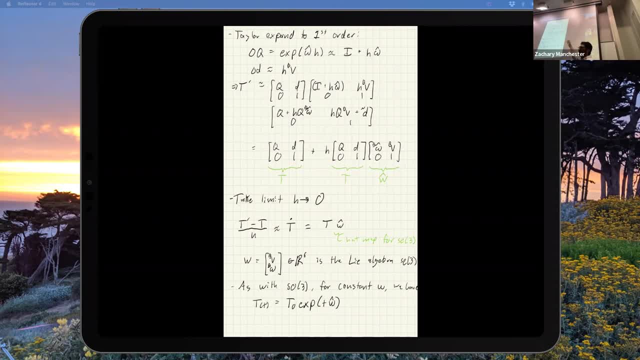 if you mix and match, so if you write like omega in the body frame and b in the end frame, it doesn't form a group. you can't end up writing it nicely as a single matrix transformation like this. it's sort of inconsistent, right. okay, any questions about this? the same kind of gymnastics we went. 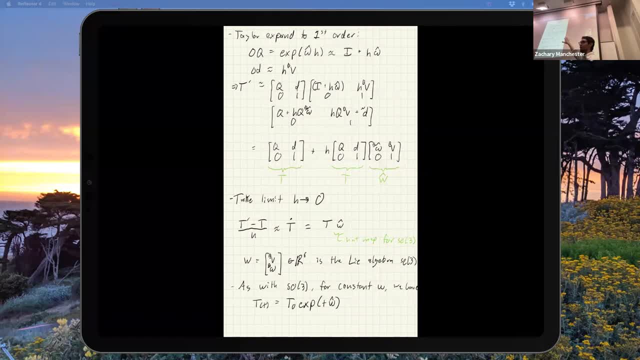 through for the just rotation case. but it turns out right. you can stuff the velocity in there and come up with the. as long as you write it in the body frame and everything is consistent, you can write this whole thing as a group too. it turns out like fun recent-ish research by last five. 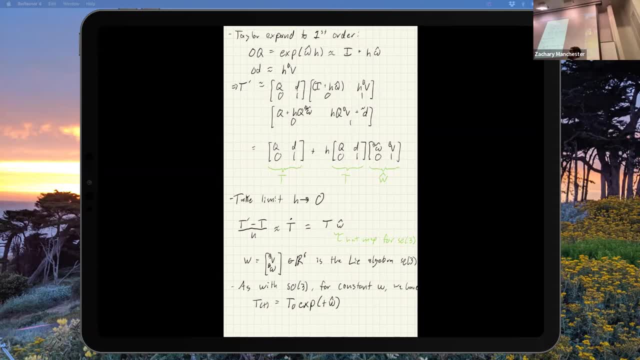 years stuff. i mentioned this invariant column filter stuff. it turns out you can stuff lots of other things into a matrix like this and keep going and make bigger and bigger groups, and some guys at michigan had a field day with this recently and like came out with a bunch of really really nice results for invariant filtering for 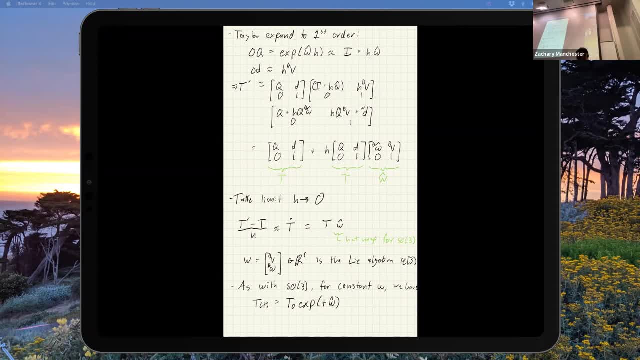 legged robots. so it turns out you can like write down the foot position in the body frame in there as like a new vector and it still obeys the group transformation properties. you can start writing down like sensor biases, like your gyro bias in the body frame. you can sort of stuff in there. 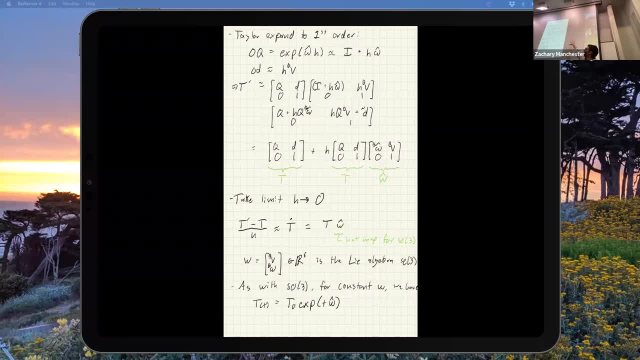 so all these like new things you can kind of like keep stuffing into this group and make a bigger and bigger matrix and um and it still maintains this group symmetry property so you can write down invariant common filters for like some pretty interesting things. so cool stuff useful in. 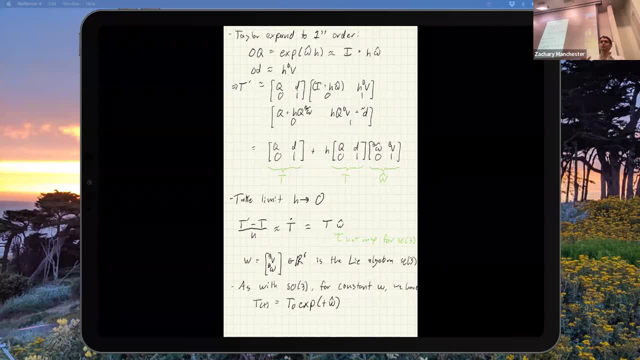 robotics, you get out provable exponential convergence for your non-linear system on in your extended column filter, which is which is slick. so if you can stuff it into a group and show that it's a group, you can automatically plug into like a pretty large body of water. 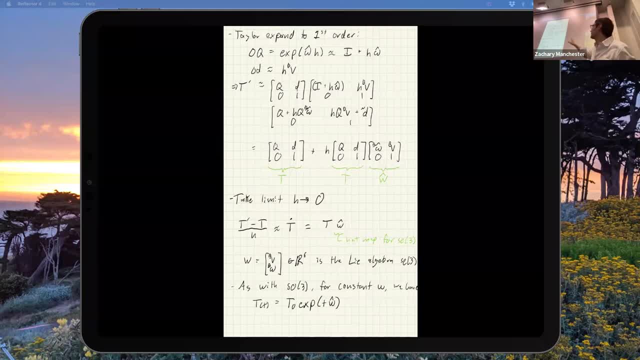 and you can do a lot of work on on invariant filtering for state estimation, and there's lots of control literature on this kind of stuff too, where you can exploit this structure to get like invariant control laws that are sort of written in that tangent plane that don't have to change. 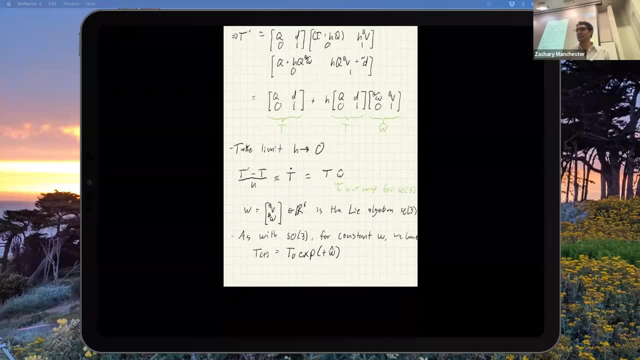 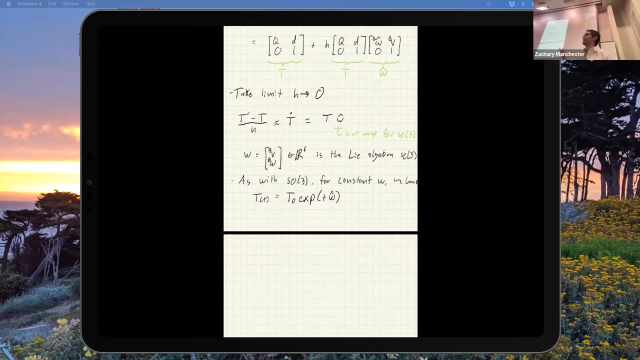 as you move around, which is cool. okay, i'll get on that stuff. yeah. so se3, super, super common. you'll see other things too. like basically, it's become fashionable to like invent new groups for for various robot applications where you stuff various sensors in there, various 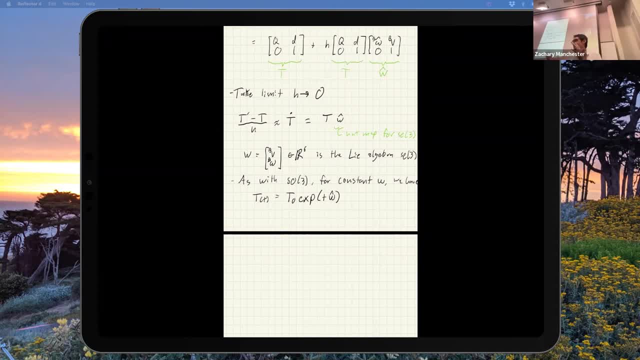 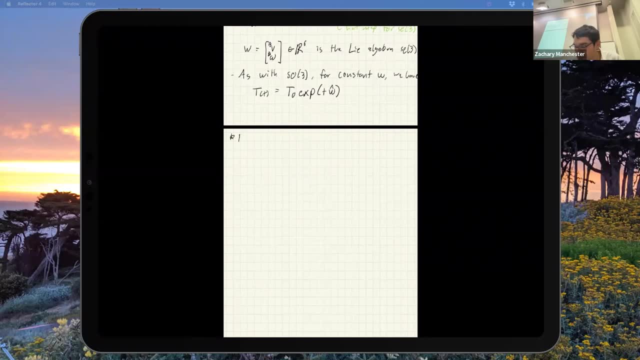 kinematic parameters of the robot and show that it all obeys a group property, and then you can do like fun, filtering things and whatever on it. okay, cool, so we'll do now the full newton euler dynamics. uh, on se3. so this is again. we're going to do with the b in the body frame, which sort of you pick up. 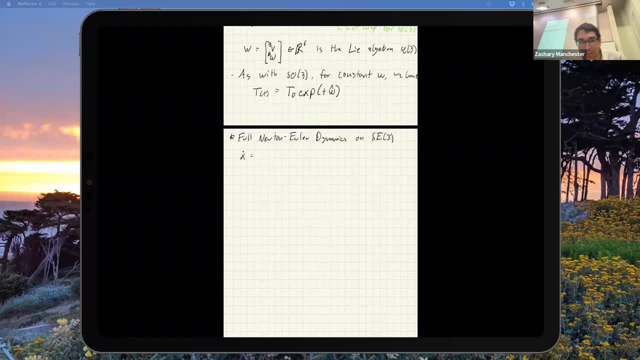 some extra weird terms, so let's make make sure everyone's on the same page with that. so x dot is going to be r dot and n? q dot, which is our usual stuff, then v dot in the body frame and omega dot in the body frame. so the 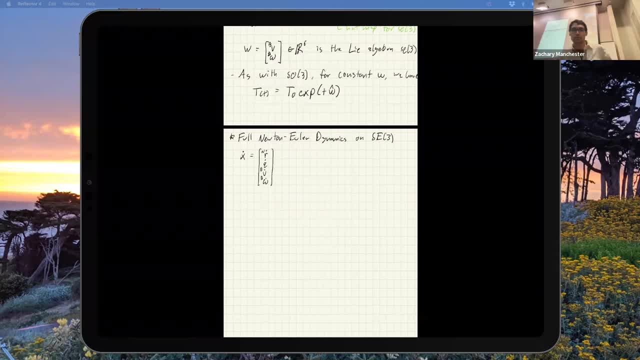 only weird thing here is really the, the velocity in the body frame. everything else is kind of normal, so let's write that out. so, um, the first line, remember our state has v in the body frame, so we've got to rotate that with our quaternion to be in the inertial frame. 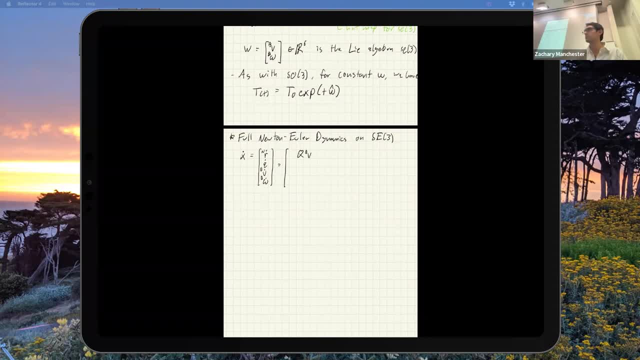 so i'm going to write like this just for the rotation matrix, because it's quick and easy, but you know what to do there from last time. so that's pretty straightforward quaternion stuff we know from before. so i'll just quote that. this is sort of our left hand quaternion: multiply our like hat. 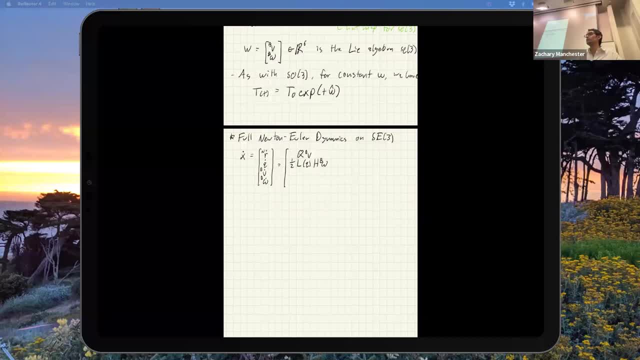 matrix and then like our omega in the body frame. so we did this last time. cool that this, by the way, that whole l and r and each notation that is our special, made up in my lab notation you'll. it's starting to catch on. you know there's some other papers that do it, but like we kind of. 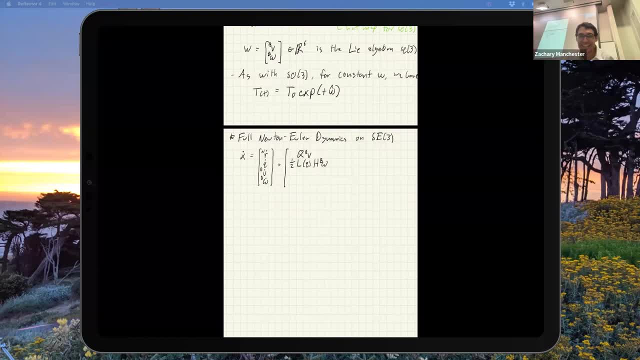 made this up so you may not see this too many other places. um, just fyi. i think it's the cleanest way to do it, obviously, because you know, whatever it's our own brand. but just fyi, um, okay. so then here's the weird part. right, so this is: f equals ma in the body frame, so we're going to write the. 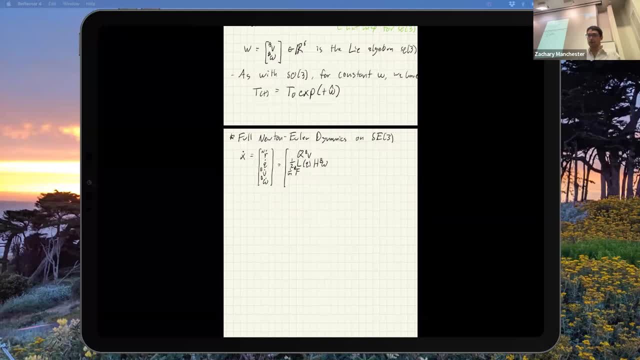 forces in the body frame and, um, i guess i'll just write this down and i'll show you how to get it. you're going to pick up an extra like coriolis term associated with the rotating frame and that looks like this. again, we'll write it out in detail to show you how to. 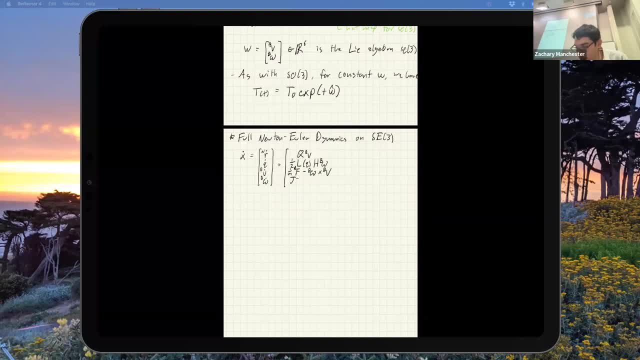 get it. and then the last line is just standard euler equation, just kind of solved for omega. so we take um everything to the right hand side and invert j. yeah, the inertia is always in the body frame, that's okay. so now, how did i get that? so this: 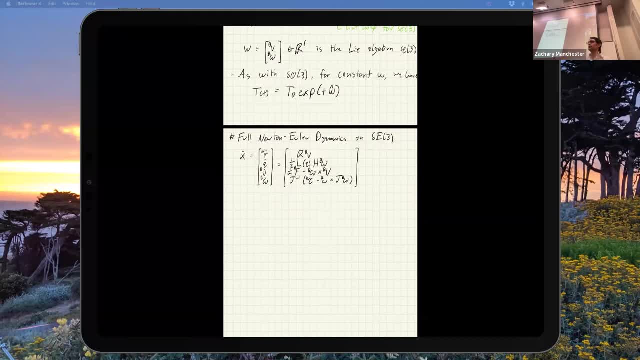 is clear: the top line is always in the body frame and then the bottom line is always in the body frame. that's okay. so now, how did i get that? so this is clear: the top line is always in the body line. is clear, right? i just literally rotate b in the b frame into b in the end frame and then i just 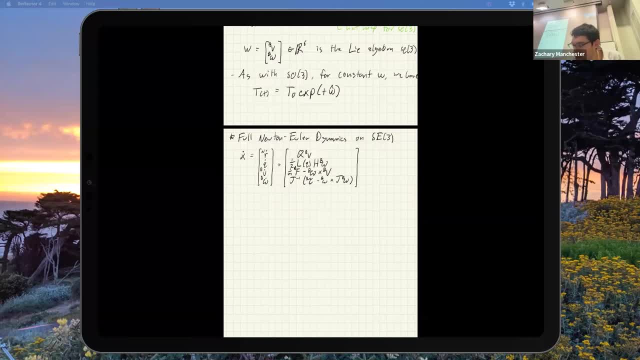 you know, usual integration. this, this one's a little strange, uh, so let's write this one out in detail. okay, so this the way this works. um is all right. so i'm going to write down: v in the end frame equals q times v in the b frame. 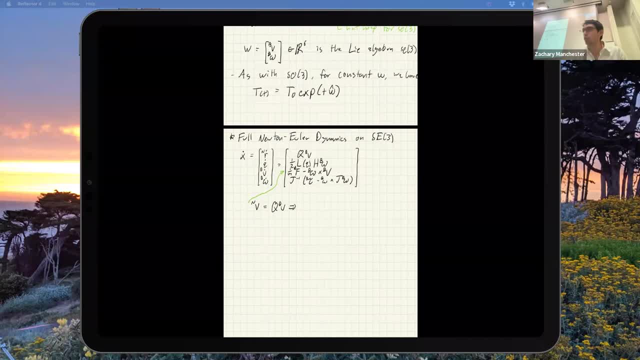 that's super clear. that's the top line. now i'm going to differ, differentiate this with respect to time on both sides. so i'm going to differentiate this with respect to time on both sides. so i'm going to get v dot n equals q dot v b plus q v dot b. cool, so far, so good. now, 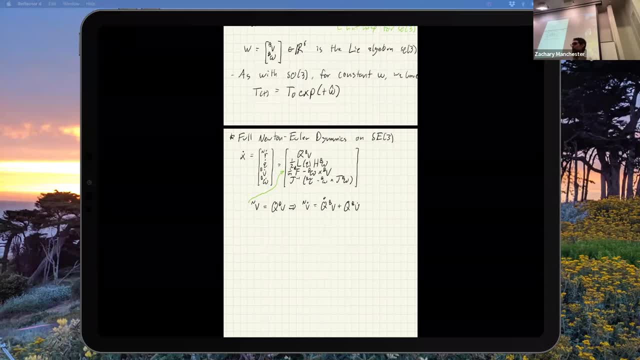 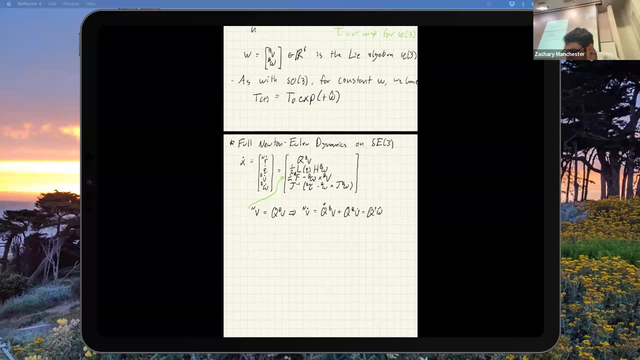 i'm going to plug in the kinematics for q dot, which is that q omega hat guy. so i get q omega hat b frame. uh, v b frame plus q v dot in the b frame, cool. and the last thing to remember is: this is so this v dot, this? 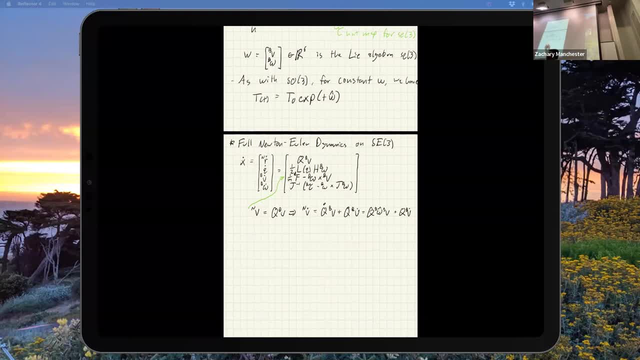 is a in the inertial frame, so that equals ma in the inertial frame, right? so i'm now going to write down: you know, this whole thing equals one over m times f in the end frame. so i just wrote down: f equals ma. and then i went through all those gymnastics. 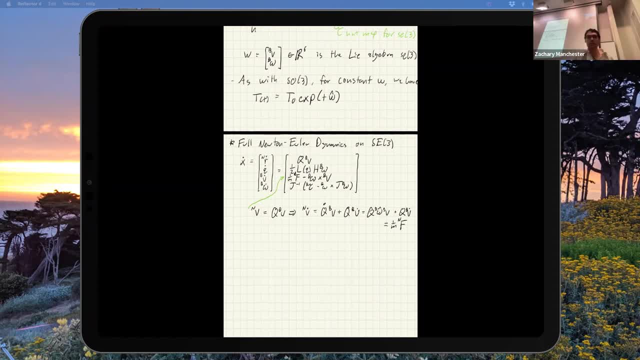 so i sort of write it in the body frame and i picked up that extra term right. so this whole thing tells me. now, if i want to write the whole thing in the body frame, i'm just going to solve this, i'm just going to massage that around and solve it for v dot in the b frame. this is the. 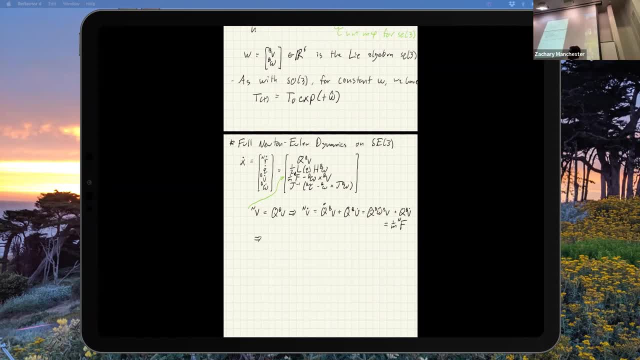 guy i want, right. so i'm basically going to like sort of move the q's over and whatever cool. so here's: v dot in the b frame equals one over m, q transpose because that's q inverse f in the end frame, minus omega cross v. cool, i'm going to do it. so i just took the, the q's. 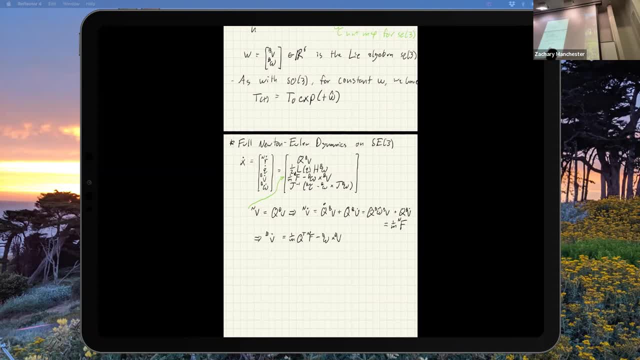 and multiplied here by q transpose. now the last trick is: what's this dot? so this is f in the end frame. times q transpose, so q is body to inertial. q transpose the inertial to body, so this whole thing is just the x in the body frame instead of the inertial frame. now 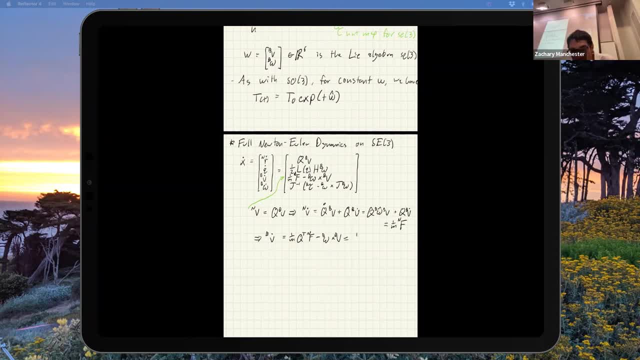 right. so now we get the result we were after. so there you go. so that's where that that like third line comes from, which is um, the f equals ma stuff. okay, so this is fe3 dynamics. the fe3 part is really the top two lines, it's right. the kinematic stuff, the dynamics part, i guess, is also, but it's basically that. 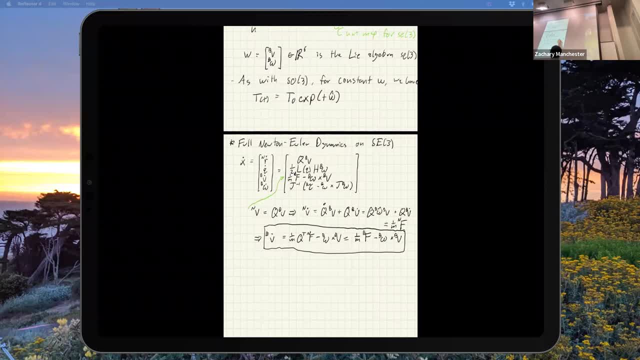 stuff is like right, writing down: f equals ma in the body frame, which gives you this extra term. and then always equation which we already had on the body frame right to be consistent with every, the velocities being the body frame. um, sort of just for completeness, because you'll. 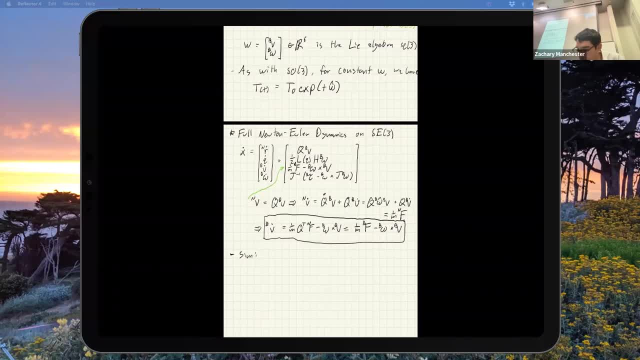 see it a lot because it's super common. if you don't do it the sc3 way, it's sort of um easier, but it's a little bit more complicated than that. so this is the, the stuff you're probably familiar with. more right would just be standard f equals ma, so you'd end up with like x dot equals. 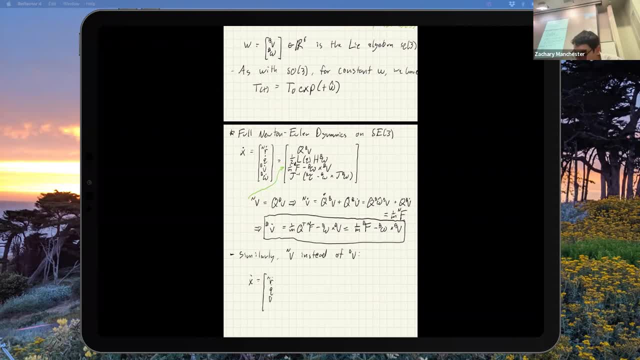 r, dot n, q, dot v, dot n, omega, dot d, and this would just be, you know, v? uh, same quaternion, kinematics, uh, this is now just f equals ma, normal f equals ma in the end frame, and those are the same euler equation stuff in the body frame. 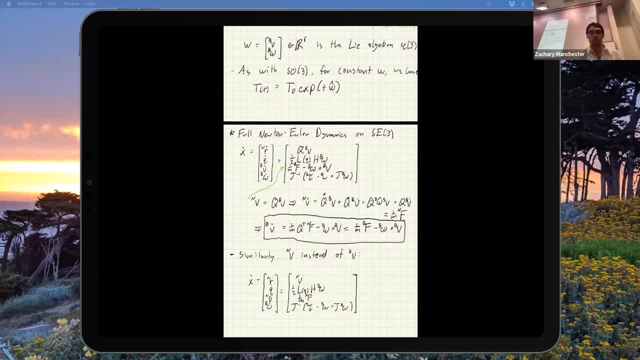 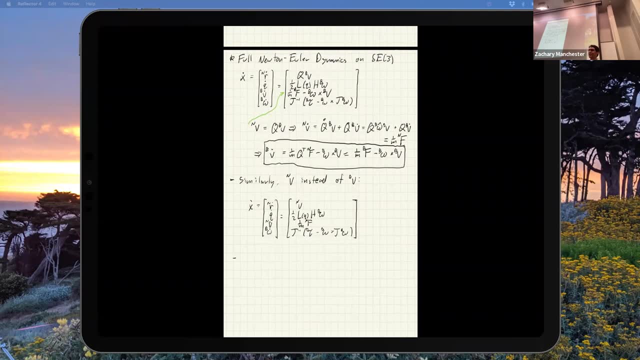 all right, i think that's okay. so, basically, this is the recipe. and now, if you want to simulate any rigid body system, you want airplane quad rotor. roger legged robots are often done this way for weird reasons. uh, i don't know, take your pick, there's probably other ones. underwater stuff, space stuff, spacecraft, um, basically now all. 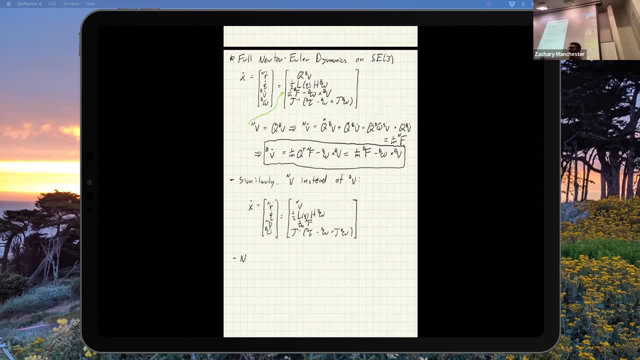 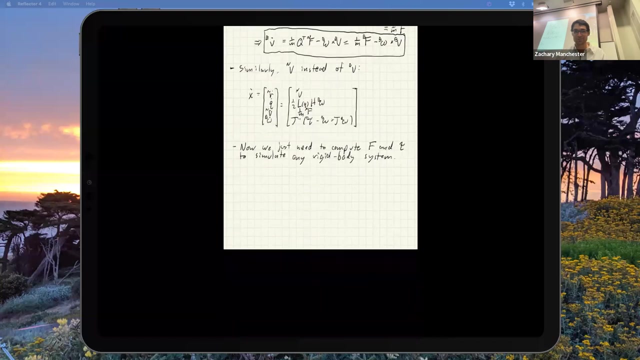 you need to do is compute f and pow. that's it right. all the rest is there for you, and now you can do like any rigid body robot. so this is actually super, super useful. Okay, so let's write down like a couple of the most sort of canonical popular rigid 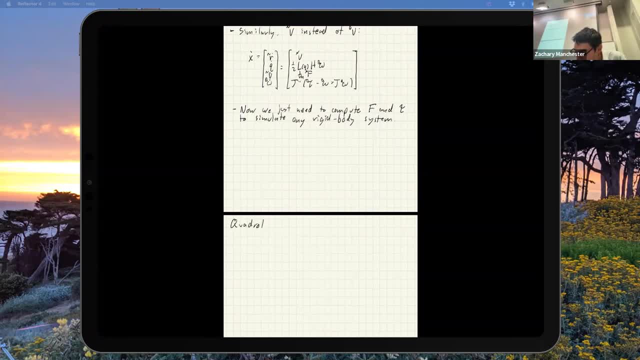 body robots, quadrotors- Those are ubiquitous, right? Everyone's seeing these things. So if you ever need to simulate one- and there are simulators, but if you want to write your own controller, et cetera, you probably want to be able to do this. 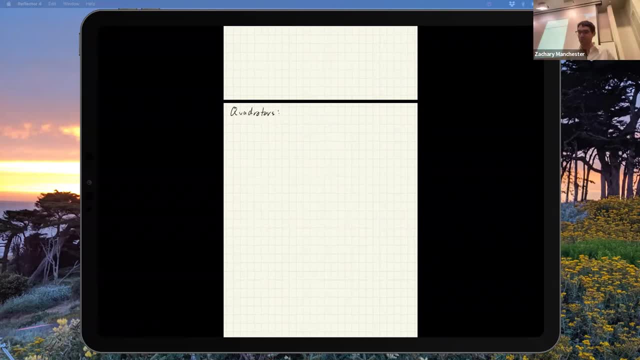 So let's write one down Again. there's like multiple conventions for everything, so always be super careful. So we're going to have like a center mass, sort of in the middle of this guy. We're going to have the four propellers coming off, like so. 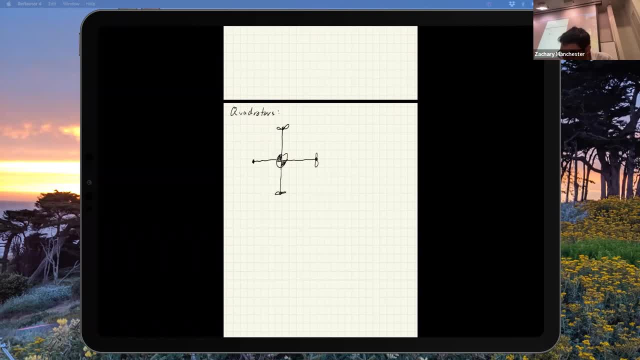 Let's see what do we have here We've got. so I guess we'll make the propellers rotate, sort of like this. So there's a key sort of they do not all rotate the same way, right, So you get opposite torque, so the thing can sort of cancel out the prop torques. 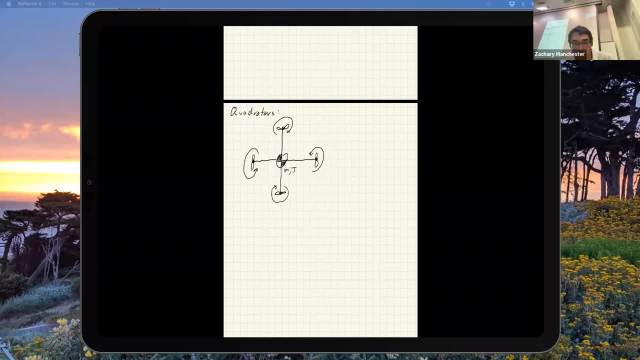 And then we're going to have mass m, Inertia j for the whole thing, And then we'll call these little vectors from the CG to each propeller, si, And this will be in the body frame. I guess it all depends. 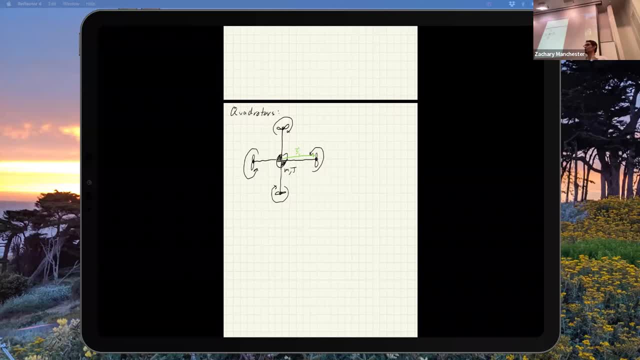 So these guys, we'll see all four s's. So this accounts for whatever the vector is. So it'll be super generic. Let's see: each prop exerts a force Which is thrust in the b3 direction, right? So if we pick a same coordinate system where the z-axis of the body frame is up like unless 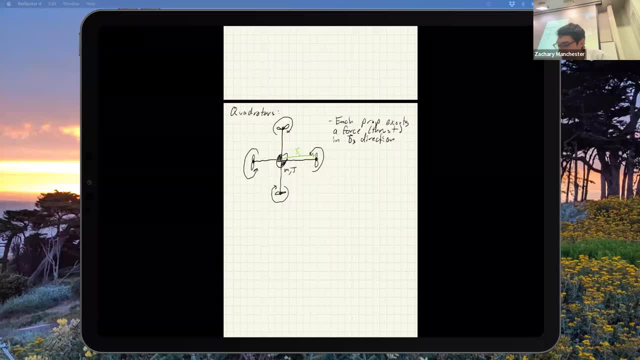 you're a weirdo, that's probably what you would do, So we'll go with that. And then so you get a thrust in that up direction in this frame, You know, Out of a Page, And then you get a torque also about that, a prop torque. 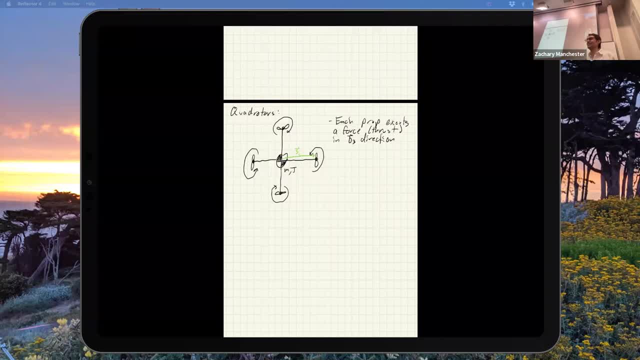 Does anyone know why you get prop torque? Like what is that? How to think about that? So you get thrust. obviously That's what you're trying to do with the propeller, right? Why do we get a torque? Yeah, so, but where does it come from? 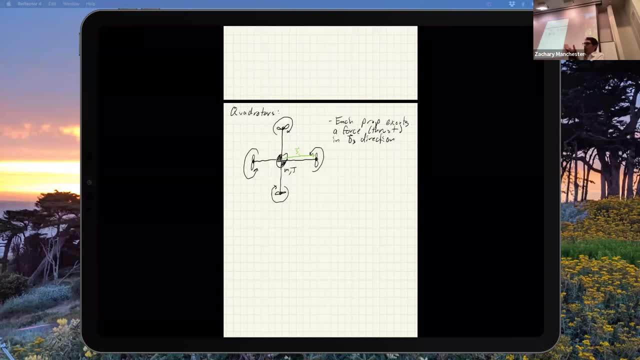 No, well, sort of yeah, So what it's actually coming from right is the way to think about this- is: each propeller blade is actually a little wing, right? So the wing generates lift And drag. The lift is your thrust right. 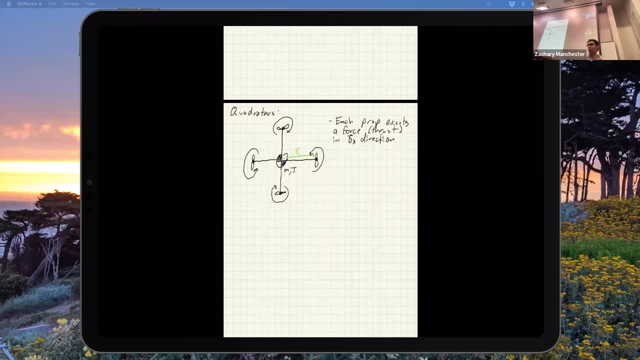 The drag on the propeller blade ends up being your torque, right? Does that make sense? So it's literally getting drag and it's spinning around. The drag force is sort of acting against the motion of the prop And as I sort of integrate that around a rotation, I get a torque. 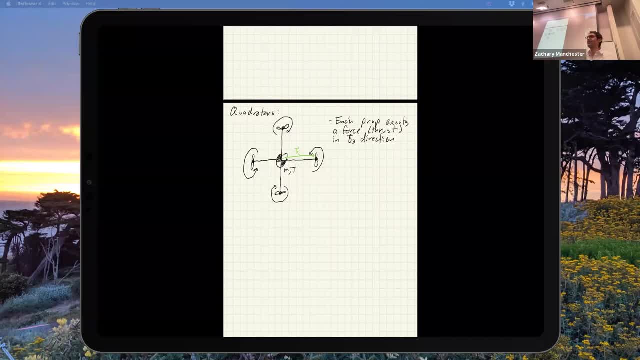 So yeah, literally, propellers are just little wings, And that's the way to think about them. They're little airfoils. This is also why they twist. by the way You notice, propellers are never like straight. They always have this like twist to them. It's because the propeller is just a little wing. The wind velocity over the propeller changes as you go out from the root to the tip. right The tip is moving faster And inboard it's moving slower. So you actually want to vary the angle of attack as you go out right. 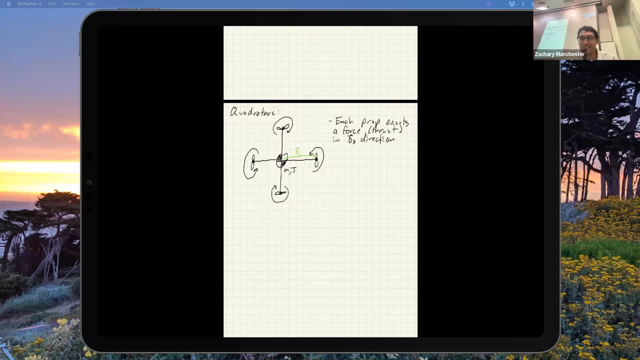 Because the airflow is different speeds, Anyway, that's a whole other thing. So you get torque in the sort of plus or minus B3 direction, And that's what we're going to do here. We're going to do a drag, We're going to do a drag. 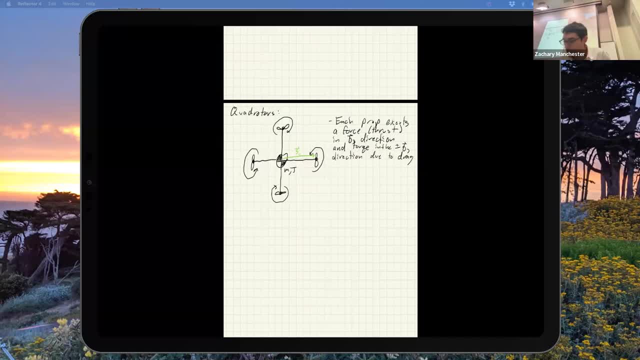 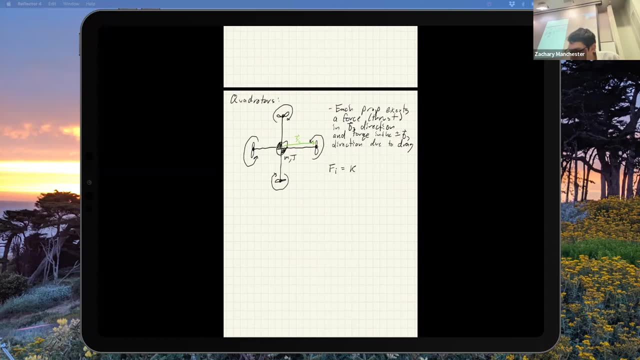 We're going to do a drag. OK, so you get. so if I write on all the forces, I got fi equals kt times u, So this is sort of typical. There's more complicated versions of this that account for more stuff. 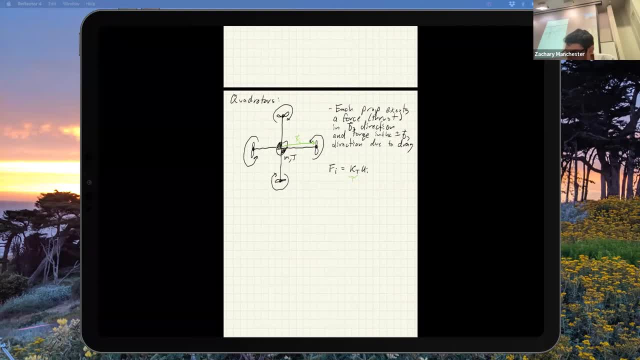 But basically sort of like to first order. this is called the thrust coefficient And if this is times your input, assuming that's like some motor current or whatever command, this is typically how it works out. to first order Again more complicated stuff. 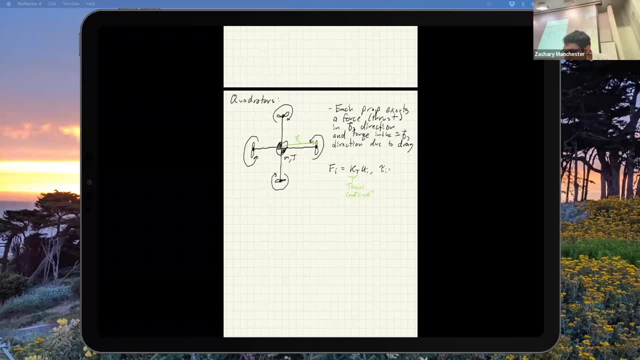 And then your torque is going to be like a. this is called the moment coefficient times- again your ui, And these are actually specs on the propeller. So for a given prop you can either go to wind tunnel experiments to figure this out. 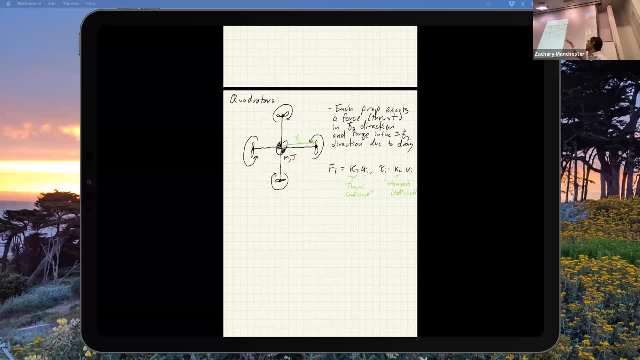 like basically put it on a test stand with a load cell and freestream and like measure this stuff and fit a line to it, Or you can generally for most anything that's like above the crappiest hoppy grade stuff, you can actually find that these coefficients advertised for props. 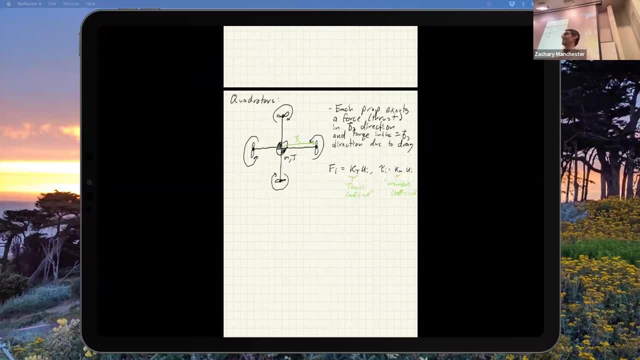 typically Anything above a certain price range. the manufacturer will tell you these: Yeah, So we're gonna. yeah, so this is yeah. so this is where it gets more complicated. So this is assuming basically: yeah, that you get like instantaneous, like that, yeah. 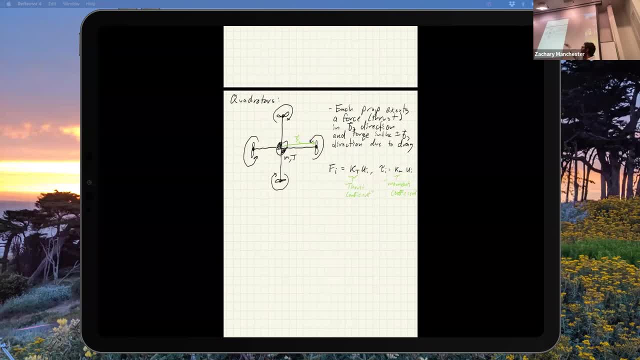 it's essentially like zero inertia that it like spins up instantly when you apply torque to it. like this, A more complicated model, you would account for motor effects, prop inertia effects, And what that ends up doing is you basically add states for these things, right? 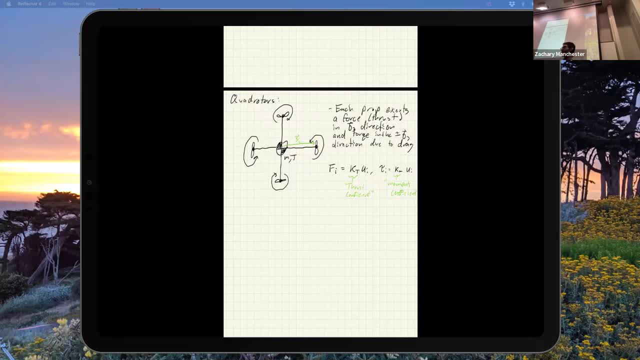 So in practice, like this is really proportionate. It's proportional to like omega squared. So you would write that down and then this would be like a torque And you'd have like Newton Euler dynamics, you know, for the props And you'd account for airflow over the prop in the sort of like horizontal plane right. 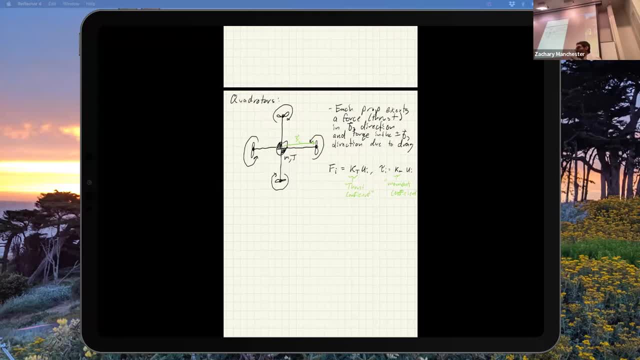 Which is gonna impact this, because now the basically, if I'm moving this way and my prop's doing this, I've got more airflow over this side than I'm receiving blade right. So this is actually the class. this is what sets the speed limit for helicopters. 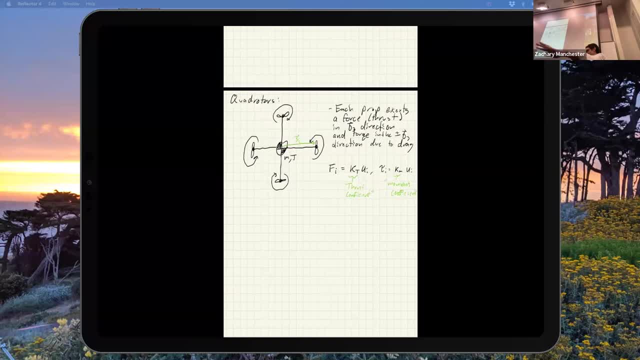 The fastest helicopters in the world top out a little over 200 miles an hour. And it's because it basically what ends up happening is the receding blade ends up installed because the forward velocity is almost what the, you know, matches the receding prop velocity. 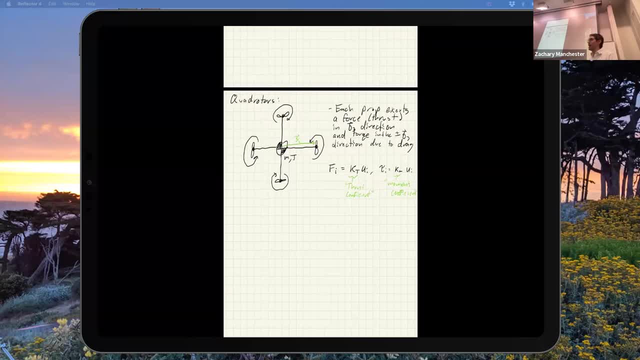 So that's bad. So you end up getting torques because of that, right? So all kinds of bad, weird stuff happens with rotorcraft. It gets a lot more complicated. This is like a good model near Hubbard, And this is what most of the quad rotor control stacks do. 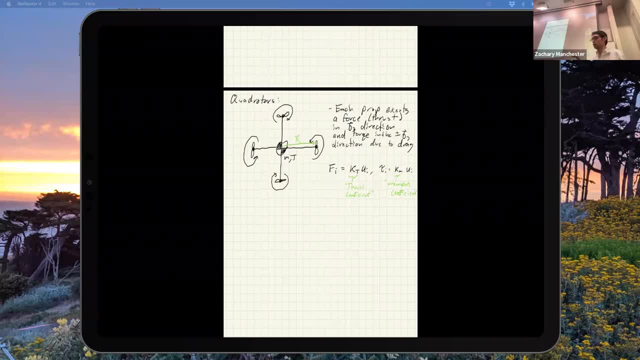 You can get more complicated, for sure, And higher end quad rotor controllers will do some of this modeling, like you're saying, Accounting for prop inertia and more of these aero effects, But the standard, like baseline model that you can use like if you were just right down. 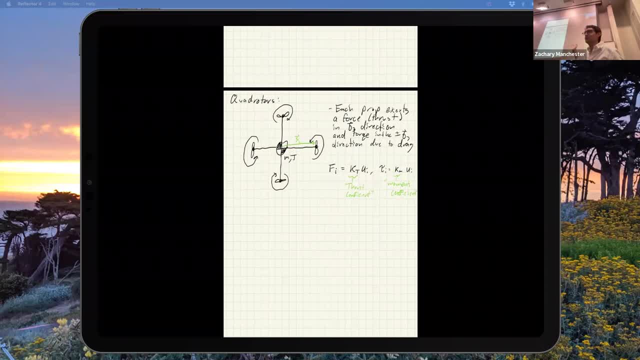 if I just needed to get a quad rotor to fly around in the lab like this is where I would start. If I wanted to get like uber accurate tracking performance and like super aggressive maneuvering, I'd probably start doing some of the stuff you just mentioned right. 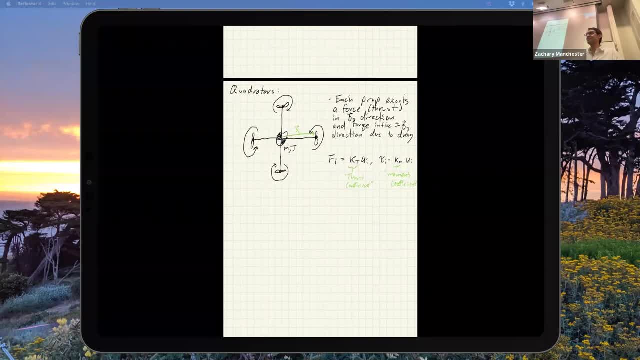 But this is kind of a good starting place. Okay, cool. Any other questions about this? Aerodynamics is hard, But we don't have to do too much of it. It turns out to fly quad rotor. Okay, so sans F and tau are linear in U. 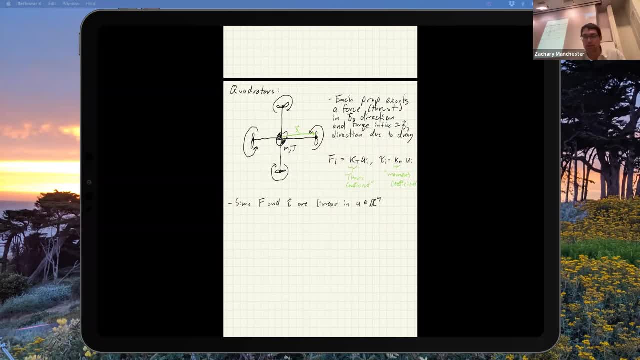 And U remember is four dimensional. I got four propellers. We can write this as a matrix, So we're going to get something like: essentially, F in the body frame is equal to some four, three by four matrix times. So I guess I gave away some stuff there. 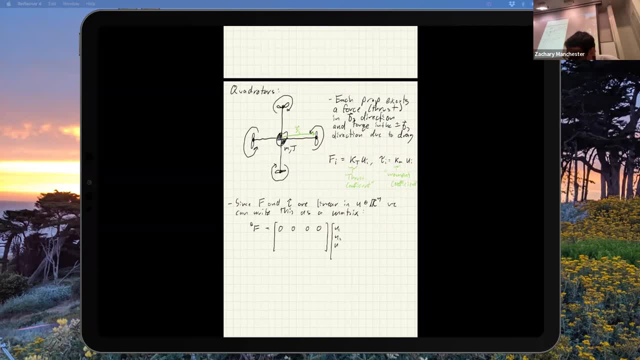 So I've got my four motor commands, and, yeah, this actually varies a lot, right, Because you've also got a motor controller in the mix here, right, When I send these commands to my ESC, whatever. So there's complicated stuff in there too that we're going to ignore. 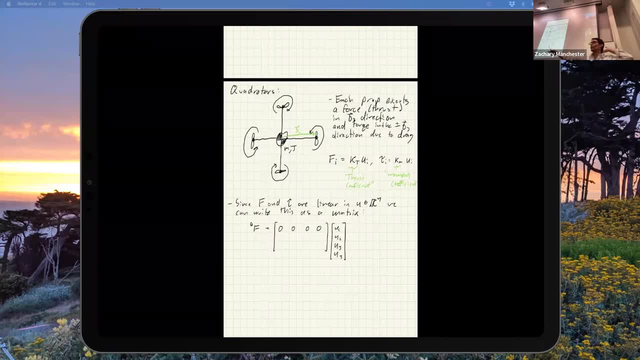 We're essentially going to say: say I'm assuming my motor controller, my low-level motor controller, is good and it's fast And the dynamics associated with the motor controller, like ramping up, are much faster than the dynamics of the quadrotor itself. 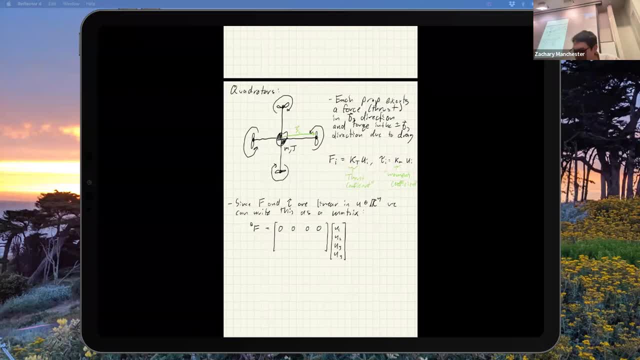 And that's kind of at the heart of ignoring a lot of these things. like you said, like prop inertia effects. So remember, the thrust is always in the B3 direction and it just adds. So we just get this kind of thing for force. simple enough. 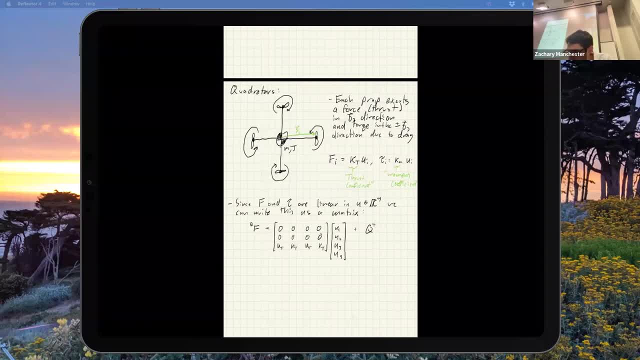 And then we got to get gravity in there, So we get a Q transpose. It's a minus mg kind of thing. And yeah, because remember that's in the minus z direction in the body frame or in the inertial frame, right. 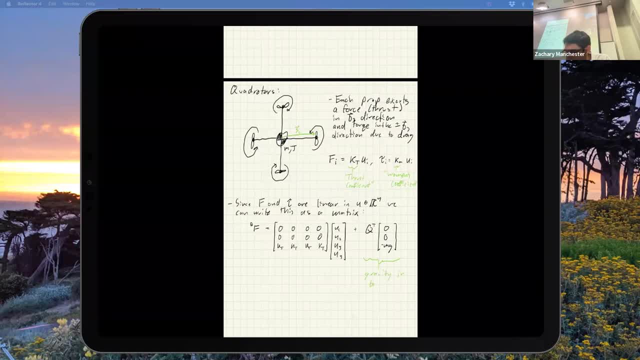 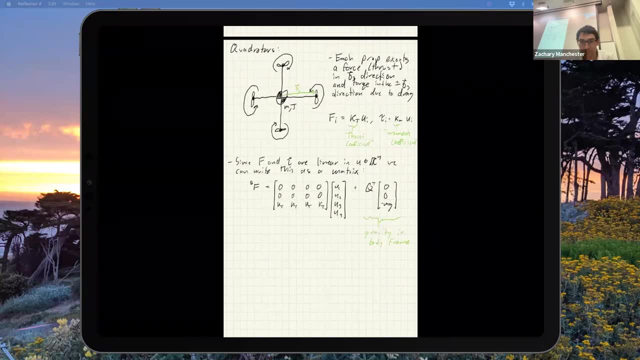 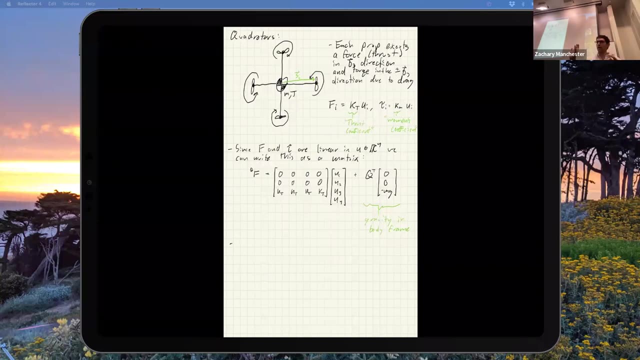 So I have to rotate it, OK. And then we've got to get the torques. So we get both this prop torque and the z direction from drag on the propeller blades, And we also get this cross product term, because the prop is offset from the center mass by these s's. 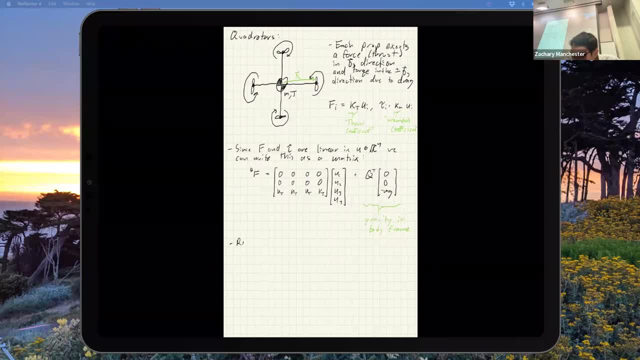 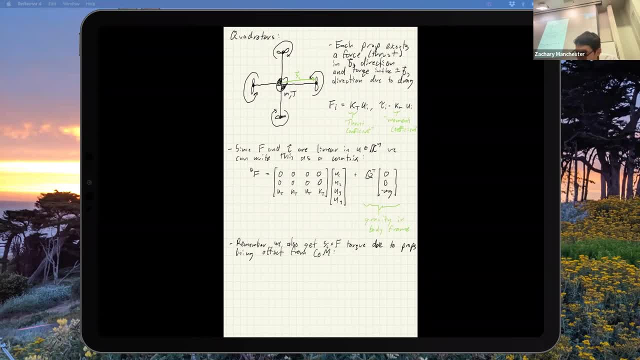 And then we're going to get the s cross, f. OK, So torque in the body frame is going to be first. we get a very similar thing to what we just had up there, where each prop has a drag torque And these are going to flip signs. 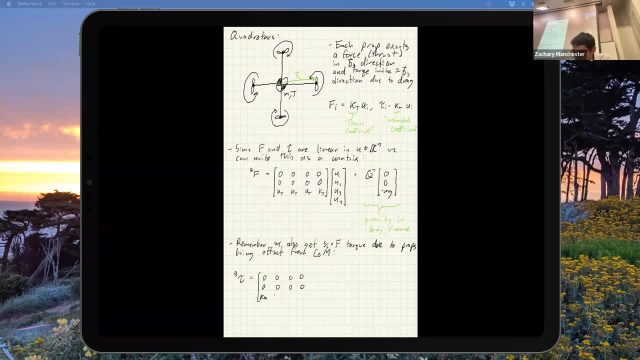 This is where you have to be careful and actually pay attention to your particular quad rotor and your choice of reference frame for the body frame, But basically you make every other one spin the opposite direction so that they cancel out, so that you can hover without getting a net torque right. 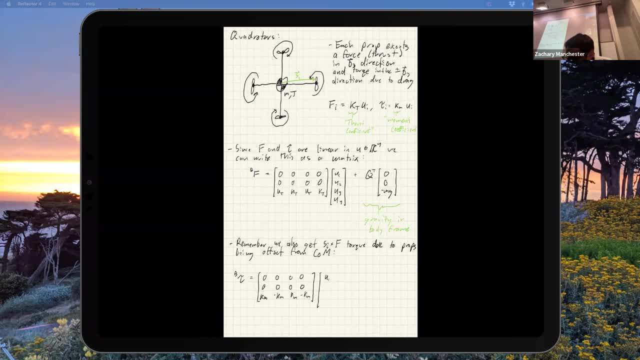 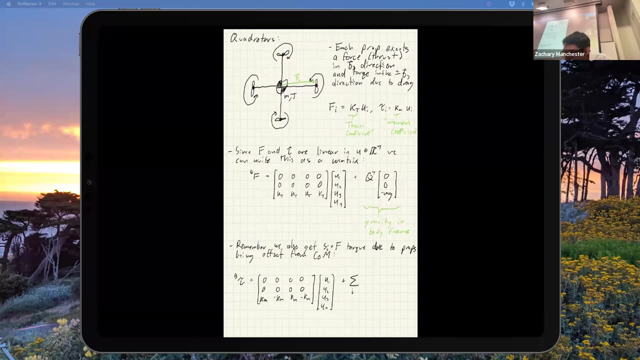 That's sort of the magic quad rotor trick. Look at that, Then we're going to get these. So that's the torque, again the drag torque on the propeller blades, Then this term so sum over. i si in the b's. 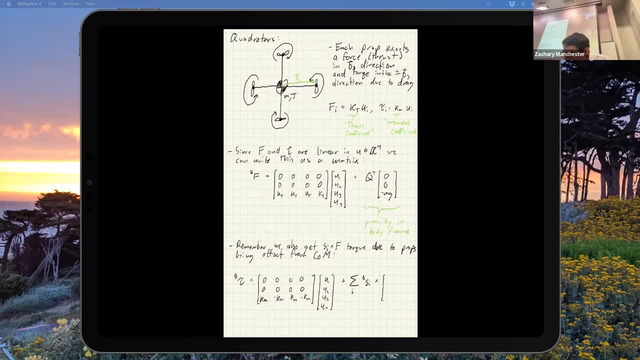 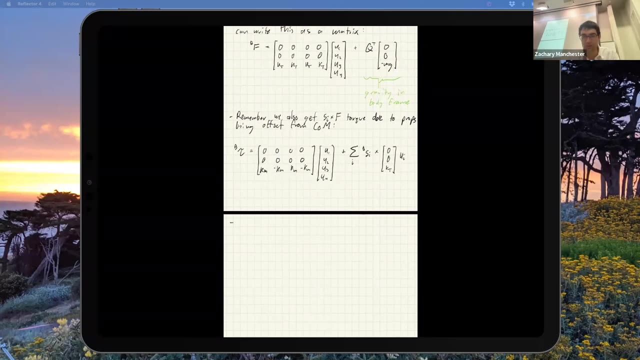 we're going to get kt frame cross each individual thrust right. So this kt times ui kind of guy And basically right now we're assuming you can simplify this some more- which is common. So usually you write down the body frame. 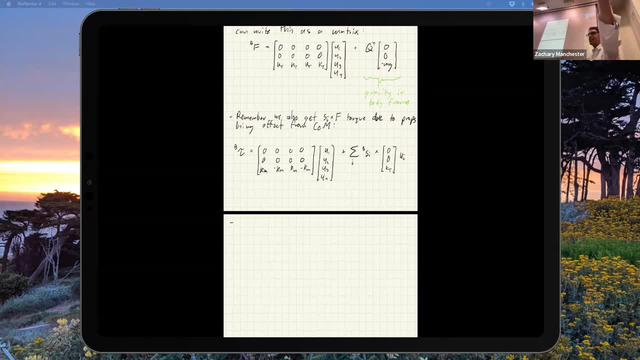 to align with. usually these things are symmetric And you write down the body frame so it aligns up with the propeller, blade, axes or something, in which case this gets even simpler. So we'll do. You can get this down to be like this sort of thing. 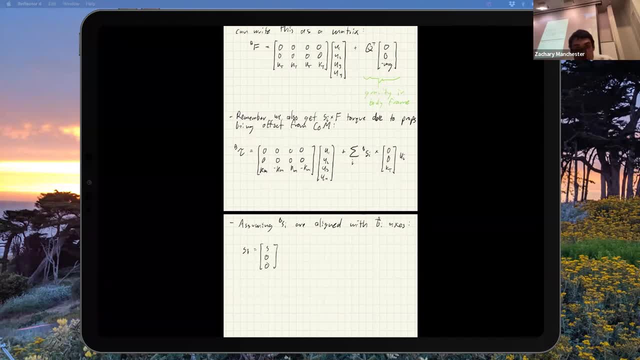 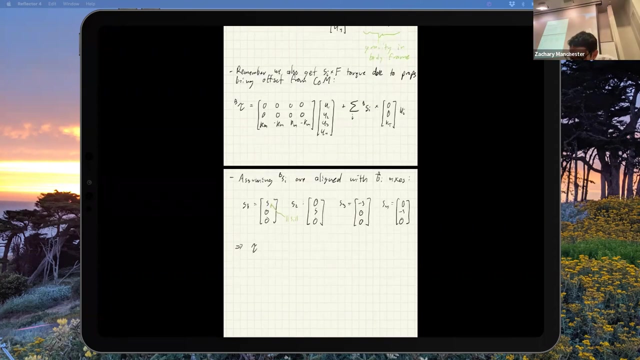 So it'd be like s00.. Something like this: right And where this guy is, norm of the si, And then you get this to look like one big matrix. So it's something like something like this: Cool, Now you're good to go. 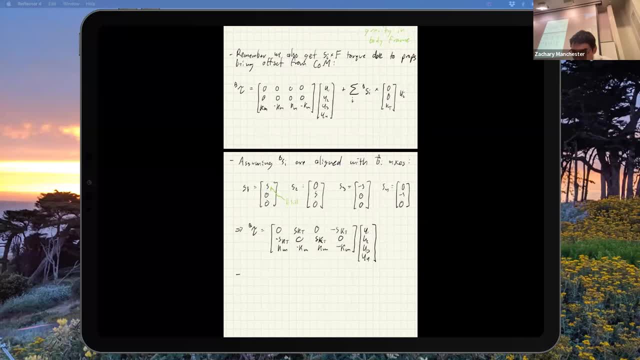 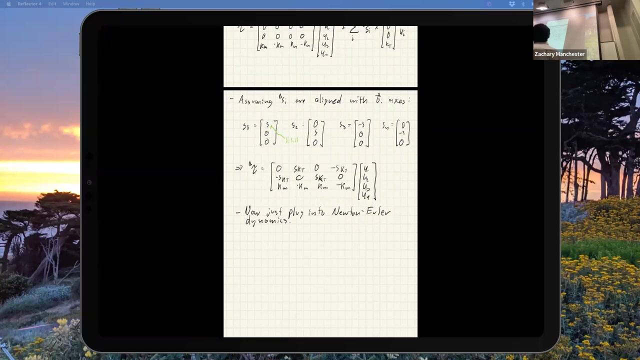 All right, So now you just plug all this into the Newton-Euler stuff. OK Yeah, When s1 equals s, are those the stigmas? These are the norms of the s's. So those little s vectors are like: this is, I'm assuming? 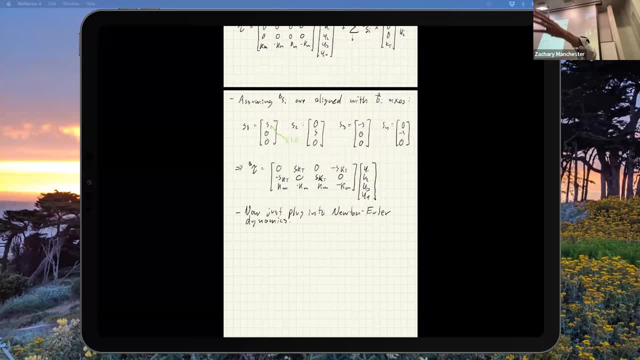 that I've. I'm assuming, a- that the quadrotor is symmetric and, b- that I line my body frame up with the prop axes right So that each prop is just in the x or y body direction. So one in the plus x, one in the minus x, one in the plus y. 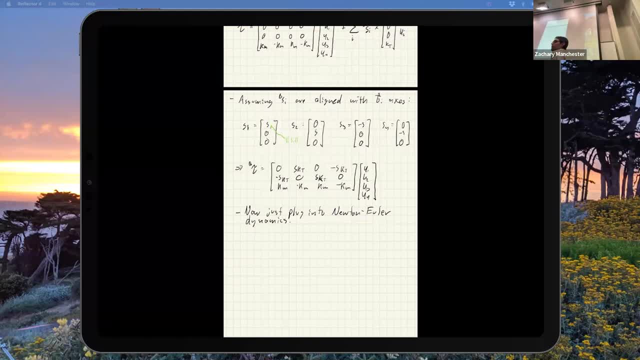 one in the minus y. So then each of these s's just looks like that, right? I mean, is s in that s-point vector the same as s in s2?? Oh yeah, I mean not necessarily, So I should probably number those. 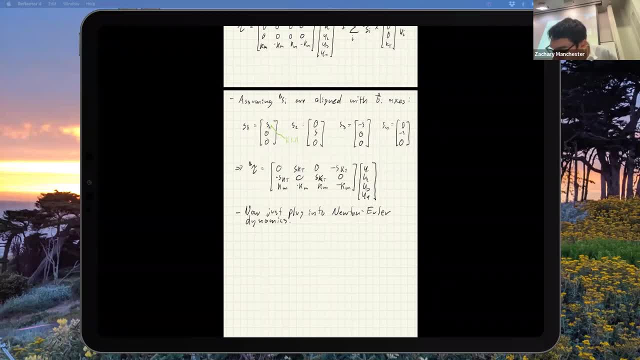 I guess we'll do this: s1, s2, s3, s4. But probably these are all the same, or at least two of them are the same, and the other two are the same. that kind of thing. right, based on what your quadrotor looks like. 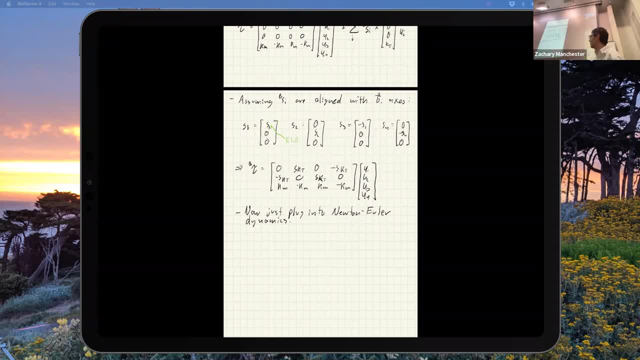 This is pretty normal, I guess is what I'm saying. You'll probably see something like this. You'll see some input Jacobian thing with a bunch of prop coefficients and these lengths associated with the crop motor offset from the CG, And it'll just look like that. 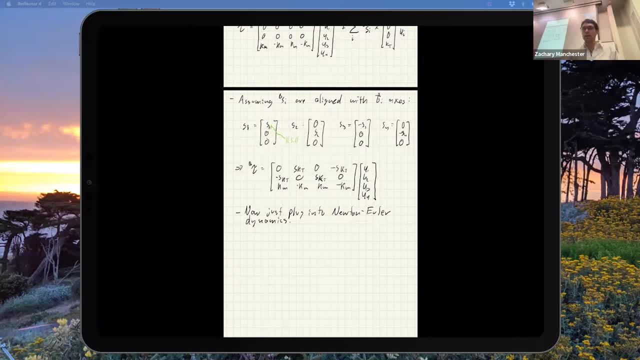 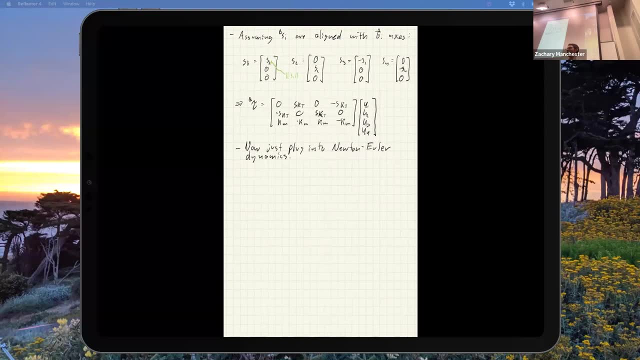 And it's basically linear in the control inputs to first order. OK, so we kind of talked about this. What is missing from this model? Where does this break? basically My thoughts: Airflow, Airflow. specifically, this does model the prop stuff right. 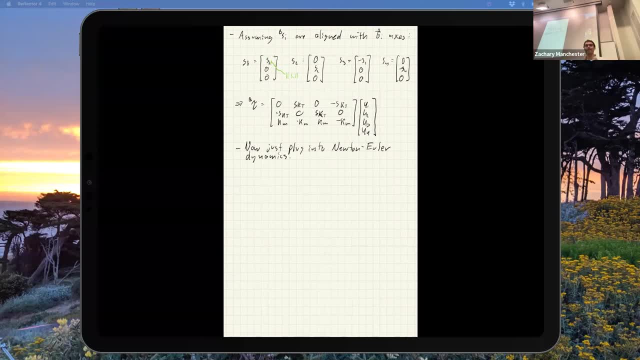 This model is like propeller thrust and drag right, But it's missing any kind of aerodynamics associated with the body of the quadrotor, OK, And it's missing more complicated airflow that happens when you have a non-zero free stream. 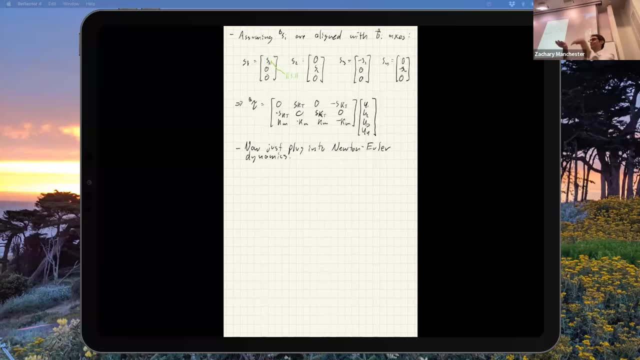 Basically like if I'm moving horizontally and I have some ambient wind sort of blowing over the prop. the other way that messes with this right, Like we said, that induces a torque due to the leading edge going faster than the trailing edge and stuff like this. 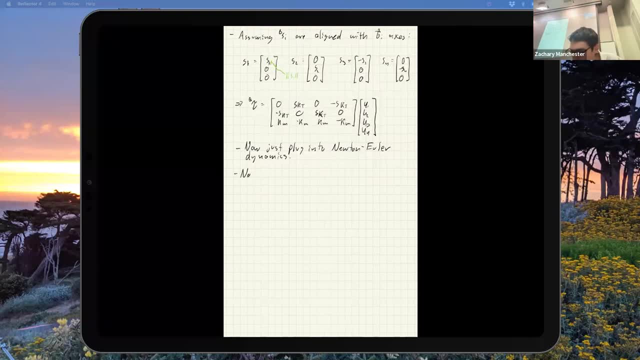 So all kinds of bad stuff happens, right. So we ignored a lot of aerodynamics. Turns out you don't need them. That's kind of a fun thing, right. Aerodynamic stuff is all proportional to v squared, right. Everyone knows this, right. 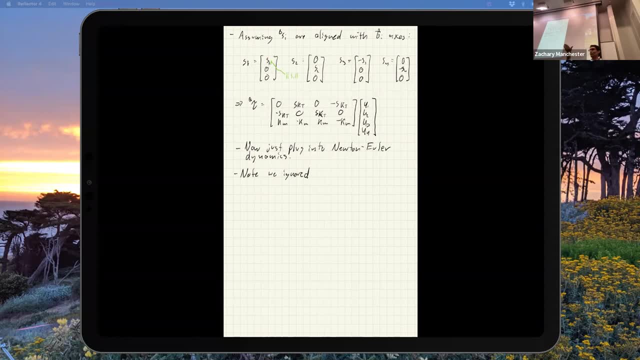 So to first order, it drops out. So if I'm near hover, if I'm not moving very fast and or I'm like linearizing about hover, this is what happens, right? Only the prop stuff actually matters And it's all proportional, like omega squared on the props. 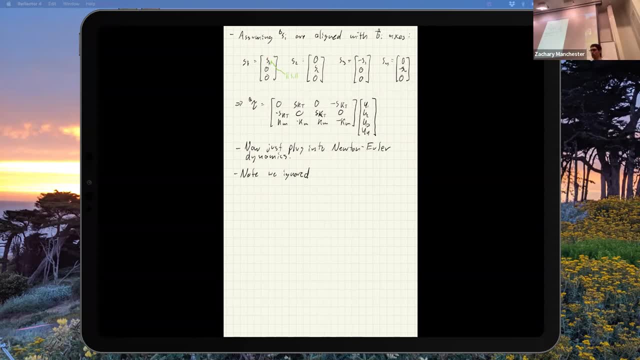 And then all the airflow stuff passed there. it's all proportional to v squared, So it all drops out for small velocities. But if I start to move fast then it starts to matter, right. So if you're doing like crazy aerobatics stuff, 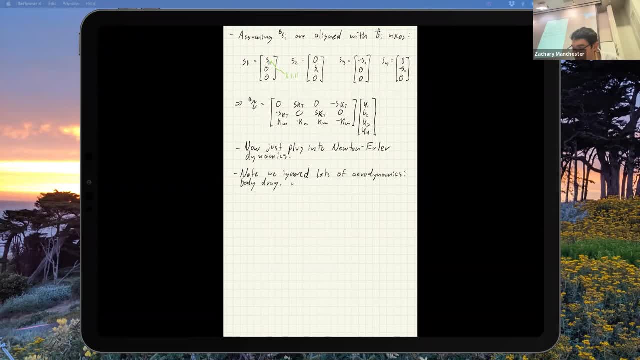 so body drag, wake and boundary effects are another big one. So has anyone ever tried flying a quadrotor near the floor? This actually came up in our seminar talk on Friday. So you get what's called round effect or just boundary effects. 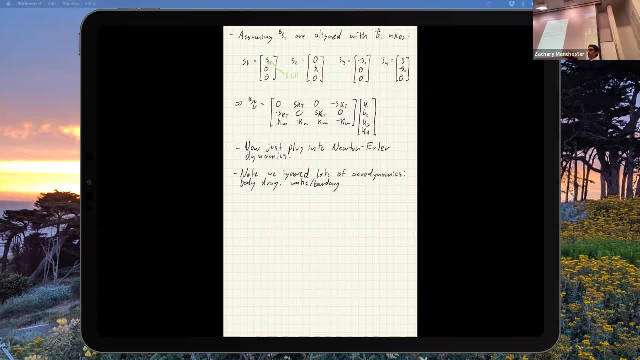 And basically you get this cushion effect from the air, basically bouncing off the floor if you're close to the floor And that actually increases your lift. So yeah, so that's kind of interesting. Same thing with flying your walls: You can get weird boundary effects. 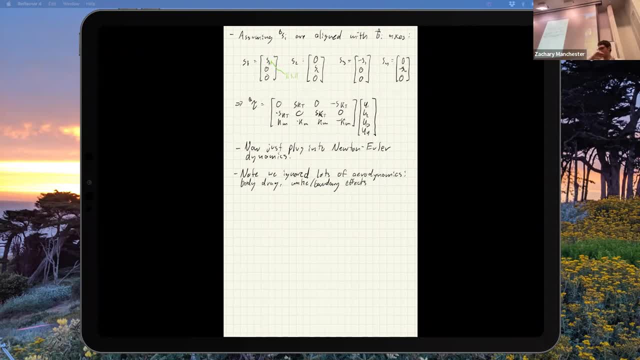 So it turns out with a quadrotor. for this model, the hold- you actually have to be a meter-ish away from the floor, So you have to be up high enough. So in particular, this stuff starts to be a poor model when you go to land. 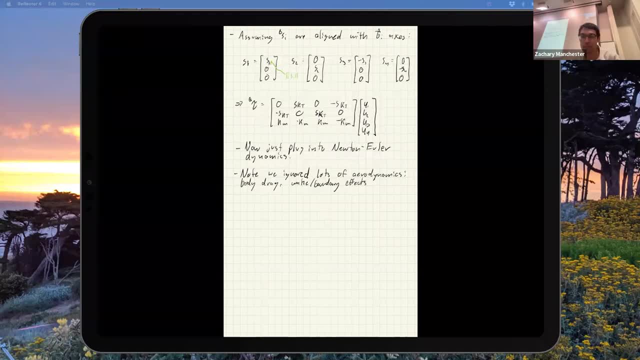 You actually get more, way more lift than the model predicts. when you get close to the floor, Let's see These start to matter, Go fast and or fly near walls, Floor et cetera. So this is kind of where people are into like, so yeah, 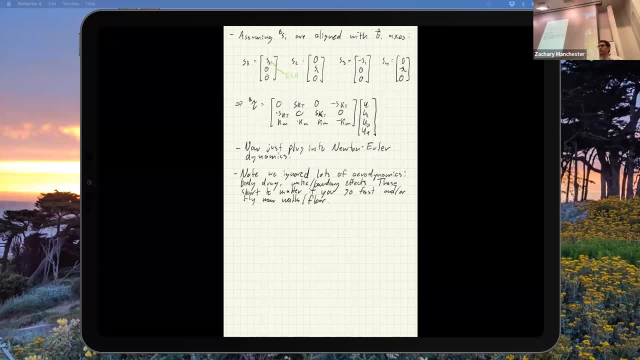 if you start going fast and doing aggressive things, more aero stuff starts to matter- flying near walls, et cetera. So this is kind of where people are into: machine learning, like data-driven modeling of these things. There's a few labs that have done a lot of work. 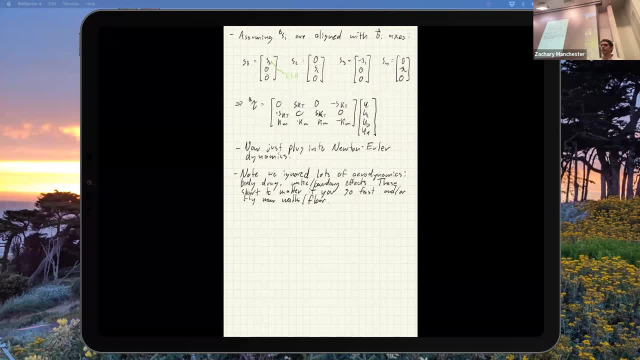 both on constructing, doing residual learning, basically to learn these extra dynamics terms from experimental data to try to do better prediction. So there's a lab, Gabi de Scaramuzo's lab, and Switzerland has done a ton of work on this last few years. 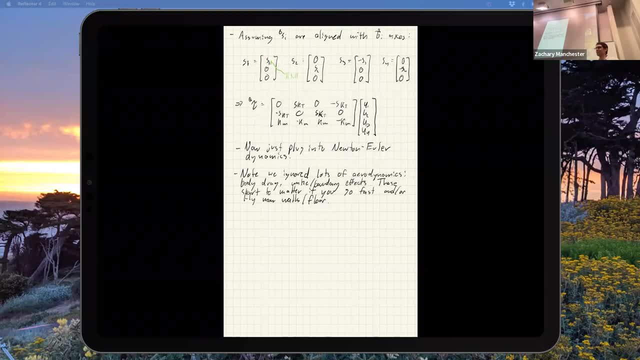 And they've got really ridiculously impressive models now that they've collected tons of data sets in a big mocap arena And they can fly this thing. They can do insane aerobatics and track to a few millimeters worth of accuracy over tens of meters at insanely full out full gas speeds. 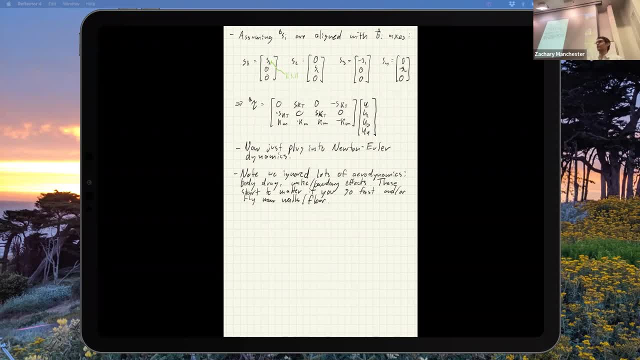 which is awesome, And there's also been a lot of work on just direct policy learning, where you're not trying to build a predictive model, You're just trying to make the controller better. And, roughly speaking, our seminar speaker, Sun Jo, 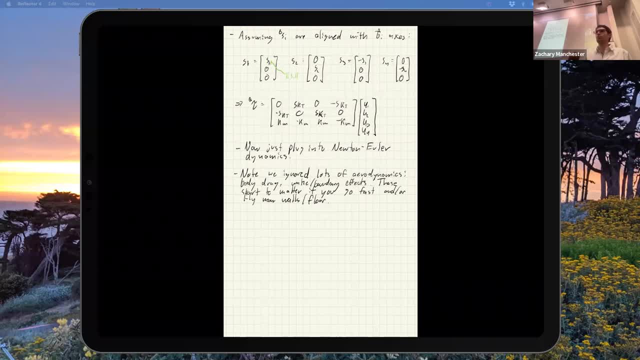 from Caltech who's here Friday. their lab's doing stuff like that, where they're learning controller terms directly, just doing policy stuff. Their particular brand is heavily biased towards giving nice control, theoretic guarantees on performance, But they have specifically some really nice work on landing. 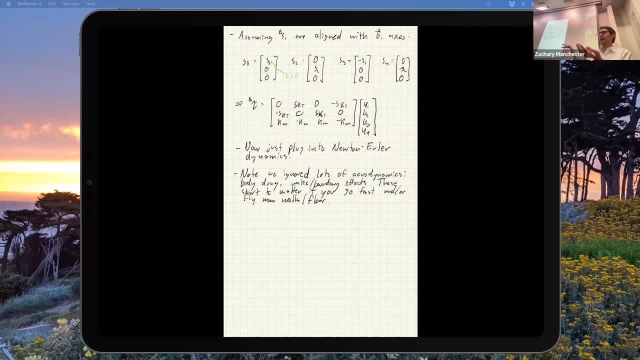 So they call it Neural Lander, So you can basically account for all this ground effect stuff and do super, super fine control, near ground effect, obstacles and stuff like this. They have a pretty slick demo Where they fly over a table where, without their sort of learned stuff, 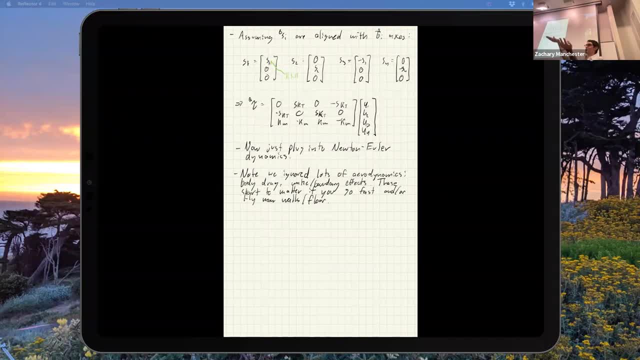 but it does this over the table because of the ground effect And theirs just is like rock solid, straight over the table because it accounts for that effect. So kind of cool. OK, Any questions about this stuff? OK, So then in our last 10 minutes we 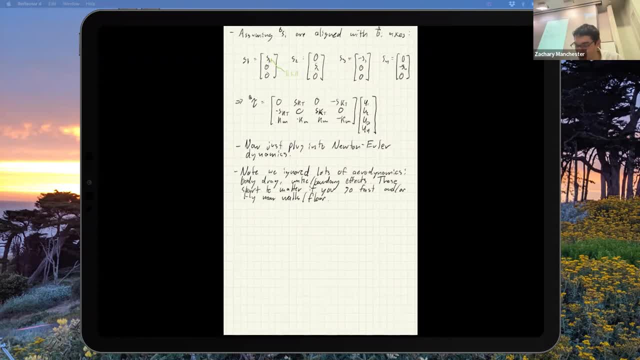 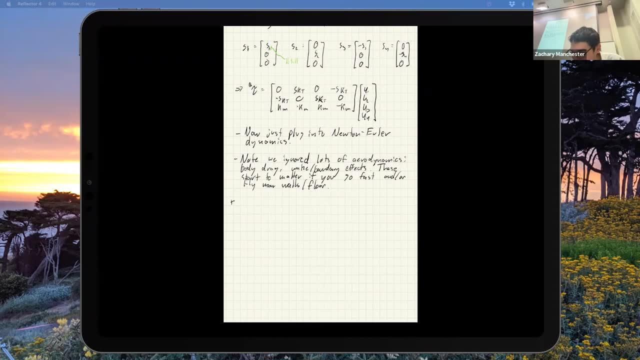 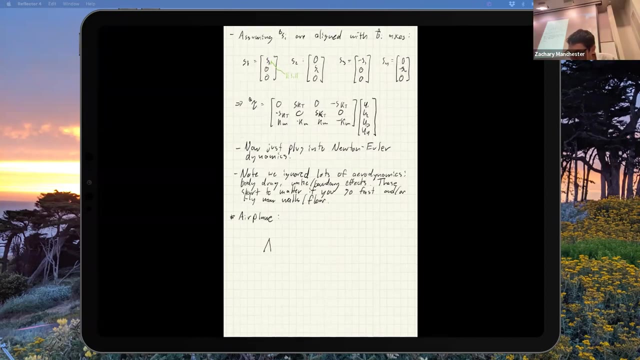 will do a crash course on how airplanes work, after our crash course on how quadrotors work, Because this happens, People do. drones and stuff are important, Right? OK? So let's talk about airplanes. So I will draw a terrible cartoon airplane. 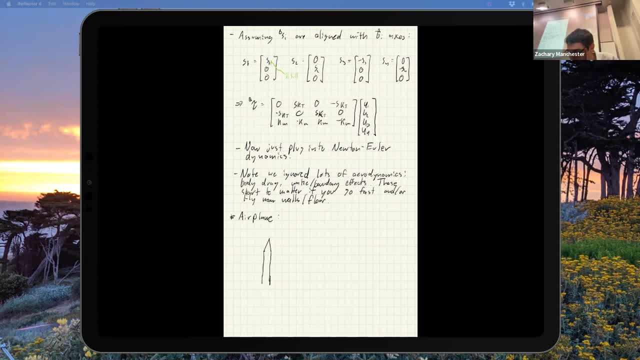 as all my drawings are terrible, Not just the airplane. They're all bad, OK. So we got wings. We got horizontal tail- This is kind of the canonical airplane. There are different versions of this, obviously- And we got our vertical tail. 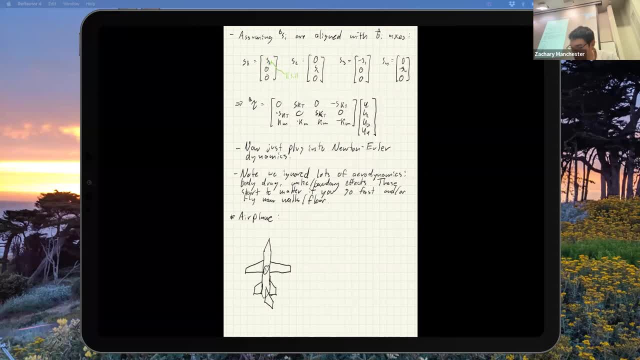 OK, So control surfaces on an airplane And we got the center lift And we got a CG somewhere over here, probably, Actually it should be a little forward. That's probably about It's close enough. Does anyone know where it should be? 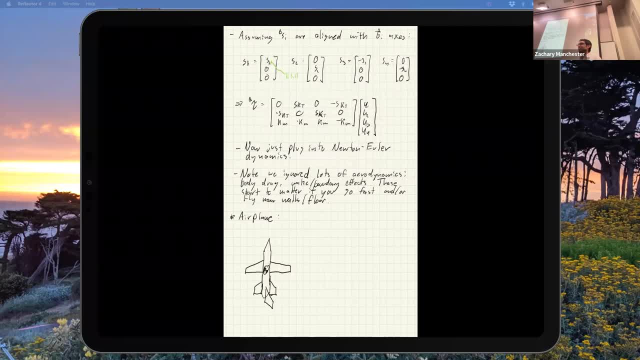 Any aero guys in here? Where's the center lift? That's the question, right? Does anyone know? It's at the quarter cord of the wing, So it's a quarter of the way back from the wing end of the wing. 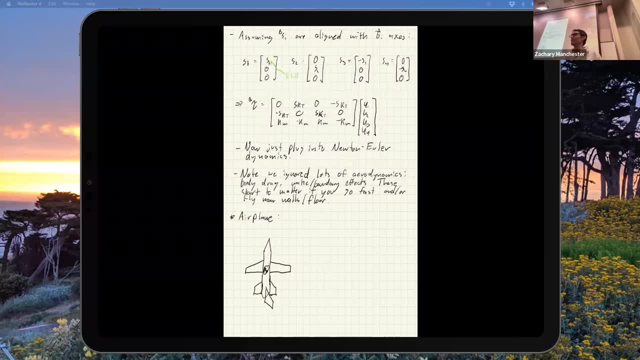 So it's at the center lift, usually Modulo, lots of approximations, right, But so this is kind of wrong. It should be up a little bit more. And then we got, Like, let's say, our propeller up here. 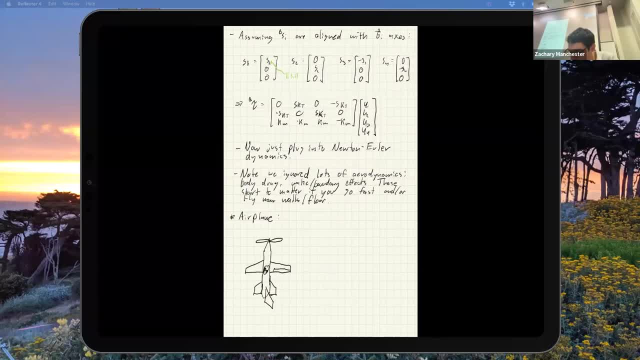 OK, So control surfaces- We got ones on the wing here. These are little flaps that I can actuate, right? What are those ones called Ailerons, right? So those are for controlling roll. You actuate them together where one goes up. 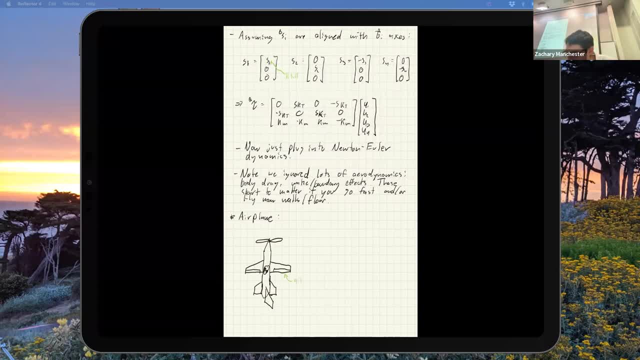 and the opposite. one goes down right to get a torque And then I got ones on the horizontal stabilizer back here that work together. So these guys move up and down together To actuate pitch right. What are those ones called? 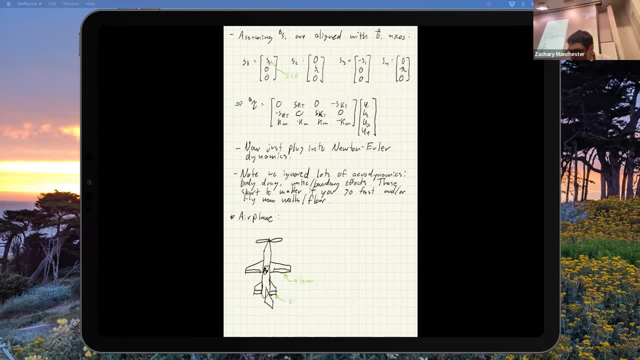 Elevators, And then I got one on the vertical tailback here that I can use to do yaw, And that one- what's that one called Rudder Cool, And then obviously I have my propeller, So the standard sort of set of control inputs for an airplane. 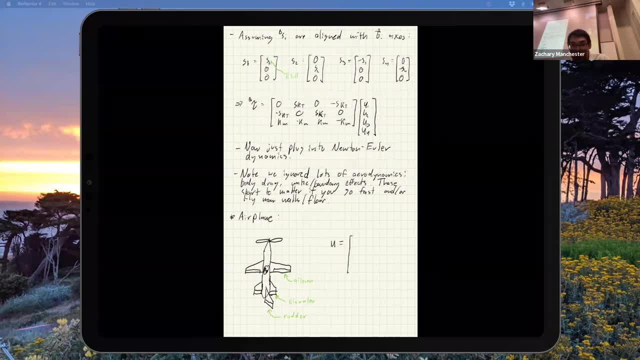 So our U is here. U is throttle, which is related to thrust. It might be like a derivative of thrust or whatever. Then I got my ailerons elevator rudder And sometimes these are combined in weirder designs, But this is kind of your canonical tube and wing. 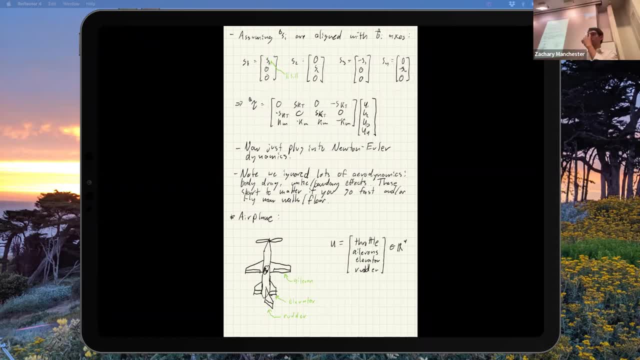 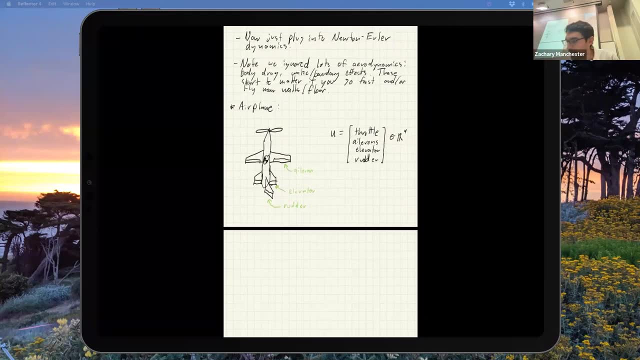 airplane design, And this is again a four vector, So four inputs, Just actually the same number of inputs, right, as the quad? OK, As a quad rotor, And then so we're going to basically use the same sort of propeller model as the quad rotor. 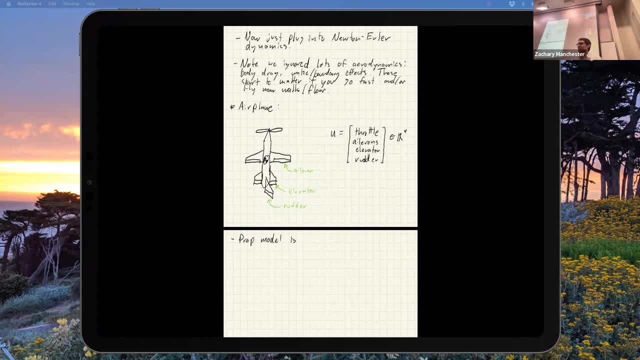 So this is a fun question. So this prop has torque, just like the quad rotor, right? So this airplane always has a torque coming from the prop that's trying to roll the airplane, right? So has anyone experienced this before? Very weird stuff. 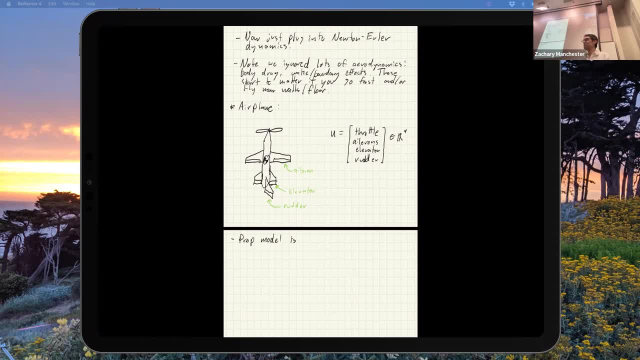 Has anyone tried a small airplane? It's a thing called P factor that is related to this. So it turns out when they build small single engine airplanes they actually build into the airframe. They trim the airframe out at the factory so that it crews it's at equilibrium. 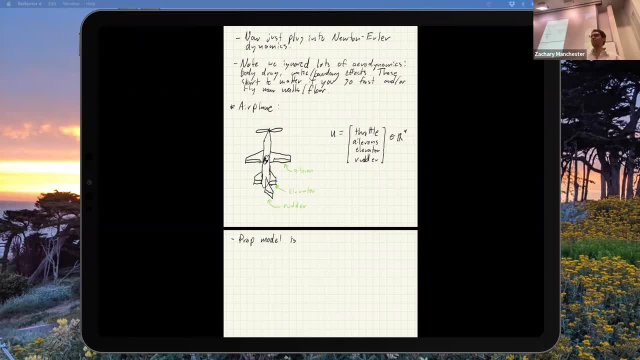 They cancel out the prop torque it crews. That's baked into the airframe, which is kind of wild. So it's like the airframe is slightly biased and twisted, So sort of like all the lifting surfaces have that baked in to cancel out the prop torque it crews. 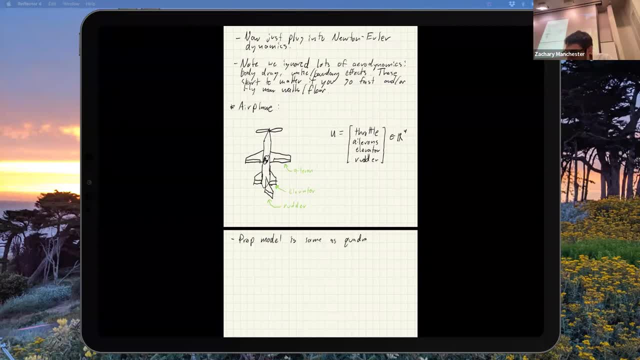 So it's a little bit more of a. So it's a little bit more of a cool. So here's, we're going to get into this whole lift drag thing. So each lifting surface, so like propeller blades, all the wings, vertical, horizontal, et cetera. 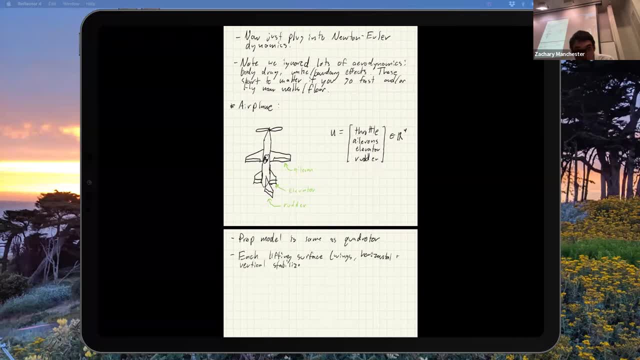 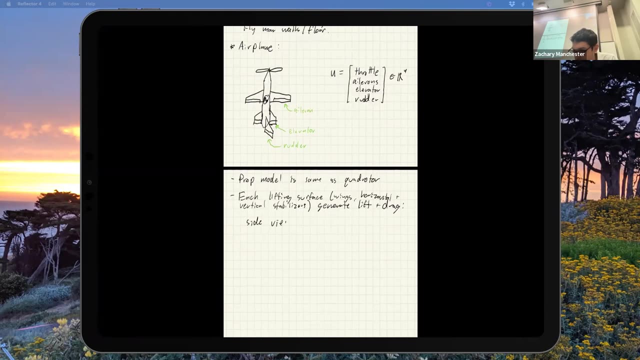 generate, lift and drag. So here's how lift and drag works. So we're going to take a side view of an airfoil aka wing. So we've got the sort of what's typically written as V infinity, which is the free stream airflow. 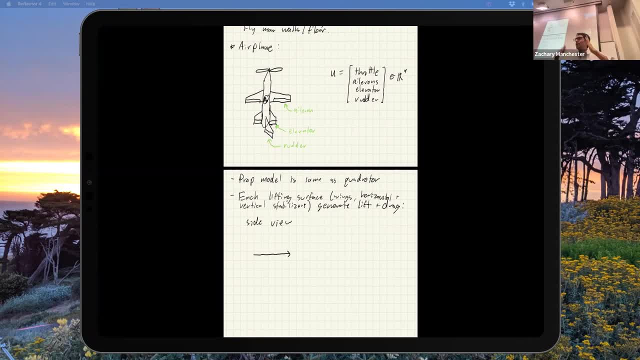 So like if you went far away from the airplane and you just have like wind, right, whatever that is. So I guess let's call this V air. But yeah, you'll see it is written as V infinity, typically in the aero literature. 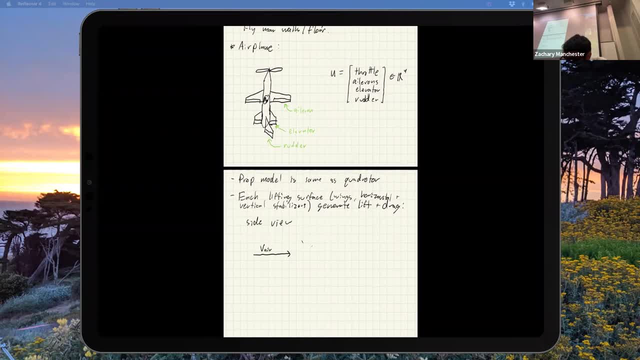 We're going to have our airfoil shape, which again apologies for bad drawing And I will exaggerate this a lot. So here's our curvy airfoil thing. So here's some line associated with the free stream airflow, This angle between the free stream airflow and the wing. 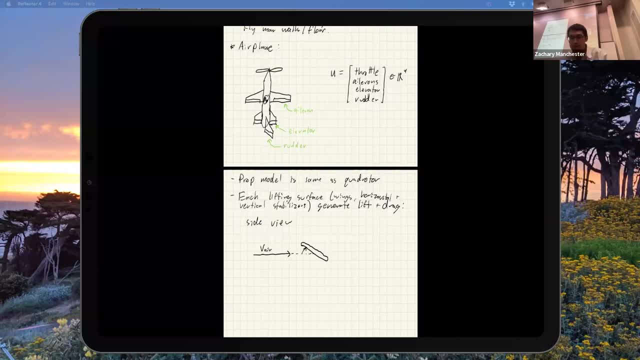 then we know that's called angle of attack, right, So that's written as alpha. And then so that's the angle between the free stream, oncoming airflow, and the lifting surface, the wing, And it's written in And we then decompose the forces, the aerodynamic forces, 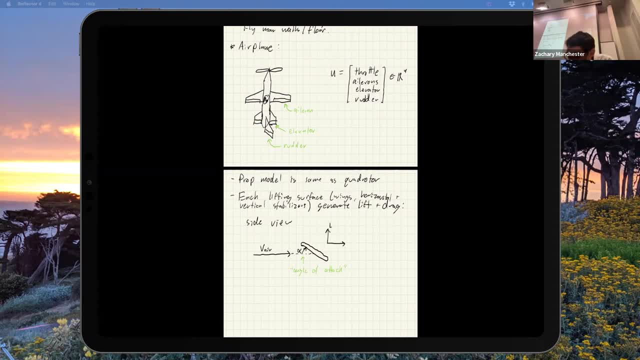 on the wing into two components That we call lift and drag And, like this, F may be something like. it's probably something like this, roughly right, It's some 2D vector right, And we're going to just decide to write it. 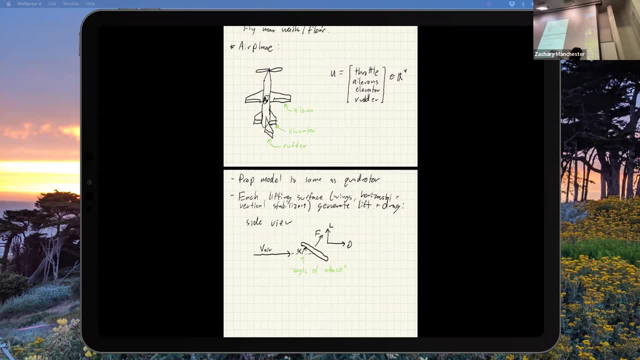 in these two components, L and D, And the specific thing to keep in mind is that this, with the drag frame, it's called the aero frame, It's associated with the free stream direction, It's not associated with the airfoil. 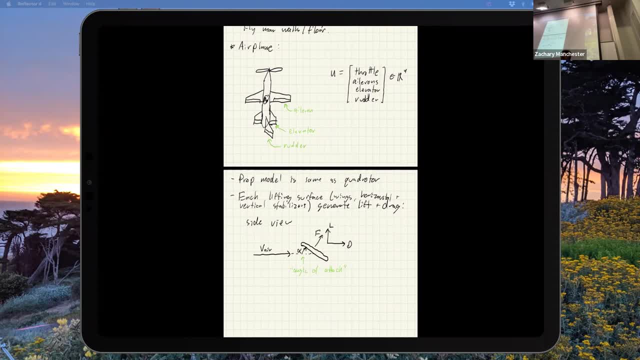 It's not associated with the wing or the airplane, It's the wind frame. is. what we're doing is where we're decomposing this into right So that messes people up all the time, And it's all coordinate transformations. So, basically, what we have to do is we take our airplane stuff. 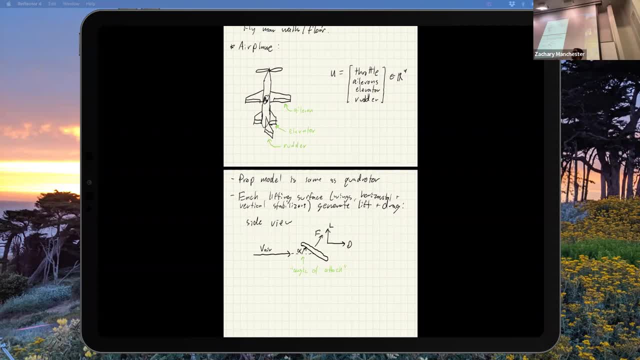 We rotate into the wind frame to compute lift and drag forces And we rotate that force vector back from the wind frame into the body frame to tack it onto our dynamics. OK, So what do we do? What do we do? What do lift and drag curves look like? 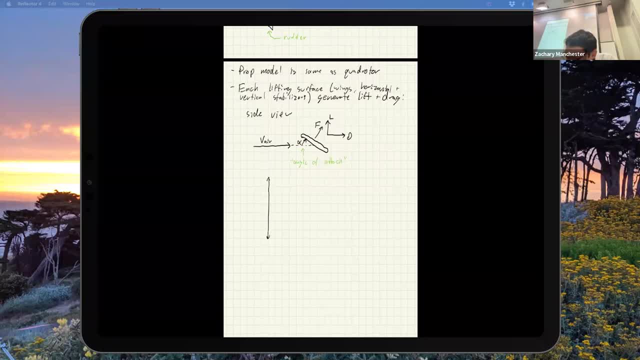 I talked too much today So we're sort of running out of time. See how far we get. We might have to do this next time a little bit, OK. So here's L versus alpha, And so roughly it's linear-ish in some region near 0.. 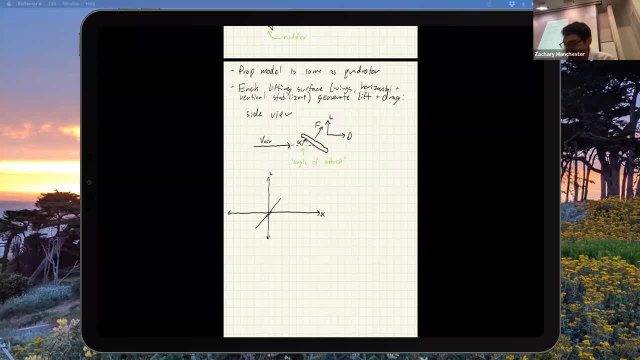 And so we pretty much always approximate this as linear as all things. And then it starts to do this: Once you get to a certain point it starts to taper off. So it does something like this: It roughly looks like a sigmoid. 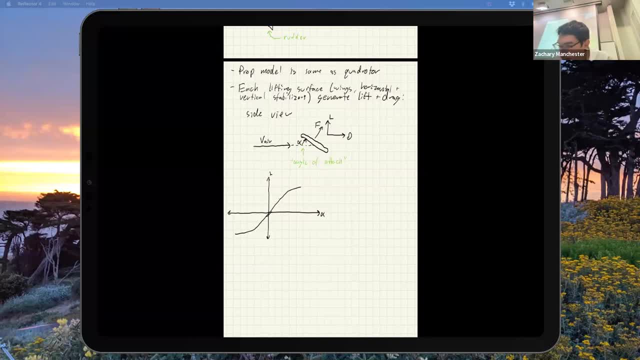 And then it sort of tails back down. It sort of does this- And this is a bad drawing, as usual for me, So something like this sort of sigmoidy- and then sort of yeah, And so this linear regime say here-ish right. 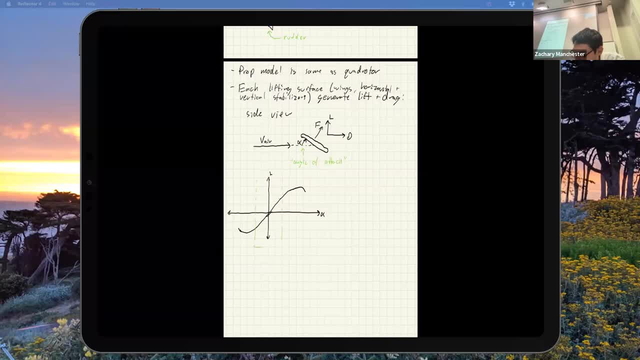 This is typically where we like our airplanes to live. We don't like going outside of this linear regime, And usually this is for most airfoils. this is sort of like plus minus 10 degrees, OK. So question is, what do I call the peak over here? 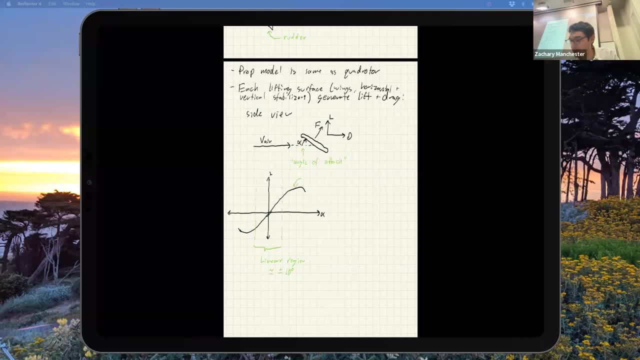 where this thing sort of rounds off and starts to go down, And this is a bad drawing. Maybe I'll fix this up slightly. I don't know what that's called. That's stall, Yeah, So when you talk about stall on an airplane. 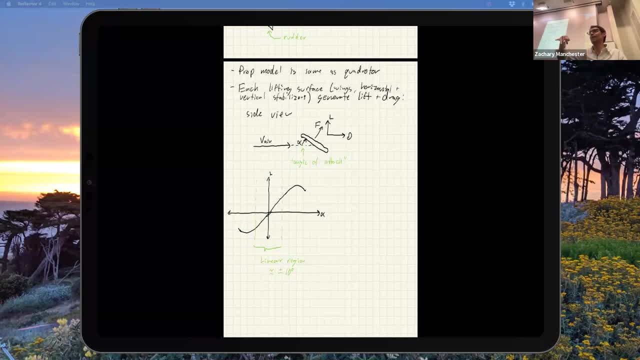 it's the peak of the lift curve where the lift starts to decrease now. So if I'm doing this, I'm getting more and more lift. At a certain point, the lift actually goes the other way And I start to do you know yeah. 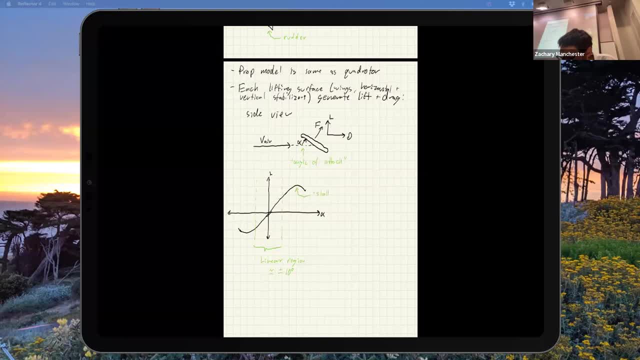 So this peak here is stall And we don't like to go there. Going there is bad. This is where It's in practice. this is due to flow separations. Basically, the airflow is starting to separate off the trailing edge of the wing. 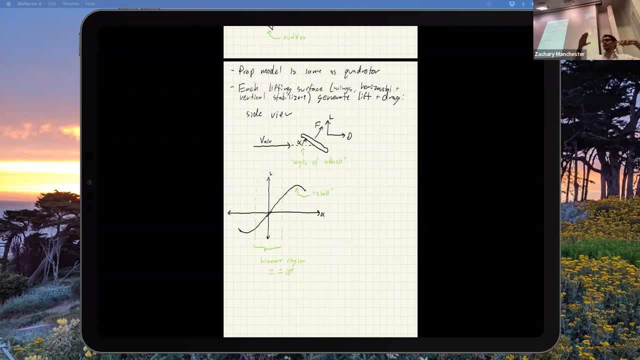 You get detached flow And you get turbulence coming off the back of the wing And you feel this in the airplane as buffeting. You start to shake And it's bad. You don't like this, OK, And then drag. So same thing, alpha. 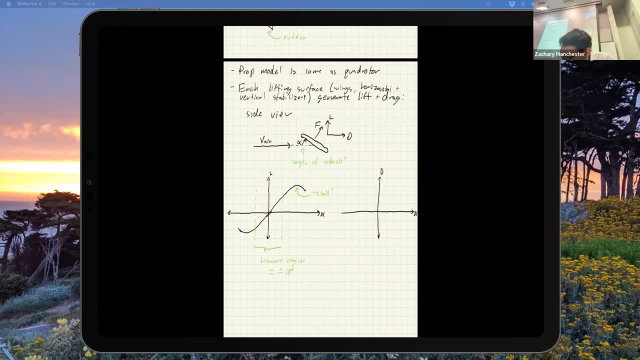 And then d here Drag is roughly quadratic For small planes, For small angles, And you've got a certain amount at zero angle of attack that's due to skin drag, just whatever friction. And then as you increase the angle of attack, roughly. 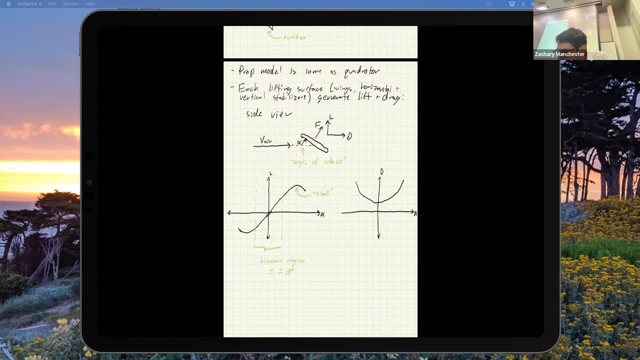 speaking, it increases quadratically. And let's see, Yeah, Is everyone good for two or three more minutes? We're almost done with this whole thing, So I don't want to keep you guys. We've got to go, But yeah. 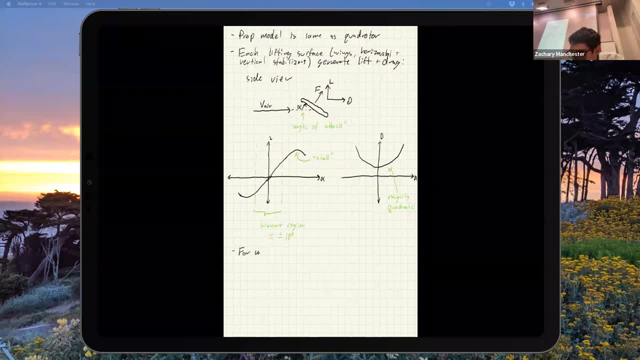 So, generally speaking, what you do is for most applications- meaning like if you're designing a controller and you don't want to do insane aerobatics, you use linear and or quadratic approximations of these, So like if you're going to have an foules. 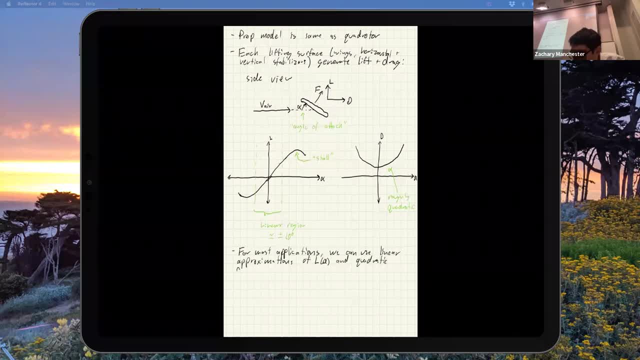 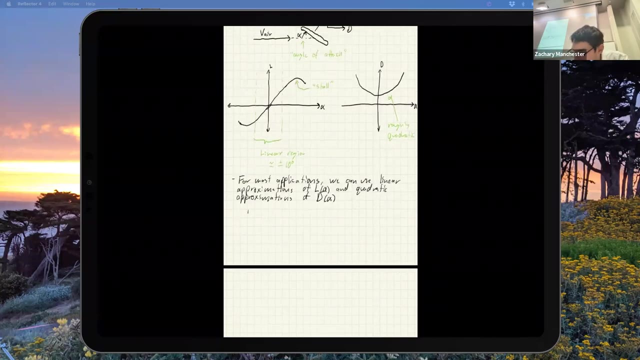 And you are going to rank them. try. you'll find that they're O Fortune 1 charts and you can't even open them that much And you can't even refer to them on the Lathe 곰 meas. and you must also understand that you can't darn them. 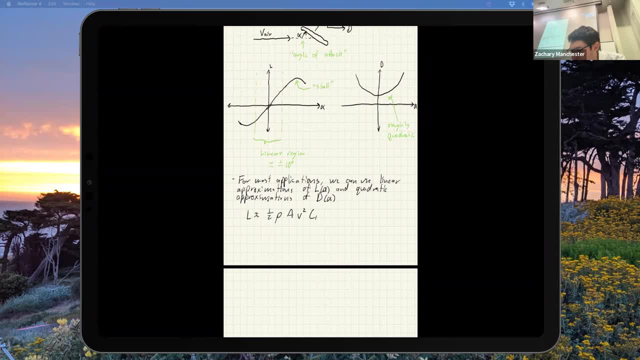 Yeah, Okay. so this is lift, This is the density of the air, This is the area, the wing area, This is velocity squared- This guy over here- CL0, this is called the lift coefficient And this is actually the slope of this lift curve at the origin right. 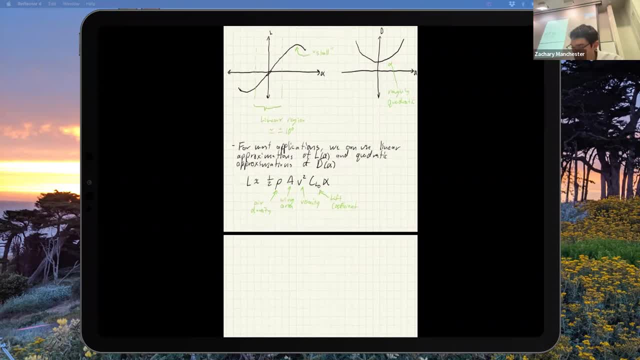 And then this is the angle of attack which we already know. And then the other one we get is drag. So this has the same form- rho, AV squared- And then it's going to look like this: It's going to look like CD0, which is the height of that lift curve at the origin right. 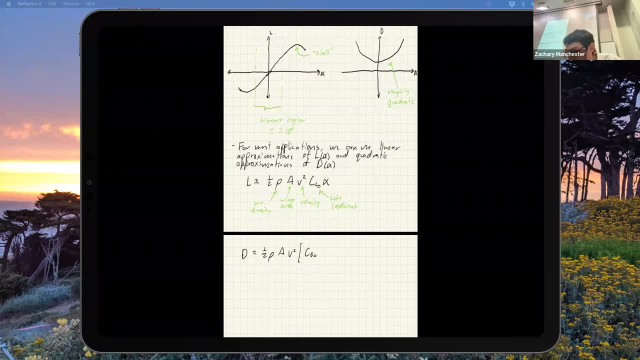 So that's a constant term, And then maybe, if you- a lot of people leave this out right, So if you're linearizing, this goes away, but then maybe you'll get what would be called like CD2 alpha squared, And then this guy is called the drag coefficient. 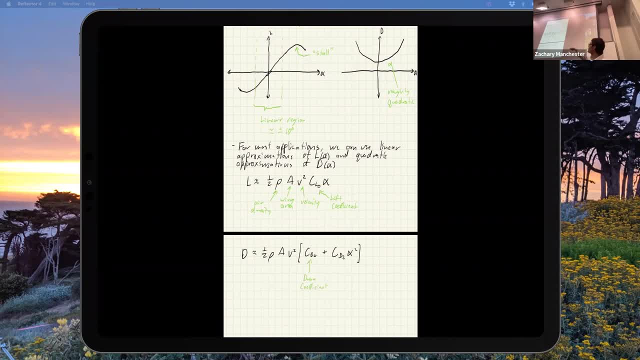 So you hear about drag coefficient for all kinds of things, cars, et cetera- right, That's what that is. It's the constant term from the second order, Taylor expansion of the drag curve as a function of alpha, It's like how far off the. it's the amount of drag you get at zero angle of attack, right? 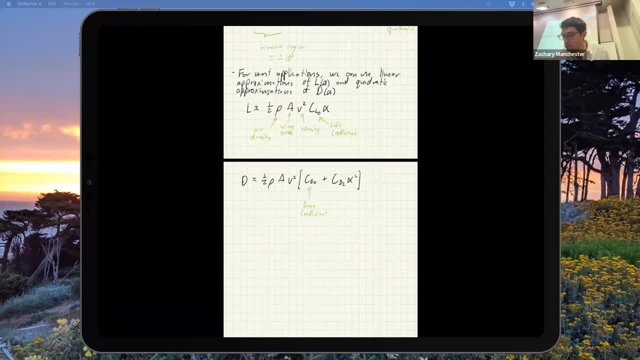 Okay, What else is there to say about this? So the way you model- so we talked about control surfaces, ailerons, elevators, rudders- The way you model those- the generic name for those is a flap. They're all called flaps. 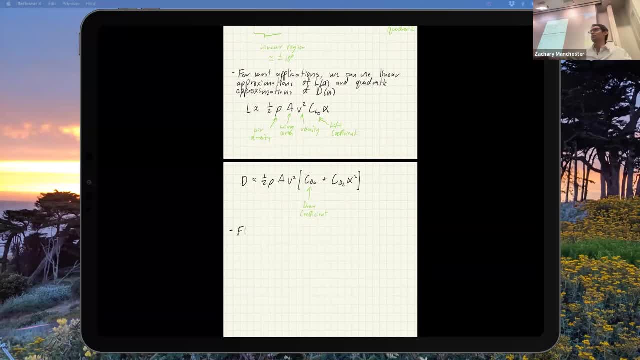 And what they do is just change the effective angle of attack when you change those control surfaces. So let's model that. So you got alpha. effective equals alpha, plus this epsilon I times UI. So this would be your control input. So this would be like your flap angle. 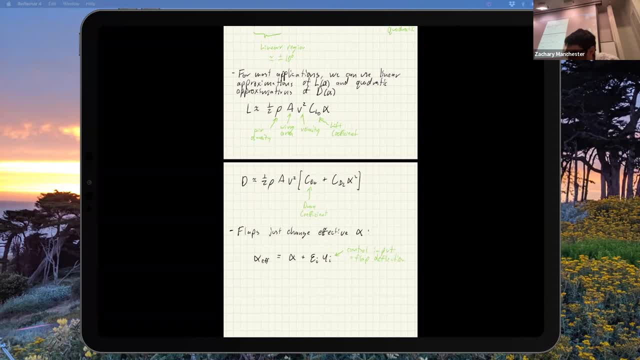 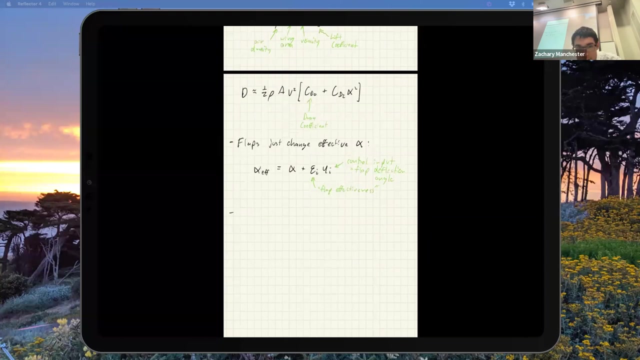 This is your flap deflection angle, for you know, elevator, whatever, rudder, this guy is called your flap effectiveness And again, this is like wind tunnel, model, whatever, and that's it. And then you plug everything in and you get your forces and torques and you get your stat. 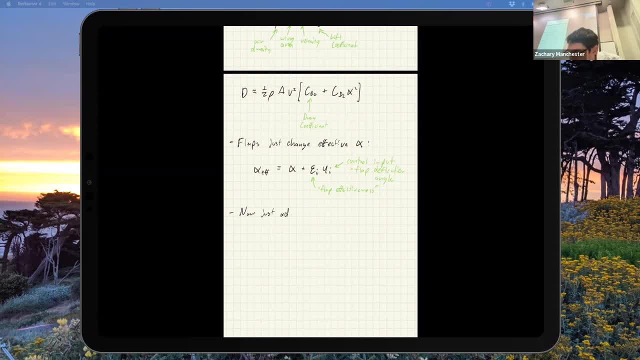 everything up, Okay, Okay, We're not going to do this by hand because it's complicated As you imagine. there's like center of lift for every single one of these and an offset vector and lots of cross-product things and whatever This model is, this is literally how you simulate like a commercial airline. 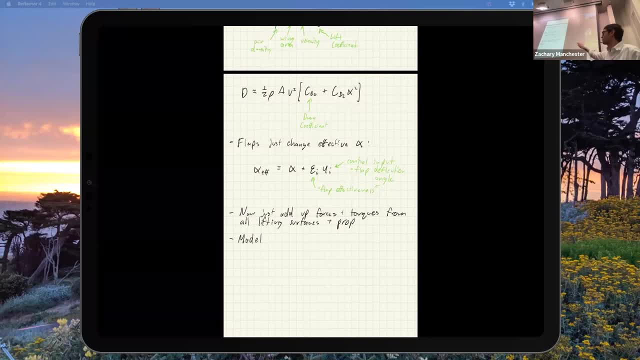 This is like the standard thing. This breaks when you start to do crazy aerobatics, Basically high angle of attack- right, It's what we assumed- plus minus 10 degree-ish angle of attack. When you start to do crazy post-stall stuff, this starts to break. 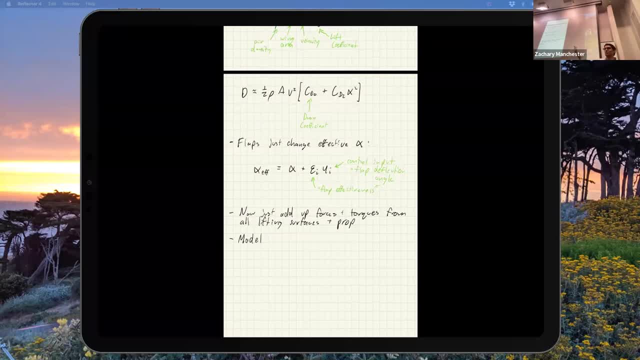 So aerobatics- really aggressive aerobatics or perching, is like another one where you try to like like a bird perching. People have done this in robotics. It's kind of fun. It's actually a really fun robotics problem.